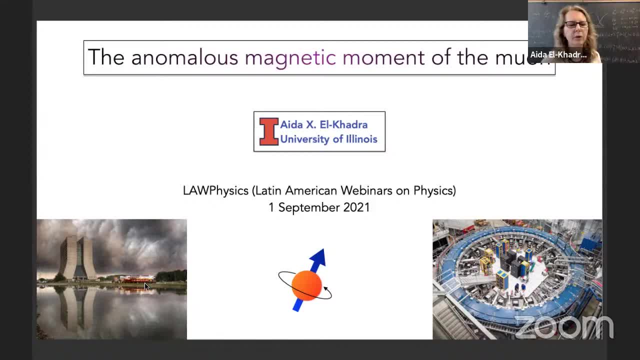 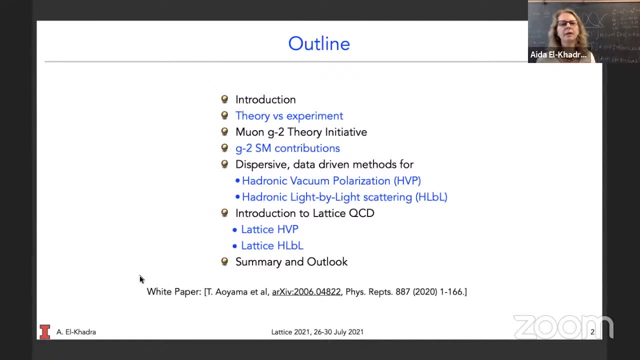 and here you see a picture of when the muon magnet ring arrived at Fermilab to begin taking data. So here is an outline of my talk. I will start with an introduction, tell you a little bit about the overall global situation and then tell you a little bit more. 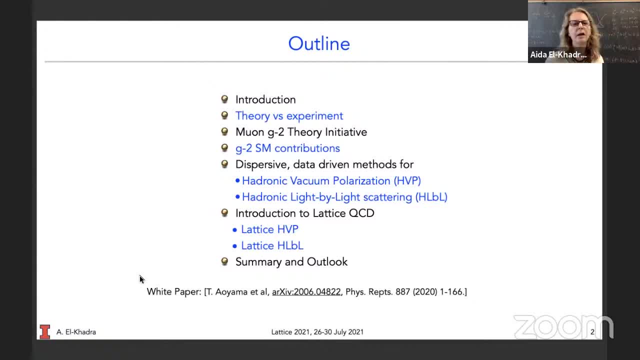 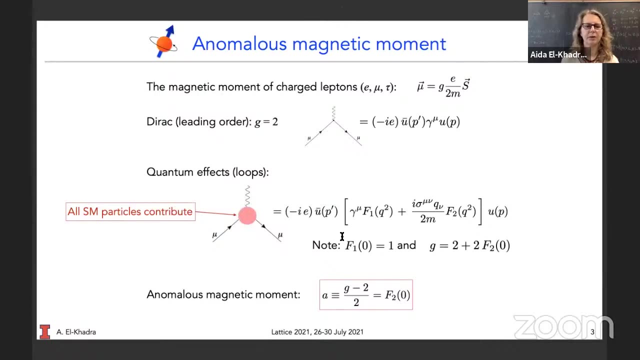 the theory initiative and the standard model contributions, before delving into more detail into the hadronic contributions with the two methods, and then conclude with a summary and an outlook. So first just to get started, to put us all on the same page, as a reminder. 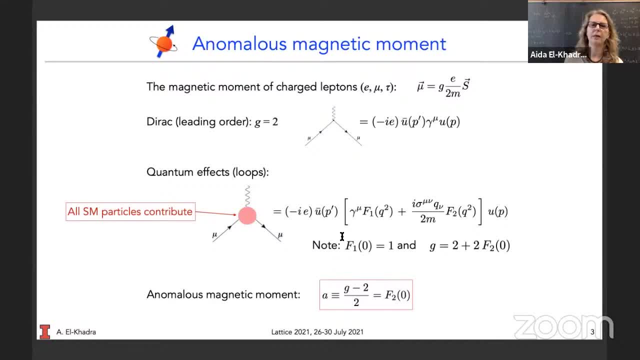 we're talking about the magnetic moment of an elementary particle that also carries electric charge. So the muon is just one of three charged leptons, the electron and the tau, lepton being its siblings, being distinguished by their masses. So the combination of electric charge and spin. 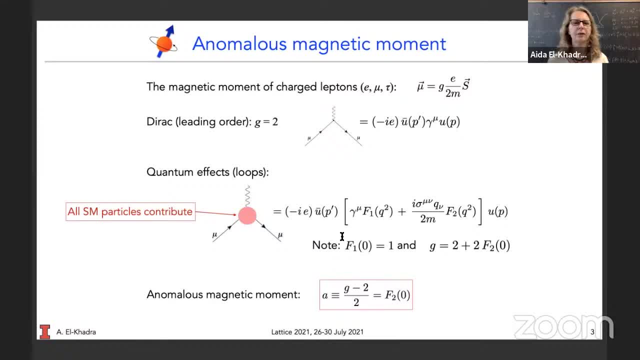 gives rise to magnetic moment which, in the Dirac theory, was predicted to be to have a pre-factor. a g-factor equals to two. Once one includes a quantum correction loop effects, then the vertex is modified to this form where, via acquiring F2 of zero, acquiring from 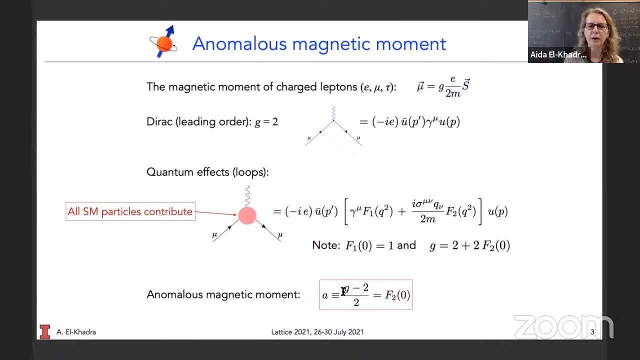 quantum loop effects and non-zero value now leads to deviation of g from two, which is parametrized as the anomalous magnetic moment. A is defined as g minus two over two is exactly equal to F2 of zero. So F2 of zero can be computed in the standard model by computing all possible loop contributions. 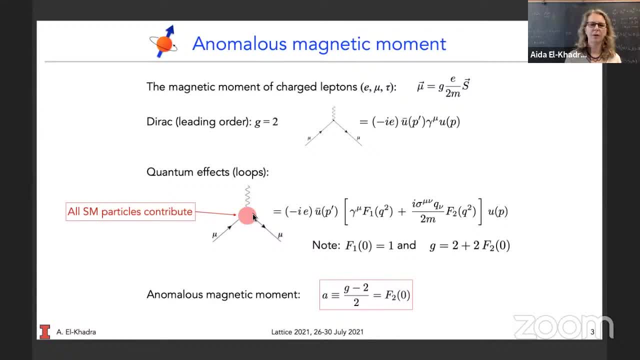 to this vertex from all standard model particles. As such, of course, this quantity is very interesting. The anomalous magnetic moment, as you see, by definition arises due to loop effects, So anything that is only sensitive to loop effects in the standard model by definition. 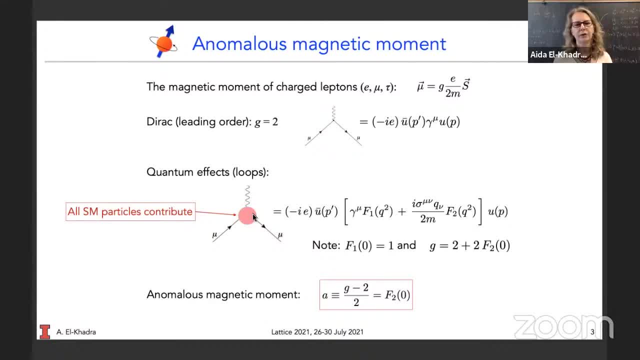 would also be a loop effect. So of course this quantity is very interesting. The anomalous magnetic also be sensitive to the effects of new particles not yet observed. And in particular, if you look at the structure of this vertex here, you will see that muon in, muon out. This means of course, 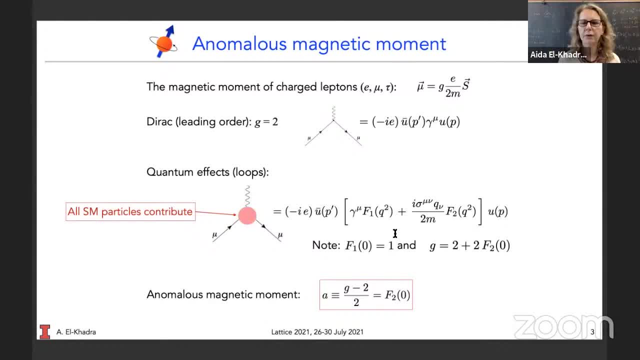 this contribution is flavor conserving, It is also CP conserving and it flips chirality. So in terms of probing new physics effects, this one is complementary to some other effects, say CP violating effects, et cetera, or flavor violating effects. So it is also from that point. 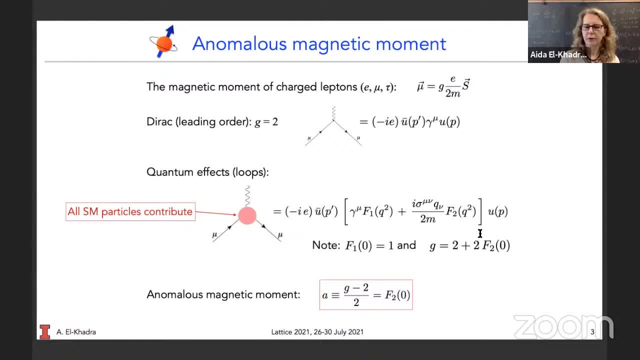 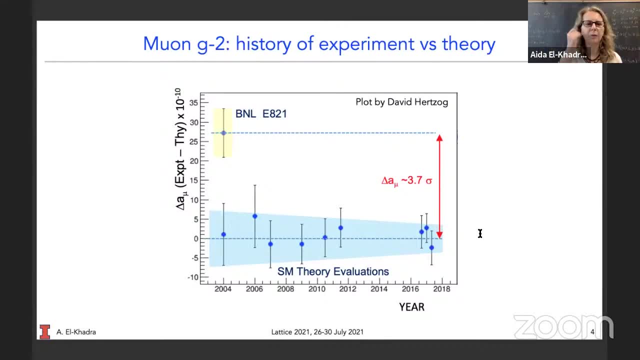 of view, an interesting complementary probe. So let me now go to a little bit to the history. So one of the reasons why the muon magnetic moment is so interesting and receives so much attention is because there's a long history of the muon magnetic moment. So the muon magnetic 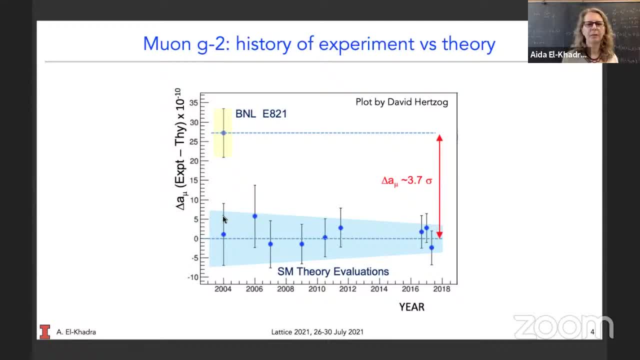 moment is a long-standing difference between standard model expectations shown here and prior to the Fermilab experiment coming out with their new measurement. The most precise measurement came from a Brookhaven experiment that concluded 20 years ago and left us with a tantalizing but. 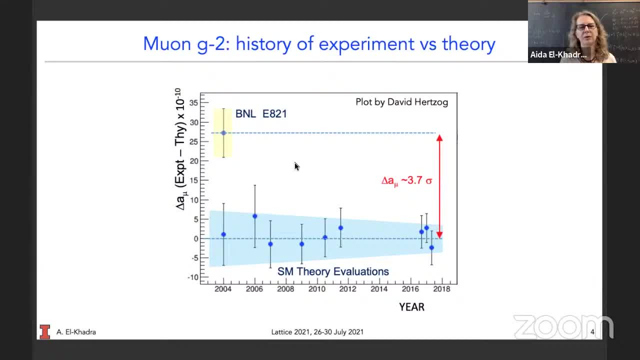 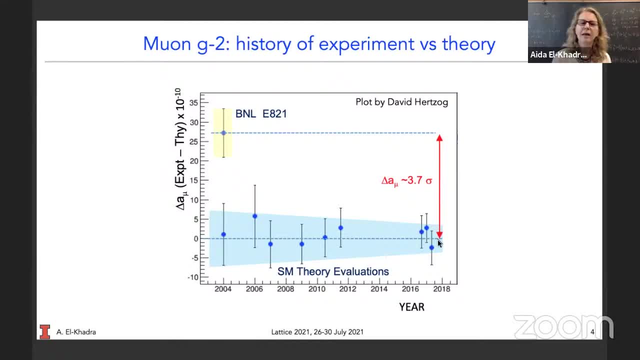 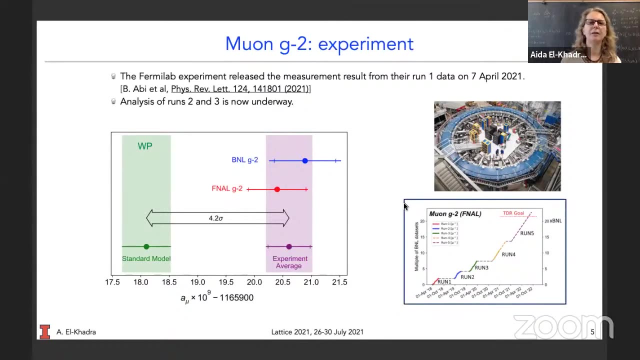 precise, in the intervening 20 years It hasn't moved, which is also significant, And now we have a new experimental measurement by the Fermilab experiment. What the Fermilab experiment did is they took the ring that was situated at Brookhaven and moved it to Fermilab. 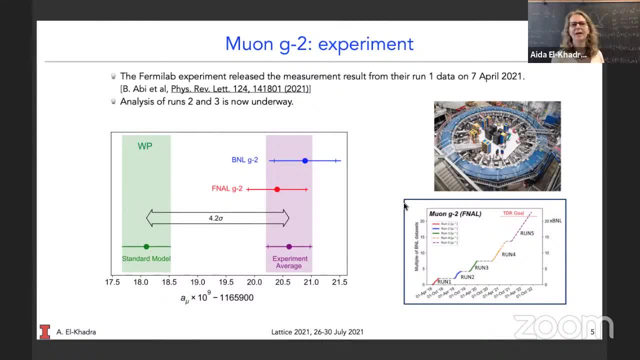 they recalibrated it and redid everything you know, made this in a much better instrument than it was at Brookhaven. It is fed by a higher energy and higher intensity muon beam, So this is really a brand new experiment, using the same experimental methods as the Brookhaven experiment. 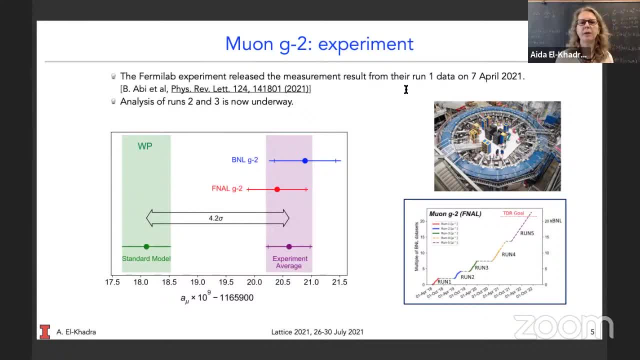 And they released the measurement result from their run one data on the April, the 7th of this year to great international media attention, And I will tell you in a second why. Also significant is that they already have the data from their runs two and three in the can, so to speak, and that analysis is ongoing. 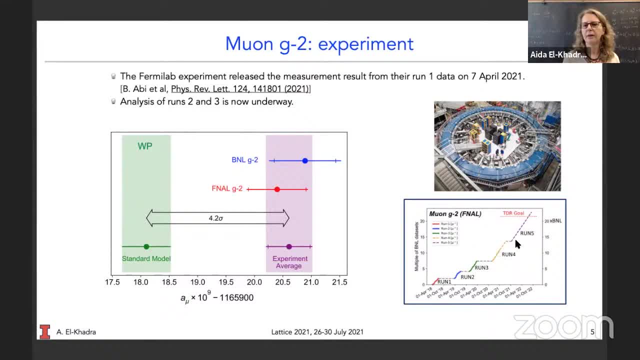 And they're currently running also. they're currently they started run five or are about to start run five soon, So a lot more data will come from the Fermilab experiment. Now, what happened and what was so super exciting when, on April, the 7th, 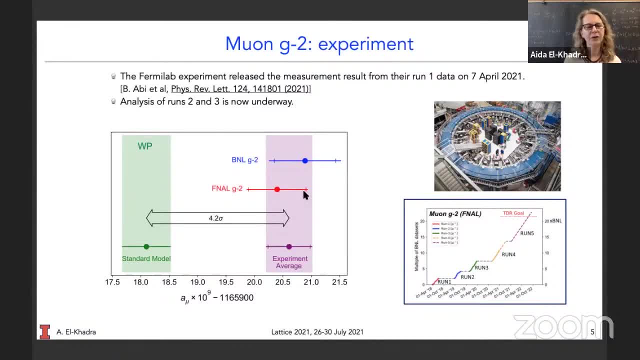 when the Fermilab experiment revealed their new measurement. first, their measurement is in complete agreement with the Brookhaven measurement, So that by itself is, you know, just an amazing success of a really beautiful experiment, And I think that's a really good thing, And I think that's. 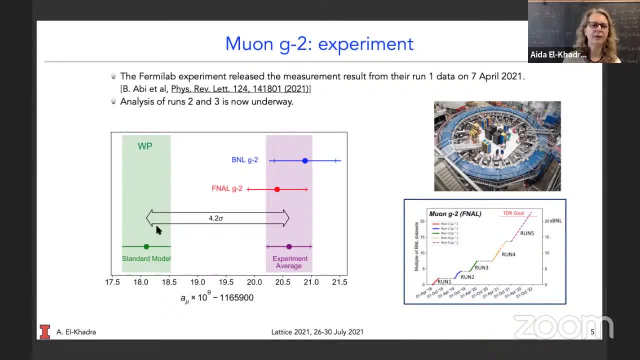 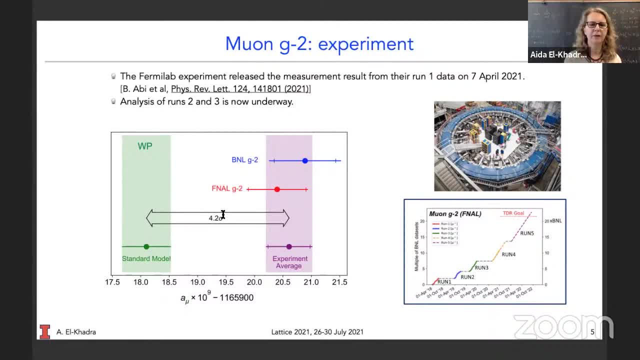 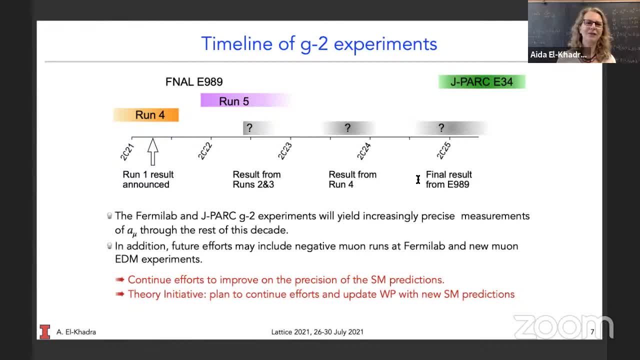 within the next five years are very, very good indeed. The prospects that we will have a total error on the experimental measurement reduced by a factor of four within five years from now is really good. So that means that theory needs to keep pace, And that was one of the aims. 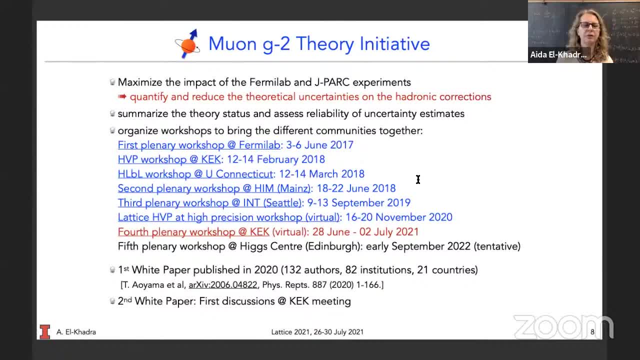 of the muon g minus two theory initiative is to address the experimental progress and bring the entire theory community, I should say theory and experimental community, together to have a comprehensive assessment of the various theory uncertainties that go in and make the theory predictions, the standard model theory predictions, more reliable. 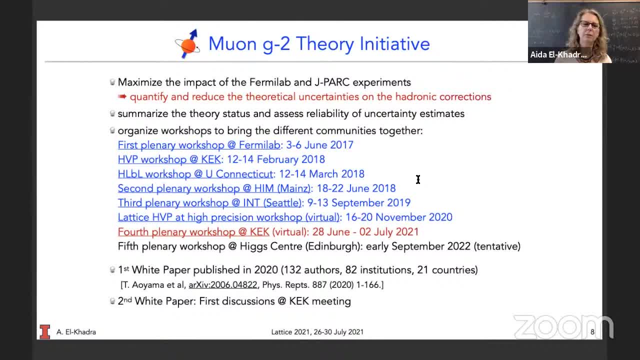 and also more precise. So by putting all of the disparate communities together, we learn more. So for that purpose, the theory initiative got going in 2017, we've already had over a half a dozen workshops. The last one was a virtual workshop that was held at KEK. 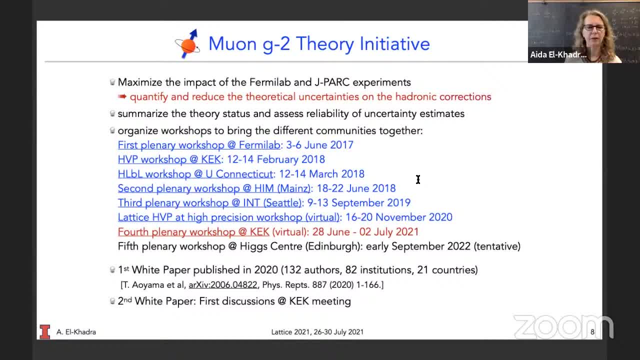 And we're planning another workshop next year because we're planning to update our white paper. The first white paper of this initiative came out in June of last year and is the basis upon which the experiments in research and development and the research efforts are being conducted. 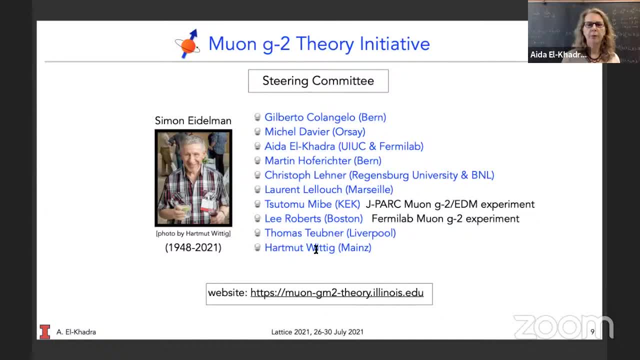 So that's a short summary of the background, and I'd like to share with you a bit of a summary of the research from the conference, the research and development team and then a few of the participants that are coming up. So, first of all, 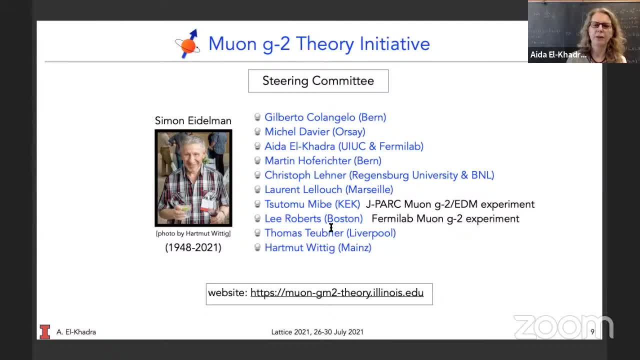 I would like to talk about the research that we're going to be doing in the next two weeks. So I'm going to start with a brief overview of the research that we're going to be doing in the next two weeks, after the conference, And then I'll share with you a little bit. 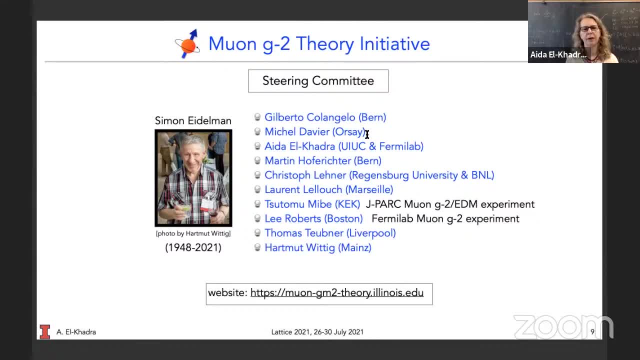 from dispersive theorists and from experimentalists that provide the experimental inputs. I should mention that the community, and in fact the community of people working in low energy experiments and hadron physics suffered a great loss earlier this year with Simon Eidelman, who was a member. 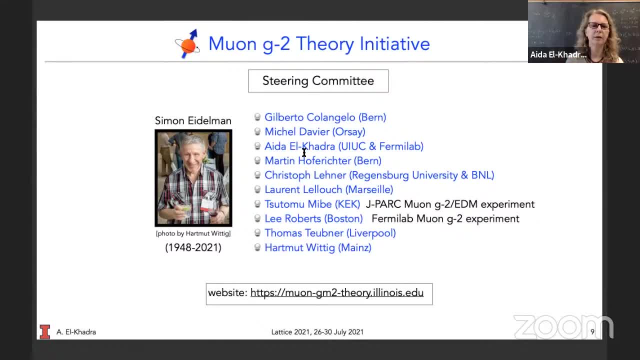 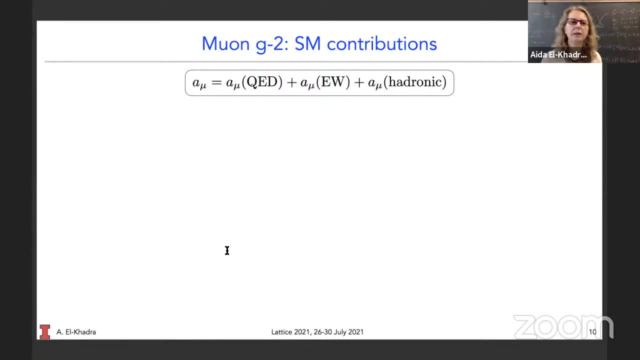 of the steering committee and involved in many experiments- relevant experiments- passing away rather suddenly And he is going to be very, very hard to replace. So let me now go to telling you about the ingredients of the standard model. prediction of the anomalous magnetic moment. 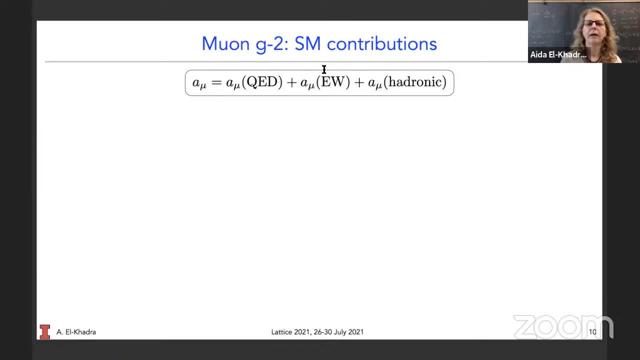 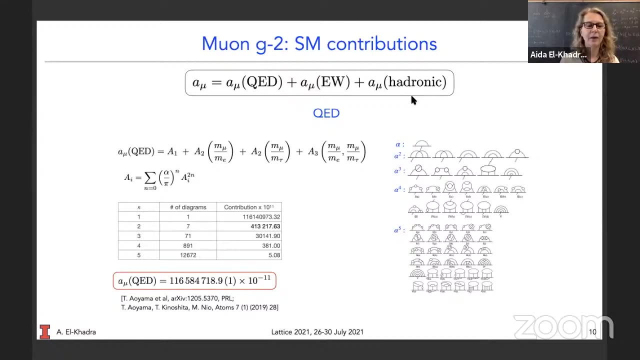 It is usually broken down into QED and then electroweak, being focused on the weak bosons and Higgs boson, et cetera contributions, and then the hadronic contributions, Starting with QED. this is a story that spans several decades as well. 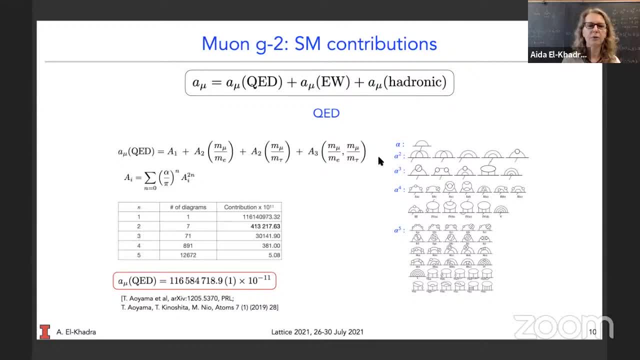 of an amazing, heroic effort to compute the QED contributions through fifth loop order, which involves tens of thousands, over 10,000 diagrams and results in the QED contributions to the anomalous magnetic moment of the muon now being known to a precision that will never be reached. 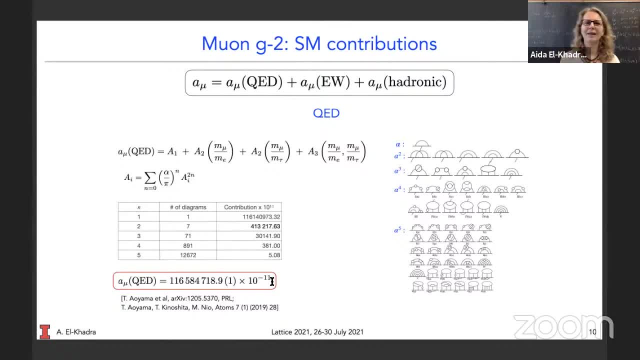 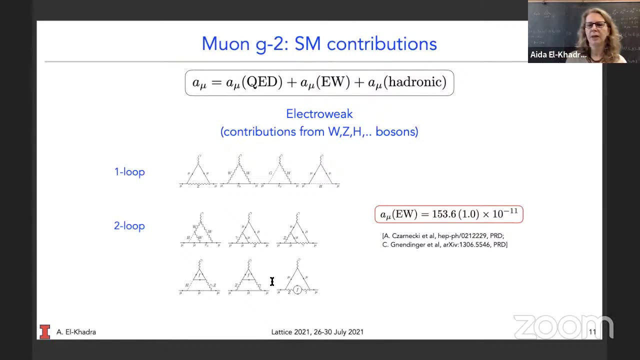 or will not be reached in a very, very, very long time by the experiments. So it is basically done and known now, thanks to the efforts of a very dedicated community of people. Similarly, for the electroweak contributions, there were dedicated efforts to compute these also. 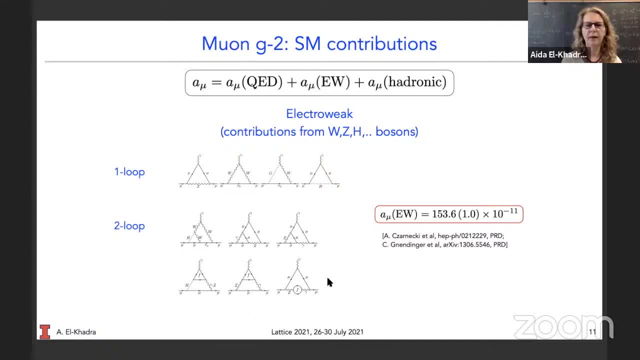 with the measurement of the Higgs boson mass. The last contributions could be computed even more precisely, And this is now known, through two loop order, with the remaining uncertainties small, the remaining uncertainties actually being dominated by hadronic loops in the two loop contributions. 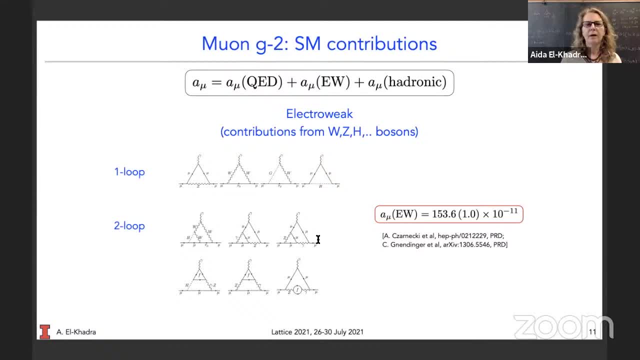 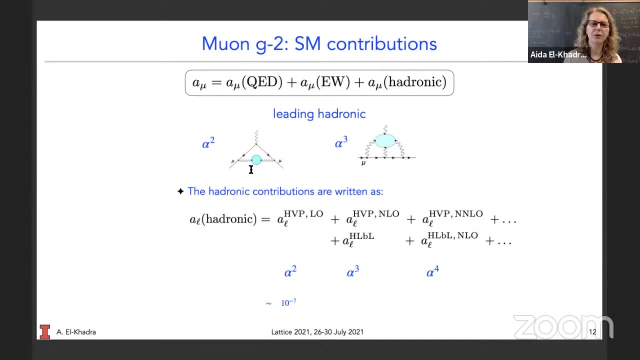 but here they don't play a large uncertainty role. The hadronic contributions are the topic of most of the discussions of the theory initiative because they drive the theoretical uncertainty. The first, the leading hadronic contribution comes from the so-called hadronic vacuum polarization. 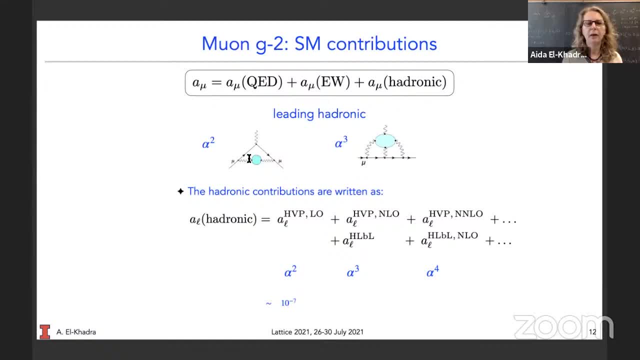 whereby a muon emits a virtual photon which creates a hadronic vacuum bubble and then recombines. So that's the regular vacuum polarization, of course as well, but now with a QQ bar loop that creates a hadronic bubble, A contribution that's suppressed by another power of alpha. 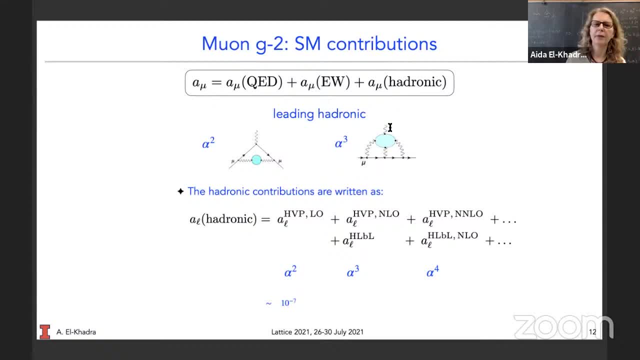 so it's of order. alpha cubed is the hadronic light by light. You can see four photons here. that looks like light by light, scattering, then connecting to the muon line. That's why this is called the hadronic light by light. 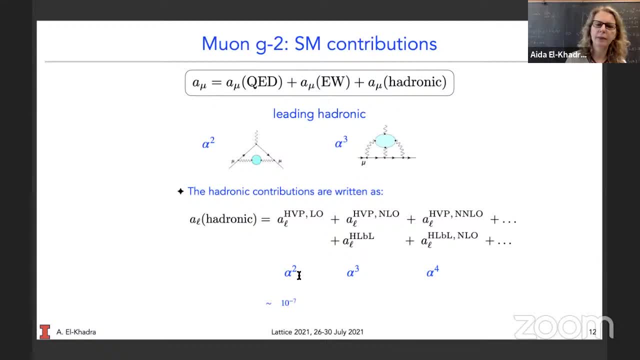 So hadronic vacuum polarization enters at order alpha squared. And then, in order to meet the precision demands of the experiments, we need to also compute the next to leading and next to next to leading order contributions, meaning hadronic contributions that entered order alpha cubed. 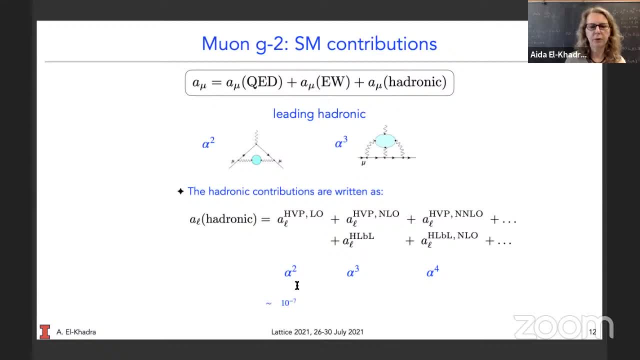 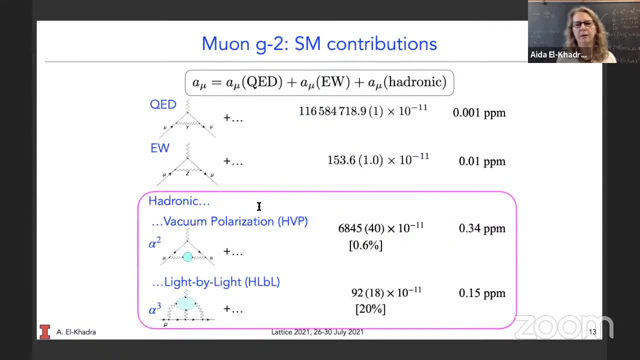 and at order alpha to the fourth. So the contributions are smaller, much smaller than the QED contributions, but they are the dominant. they make the dominant contribution to the theory error. So this is summarized here, where you see the QED contribution. 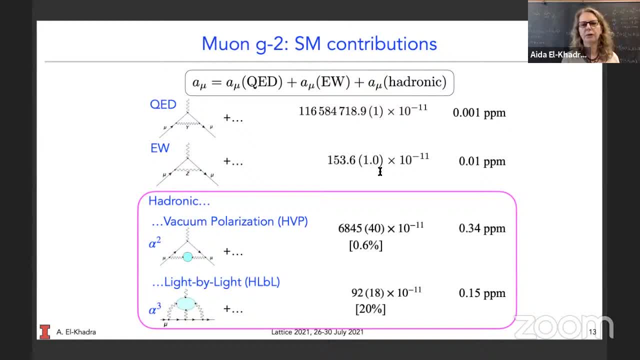 the electroweak contribution also very small. It's 150 in units of 10 to the minus 11, with the theory errors that are basically negligible. recall that the precision target is 140, of the experiment is 140 parts per billion. 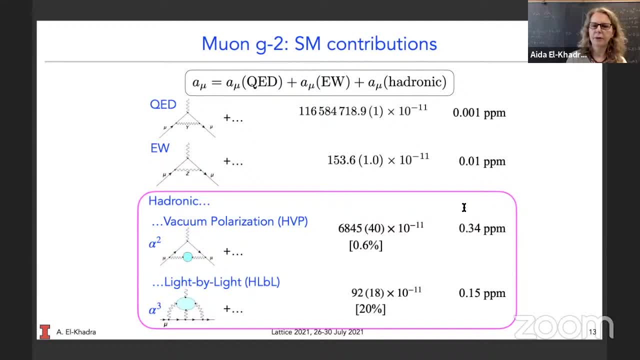 So these are basically irrelevant, these uncertainties, but these uncertainties are very much relevant And that's what I will be discussing Now. note that this is the driving uncertainty, but the hadronic vacuum polarization itself is known to sub-percent precision In order to make this uncertainty small enough. 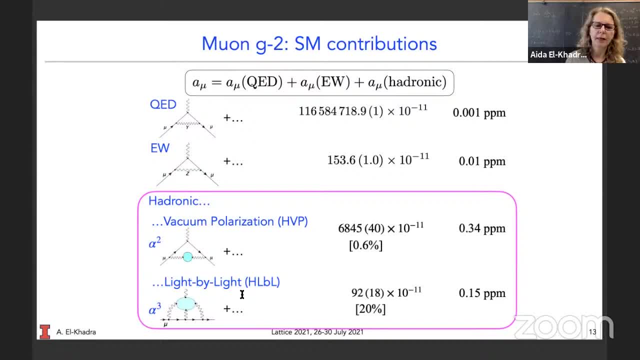 it needs to be known to about 0.2% The hadronic light. by light being suppressed, you can see its overall size even further. actually, to address the precision targets, we only need to know it to about 10 to 20%. 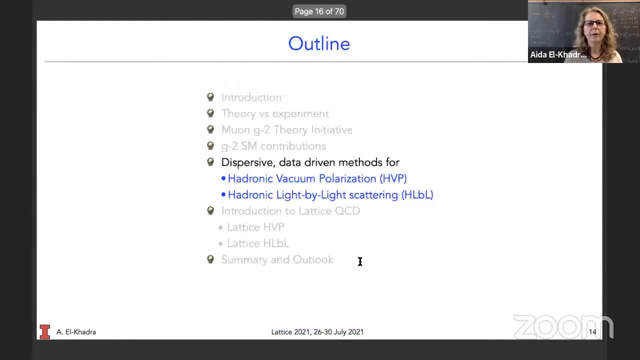 in order to meet the precision demands. Okay, so this is a briefish introduction, So let me now delve a little bit more into it, A little bit deeper, into the hadronic contributions, First describing you how these are evaluated using dispersive data-driven methods. 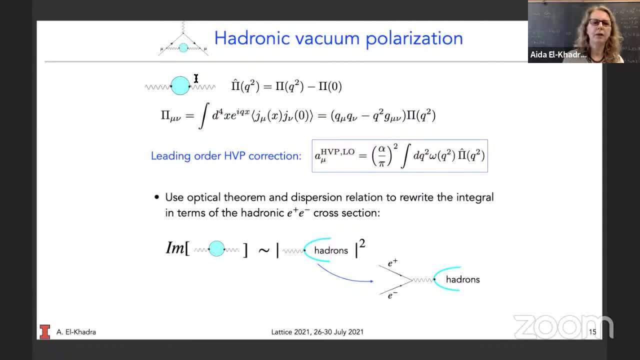 So, just again as a reminder, we're talking about the hadronic vacuum polarization function defined here, which is then plugged into the loop integral to be evaluated, and the schematic form is given here. Okay, So with knowledge of the vacuum polarization function, 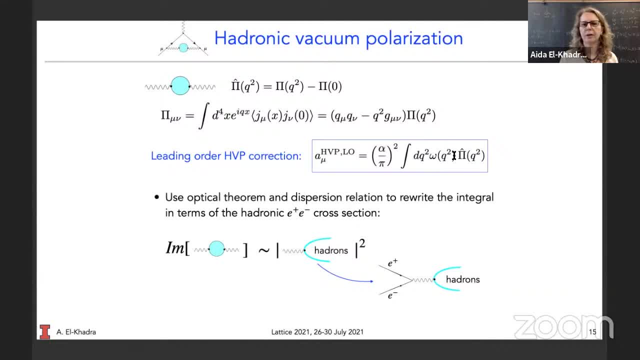 and this is just the. this is just. this comes from the loop integral and contains kinematic factors, et cetera. one then can compute the hadronic vacuum polarization loop contribution to the anomalous magnetic moment. In the absence of being able to compute, 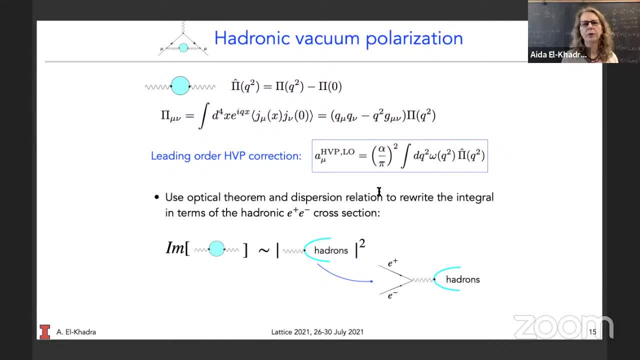 the vacuum polarization function over all Q squared ranges. we need to know this not just at large Q squared, where we can use perturbative QCD, but also at low Q squared, where the vacuum polarization contribution is dominated by hadronic contributions. 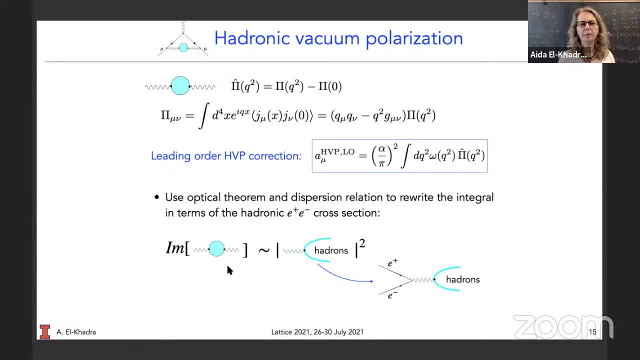 And that is of course the difficulty. So one uses the optical theorem and then a dispersion relation to rewrite the integral in terms of hadronic cross-section, which gives you this expression, with a new integration kernel shown here. Again, these are all known equations. 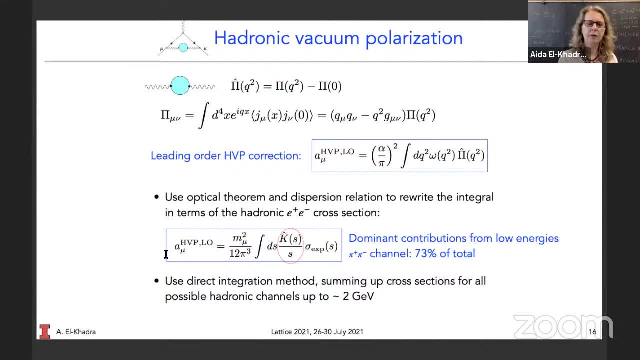 I'm not going to write them down Now we have expressed the hadronic vacuum polarization, at least at leading order in terms of experimentally measurable cross sections And if all of the cross sections that contribute at all of the different center of mass energies are known. 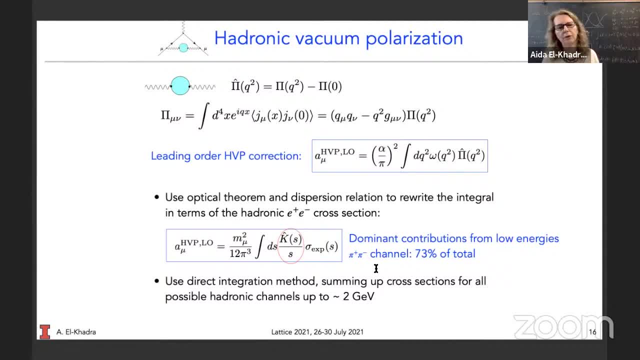 then all one needs to do, basically, is sum up over all of the channels to obtain this. So this then leaves the determination of the hadronic vacuum polarization contribution. that is driven by the experimental measurement errors. So this method has been developed and refined over the past 20 years. 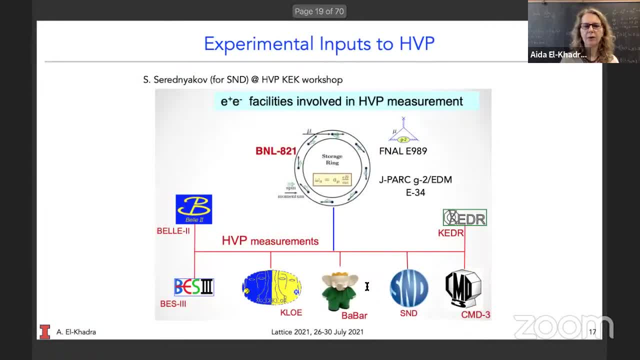 and the experimental cross-section measurements have also been performed over that long, So there's a whole community of experiments that provide these measurements. some of them are still active, even though the experiments themselves have long stopped collecting data, for example, like the Babar experiment, and some have just started collecting data. 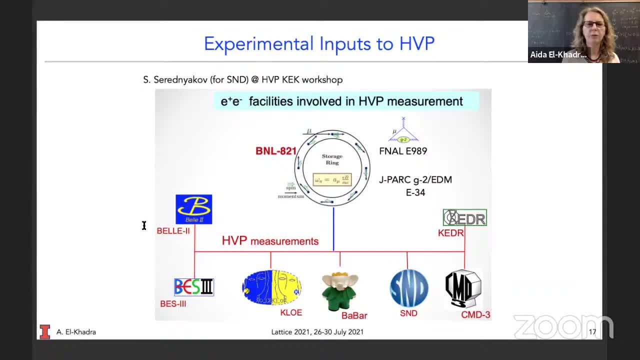 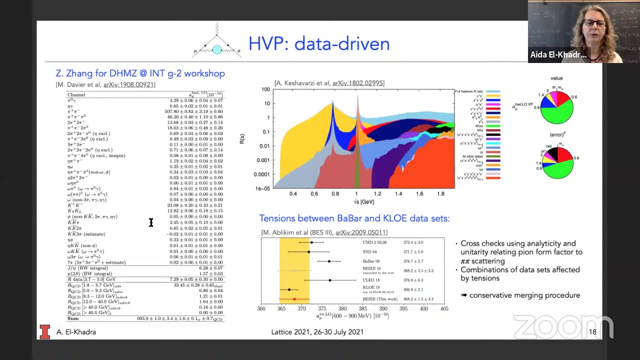 So this is a good situation because these measurements are needed with exquisite experimental measurement precision, and having many different experimental measurements that can then also be compared to each other is good, so that we are really ensuring ourselves against measurement errors in this important quantity. So here's a summary of two of the leading compilations that do these evaluations. 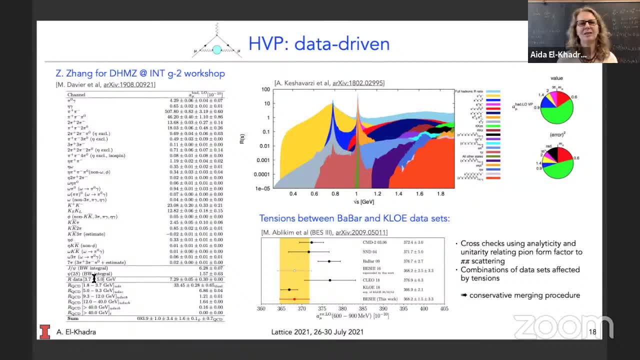 You know I'm not meant to read all of the channels, This is basically just an impressionistic view to tell you that basically all of the channels up to about 2 GeV, all of the different hydronic channels, have been measured. 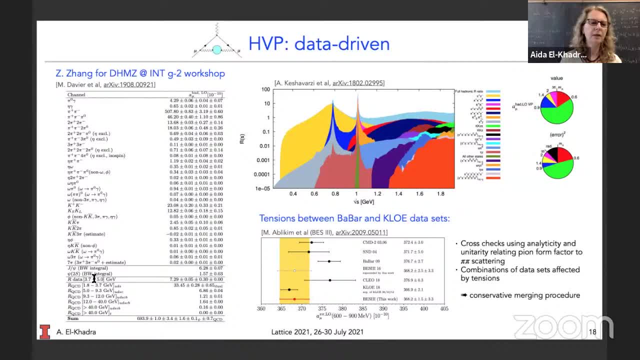 And some of these measurements are very, are rather recent- some of those high pion, multiplicity and other channels, but they're all now measured and can be summed up in the direct integration method. So this is- this is also illustrated here. So this is from the DHMZ compilation and this is from the K&T compilation, with a very colorful mountainous plot indicating all of the different channels and their contributions in this region. 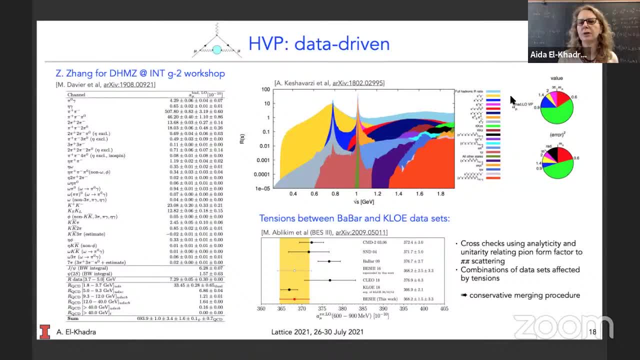 And over here in the pie chart. it shows the contributions from these different channels to the value of AMU and the contributions from the errors. What you can see is that it is the this region here, the region below a GeV or so, that gives the dominant contributions to the theory error. 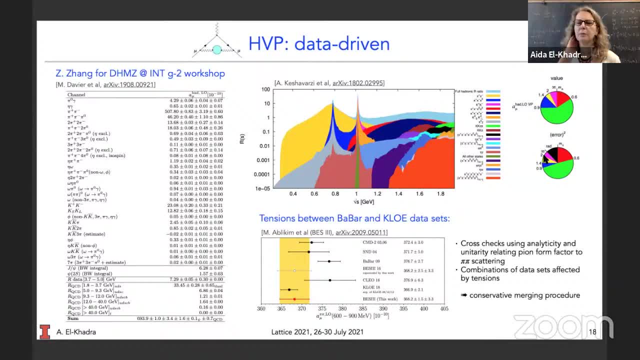 There's also contributions due to radiative corrections and perturbative QCD, but those are really really small, comparably small. So the experimental errors in this energy region are very important and measuring the channels in this energy region, which is dominated by the pi-pi channel. 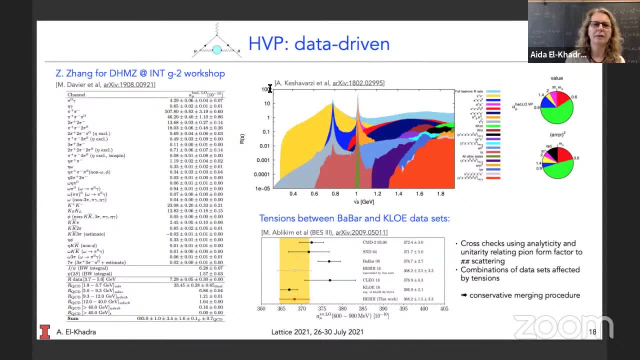 that's the yellow shown here. Note that this is is a log plot, so in a regular plot, this yellow would be huge, This yellow contribution would be huge. it dwarfs the other ones mostly. Okay, so what? what is, however, also going on is in that important yellow region, the, there are some tensions between the two different data sets that have the smallest. 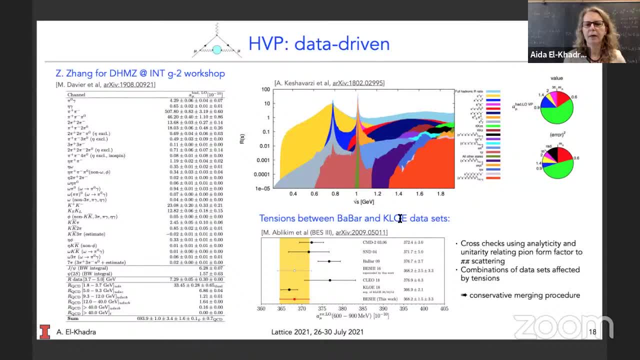 overall uncertainties from Babar and Chloé and that tension needs to be taken into account. obviously, if we take the, if we want to take these compilations to obtain AMU. This was subject of intense discussions at our workshops: how to do this safely, how to understand the tensions and then how to deal with them. 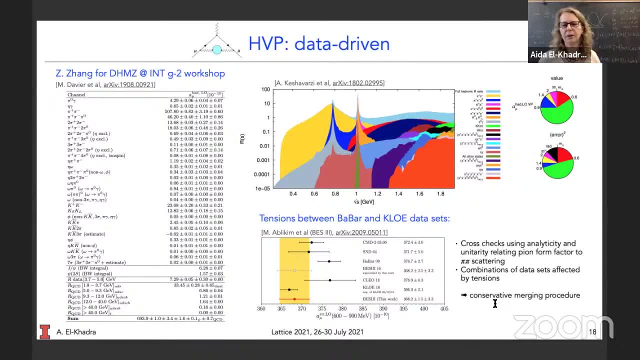 So the outcome of that at the INT workshop was in 2019- was a conservative what we called merging procedure, in order to account for all of the tensions in the data and also for slight differences that are that occur when different groups of people make slightly different choices. for when do you connect to perturbed? 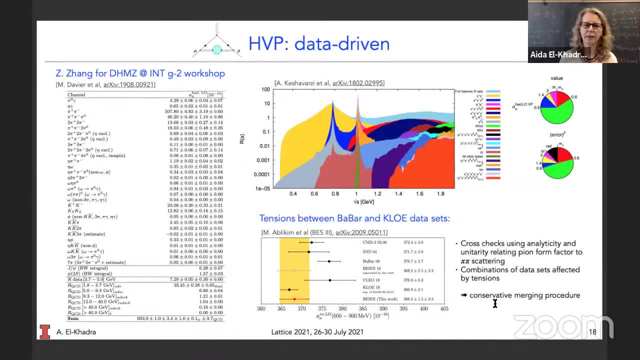 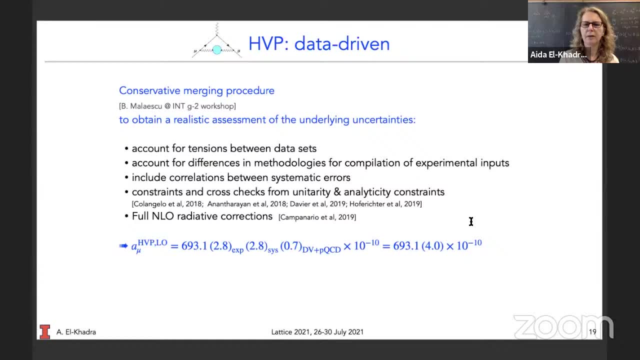 of QCD, how do you treat the systematic errors exactly, et cetera. So the ultimate result is then this: this: this is the result that came out of this theory initiative effort, And you might note that the total error is not smaller than individual errors from individual compilations. 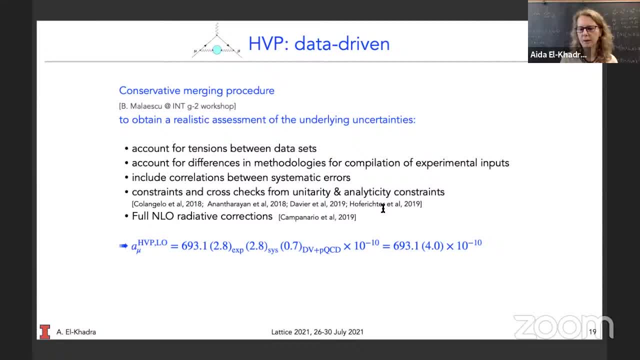 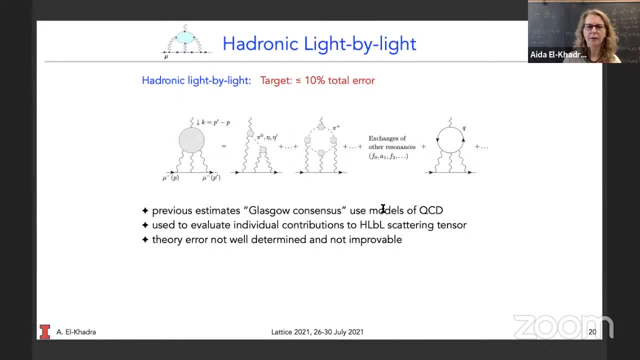 because we were conservative in how we treated the total errors. Now let me talk a little bit more about. well, let me start talking about the light by light contribution, which is illustrated here. Prior to the theory initiatives efforts, the light by light contribution was estimated using, essentially, models of QCD using large N. 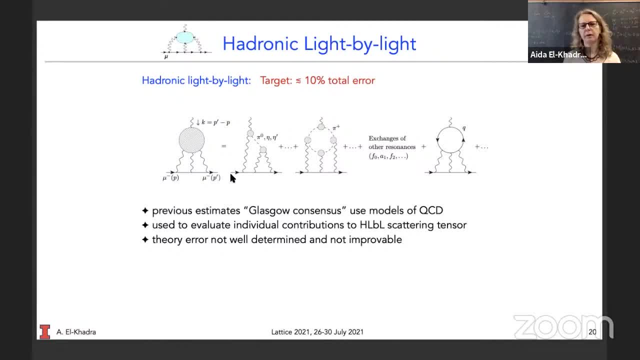 um estimates and uh chiral perturbation theory inspired models where uh, where one then uh obtains uh estimates of individual contributions into which this hydronic bubble can be broken up to uh. the dominant contribution comes from pion exchange. 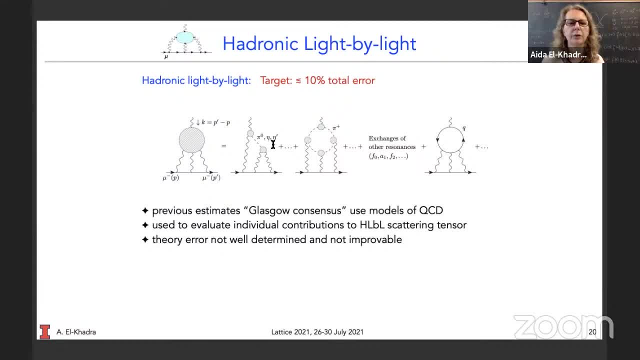 but they will also be um higher pseudo scalars and there's loops and other resonances contributing. The problem is that different models will break these contributions down differently And this was tried to be estimated using- uh, just averaging over all of the different models and the Glasgow. 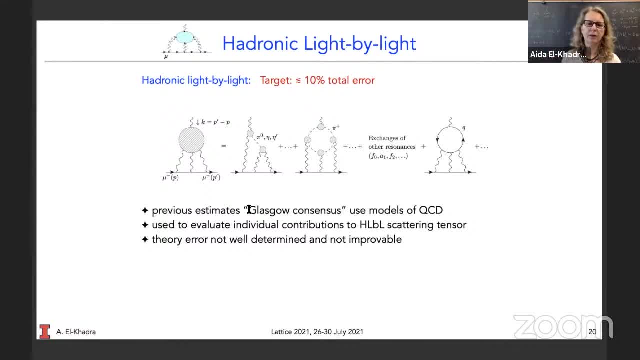 consensus. This means that, um, the theory error for this quantity prior to the theory initiative was really not well quantified at all And people were worried about: uh, what if these models are simply wrong? What if the estimate of the light by light is off by a factor of two? then it could be. 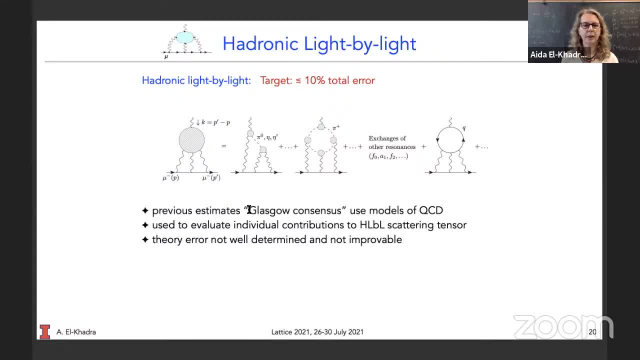 found in the standard model and all the measurements, the measurement of the light, count them correctly And then it could actually rescue the standard model And it could bring the standard model into agreement with the experimental measurements. So this was a big question mark prior. 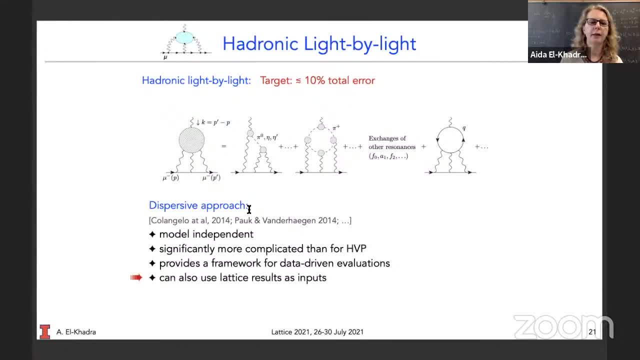 Excuse me, And uh, now there is a dispersive approach that was being developed in the mid 2010s and refined as a result of the theory initiative activities, which provides for a model independent uh inclusion and then additional consideration, but also seems to be a 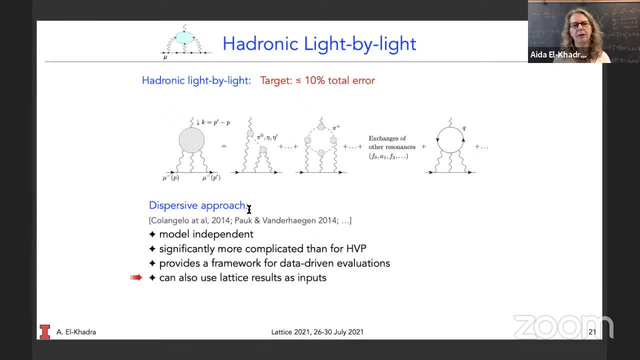 approach similar to the hydronic vacuum polarization. It's much more complicated because you're dealing with a four-point function instead of a two-point function, But that framework then allows for a data-driven evaluation if you have enough experimental data. Also interestingly is that one can use lattice inputs. 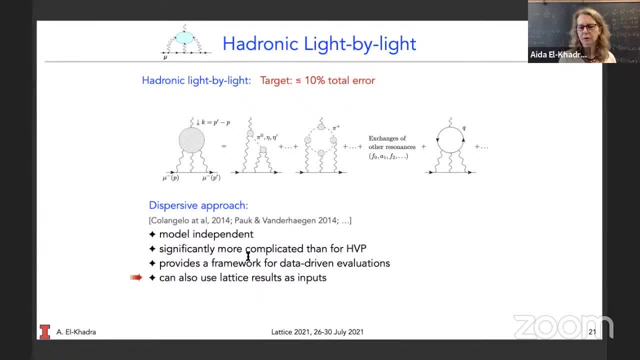 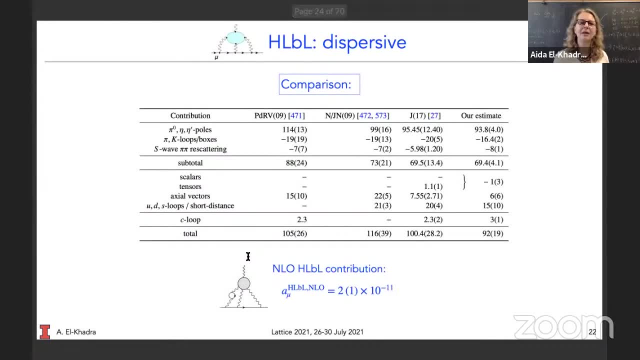 lattice results, lattice calculations as inputs into this dispersive approach. I don't want to spend too much time on this. This could very easily be a long seminar of its own, But here is a comparison table where you see the old model estimates and their spread. 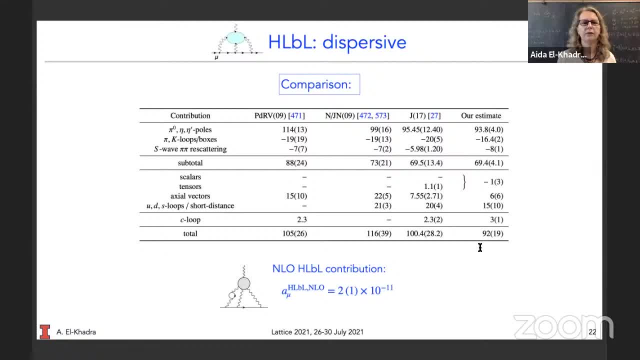 And here you see the results from the data-driven approach where basically the dominant contributions from the pion and pseudoscalar poles, from the pion and kaon loops and boxes and pi-pi rescattering in the S-wave are computed using lattice inputs and experimental inputs. 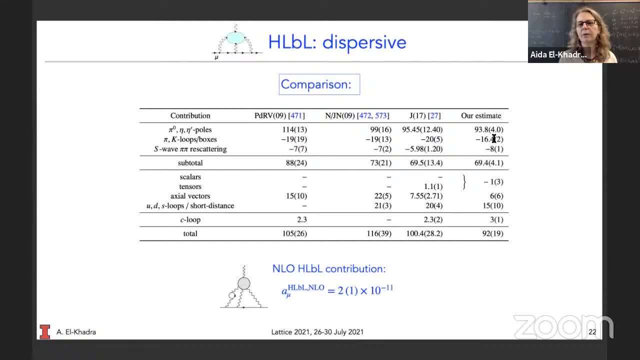 that are well enough known to obtain these, with these relatively small errors and well-quantified errors. So these contributions here, this error bar, is really well-quantified. We know where the errors come from and the errors, of course, can also be refined. 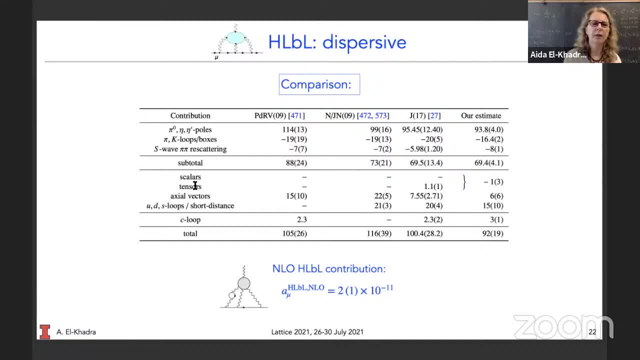 There are still contributions from the larger energy scales that are much smaller but much less well-quantified, And those are the main source of theory errors in the dispersive framework. So it's basically the errors of these contributions. These contributions are taken with essentially 100% error. 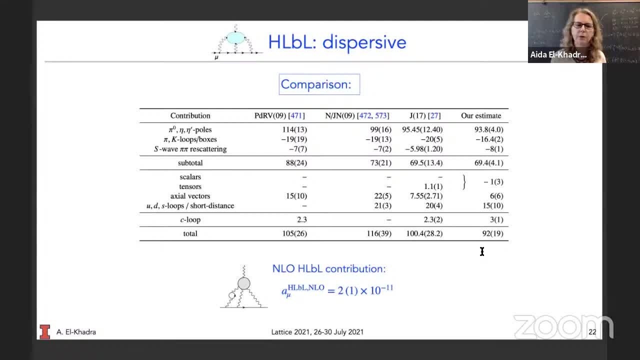 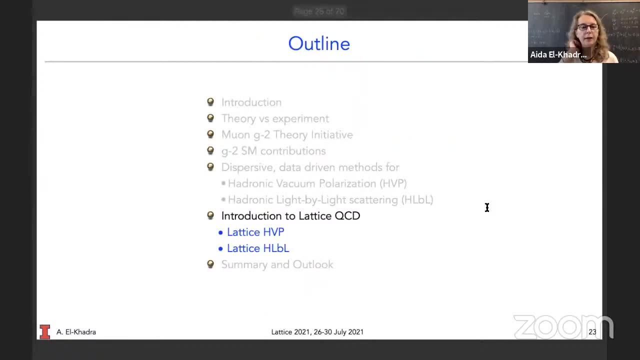 in order to obtain this estimate from the data-driven approach, The data-driven dispersive approach. So we can say now that the errors are almost well-quantified, but there are still pieces that need to be done better. So that is the situation of dispersive methods. 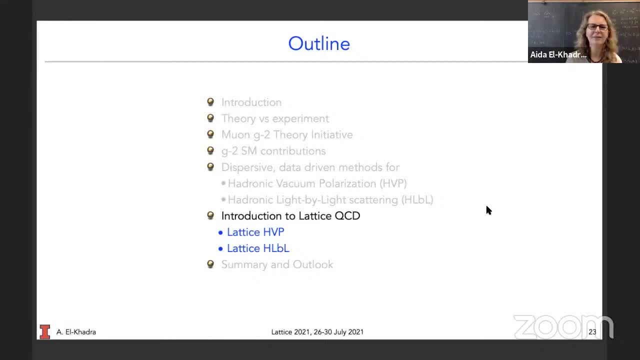 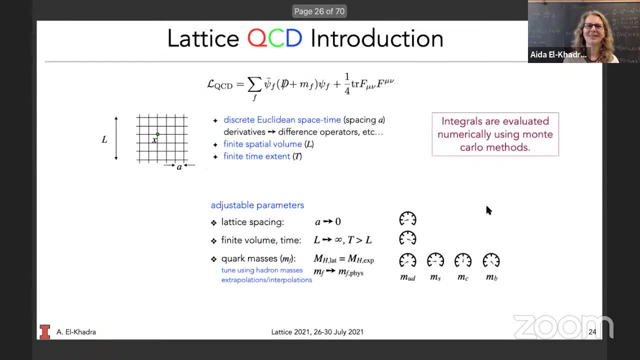 Let me now talk a little bit about lattice methods, starting with a lightning fast introduction to lattice QCD in two slides. So in lattice QCD, in lattice theory, spacetime is separated into discrete spacetime, lattice with next to nearest spacetime points being 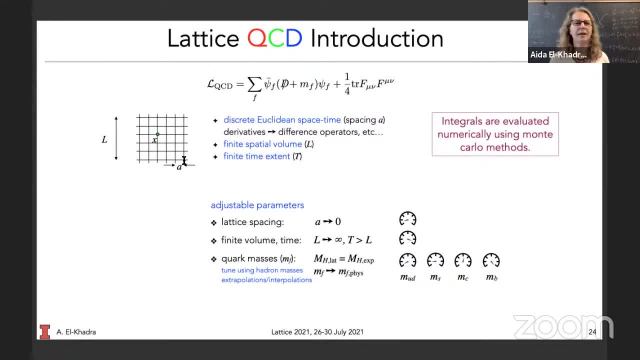 separated by a finite lattice spacing. So that's an approximation And that is needed in order to evaluate the integrals, the path integrals, numerically using Monte Carlo methods. So there are several approximations. There's the lattice spacing, Which is always called little a. 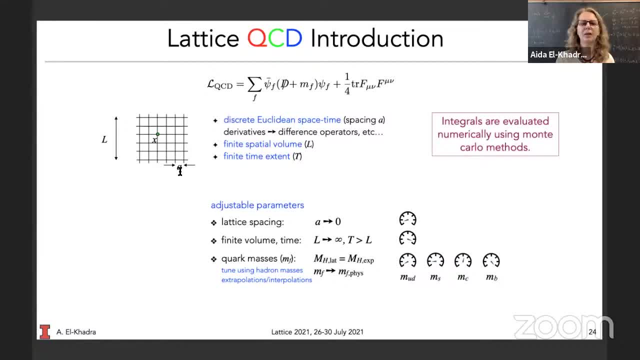 And so that's the same letter we use for the anomalous magnetic moment. So you have to understand what context a we're using. There's the finite volume and finite time extent. That also then turns the degrees of freedom into a large but finite number by which we can evaluate. 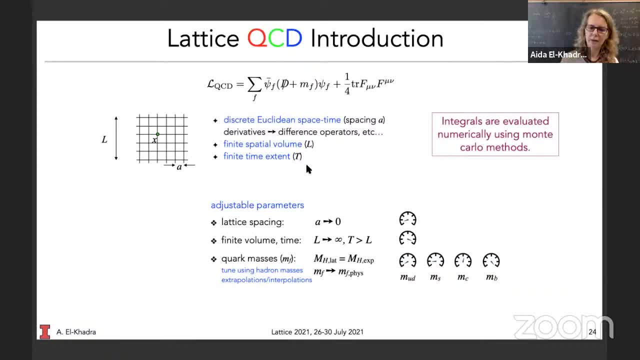 the integrals numerically Now, in order to make contact with the real world. of course, these approximations must be taken away, And the good thing is that we have to know that they come with adjustable parameters that can be studied. So, instead of doing one computation with one set, 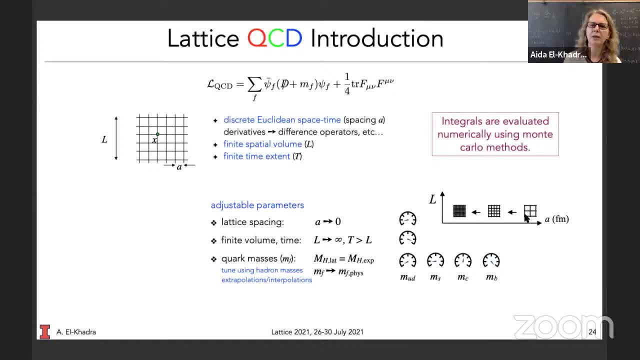 of parameters and lattice QCD computations, where we want to obtain results with quantified errors, we repeat our simulations, We repeat our Monte Carlo integrations over by varying these parameters. The other thing is that these adjustable parameters all come with an effective field theory that provides. 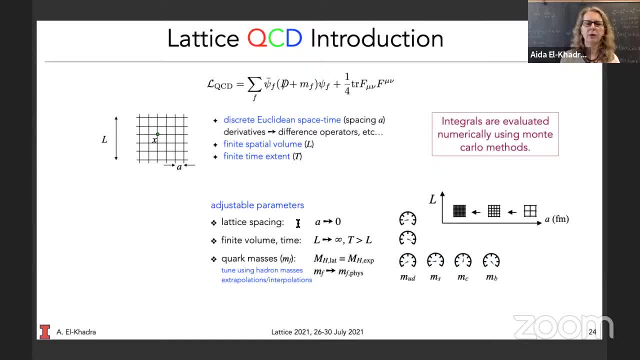 the underlying description of QCD, And so the effective field theory then guides the extrapolations or interpolations that is associated with these parameter variations. So the continuum limit is guided by semantic effective field theory. There are effective field theories for the finite volume and time as well. 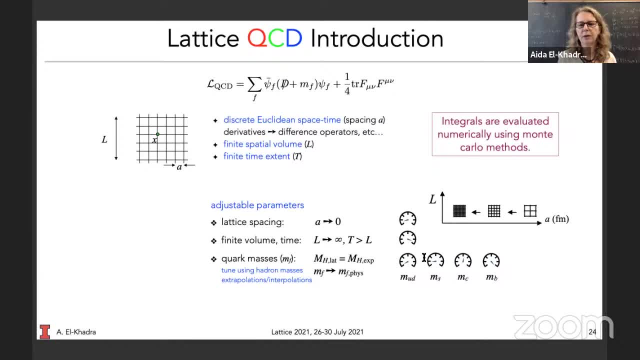 And the approach to the final volume, the final time. these are all associated with these parameters. variations to the physical up and down quark masses can be described by chiral perturbation theory, for example. So what this means, then, is that any lattice calculation 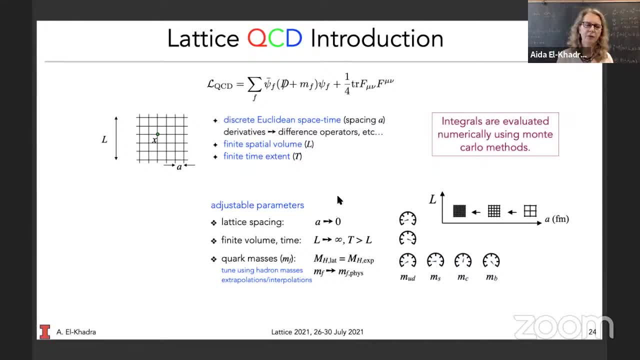 that claims to be quantitative. to have a quantitative estimate of the underlying uncertainties must be based on a computation of several ensembles where you vary these parameters And so over. on the left is an example of a section ensemble set that was created by the MILK collaboration. 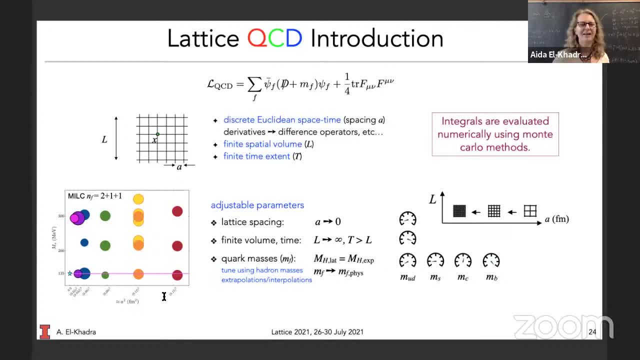 And this is just showing the ensemble parameters in two dimensions. So on the X-axis we're showing the lattice spacing and on the Y-axis the pion mass that is given by the masses of the underlying C quarks. So it's showing you this parameter and this parameter here. 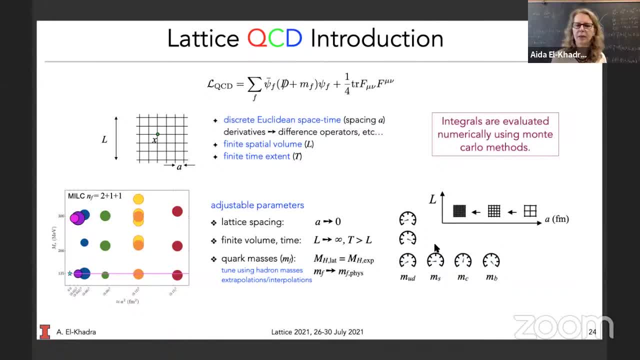 Obviously, you can also vary these other parameters and simulations, as C quarks are only included for the strange and the charm case And that's what's indicated in the two plus one plus one. the up and down quark masses are degenerate and that's the two. 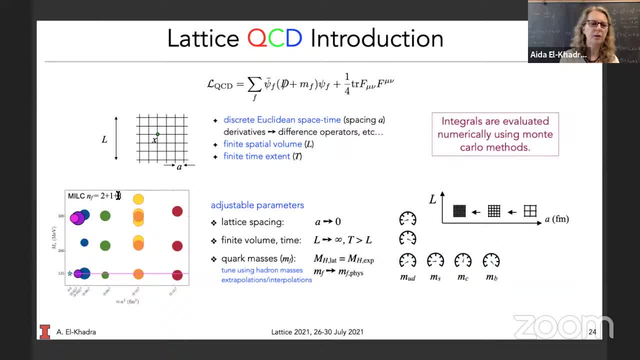 And then there is a C quark for describing the strange and the C quark describing the charm, The charm effect. the C quark effects of bottom, bottom quarks can be estimated perturbatively. So this is a large ensemble set. 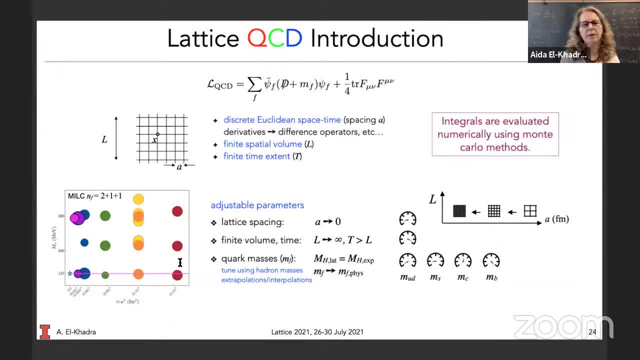 Then what is also shown here is the size of these circles indicates how much time we spend on the Monte Carlo integrations. The bigger the circle, the smaller the statistical error, basically. And then over here is the science star indicates the physical point in these two parameter sets. 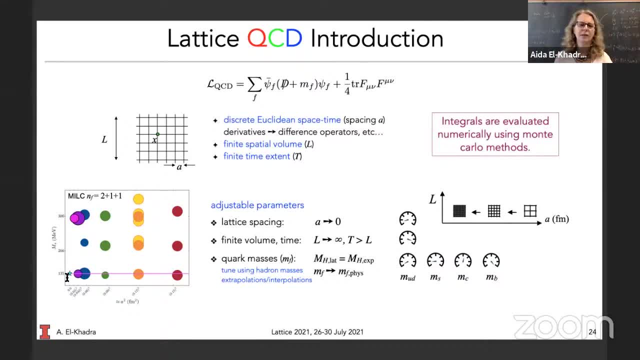 You can add more dimension to this. you can add more dimensions to show the finite volumes et cetera as well, But this is just an illustration. So with such a large ensemble set, with all of these different parameter variations, taking the continuum, infinite volume, 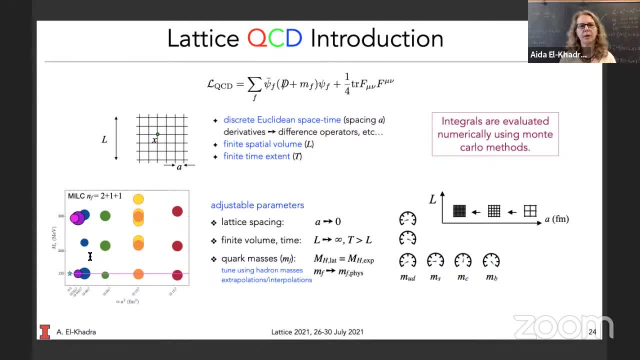 and interpolating to the physical masses is something that can be done reliably with quantified errors. Doing this, then, is what we mean when we say that lattice QCD computations provide us an ab initio picture of QCD. So what is the state of the art? 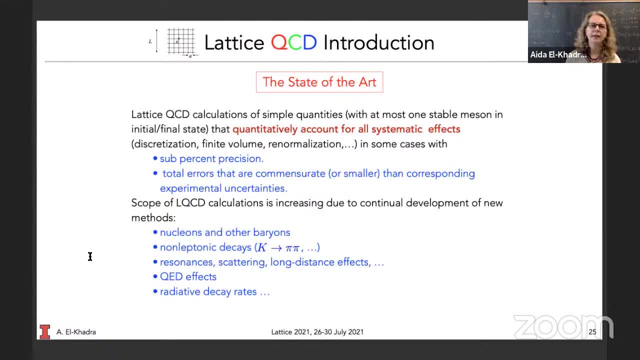 Lattice QCD calculations have progressed within the last decade to provide us computations of very simple quantities involving stable mesons in the initial and final state, with this quantitative accounting for all systematic effects, And we have results of very simple quantities, for example the decay constant. 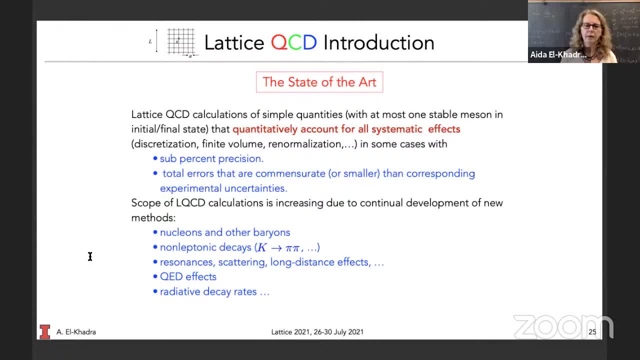 of a pylons, a pion and a kaon, where the errors from the lattice calculations are at the sub-percent and also sub-half percent, like 0.2% errors In some cases the errors from lattice calculations of the hedronic quantities that would be needed. 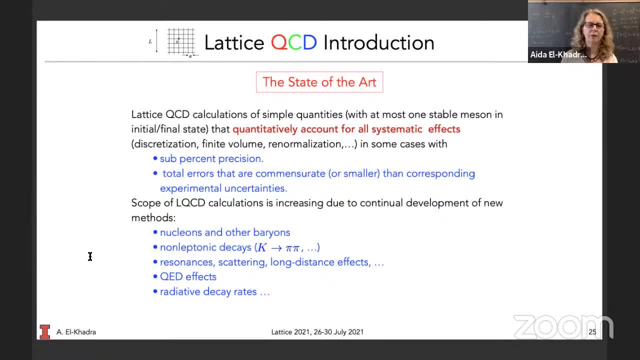 to compare with experiment, are smaller than the experimental uncertainties. So in this background, then, it makes sense to also use lattice QCD methods for the hedronic vacuum polarization which has such demanding precision needs. Okay, so part of this scope, then, part of this progress then, also means: 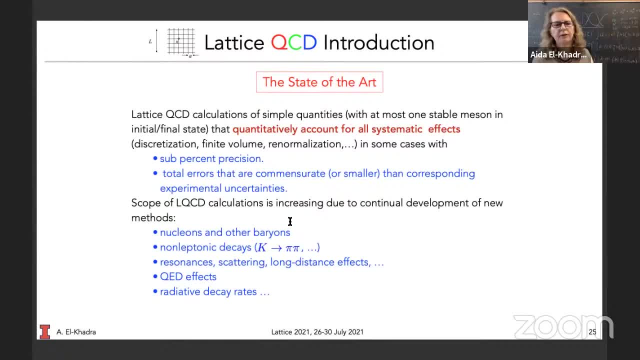 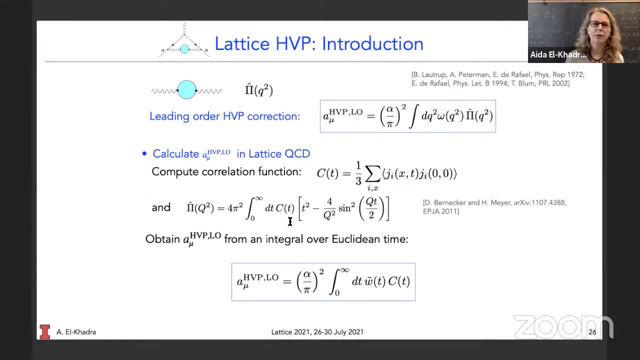 that the scope of lattice QCD calculations has increased very rapidly in the last decade. of lattice QCD computations where the uncertainties are quantifiable. So going back to, going back to the hydronic vacuum polarization function, then there's some small, some differences. 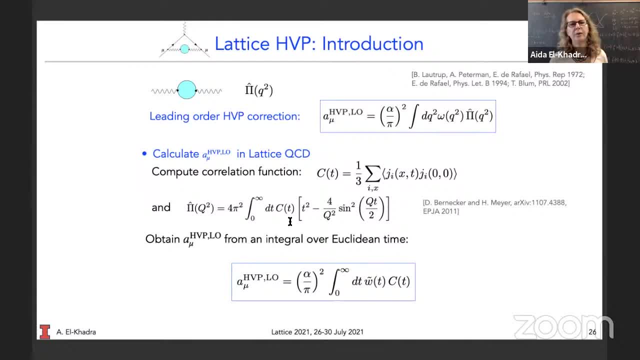 between how this is evaluated when we use lattice QCD, where we live in Euclidean space, And one can then rewrite this as an integral over Euclidean, over Euclidean momenta or even Euclidean time, as is done here. So in the in lattice QCD we can very straightforwardly compute. 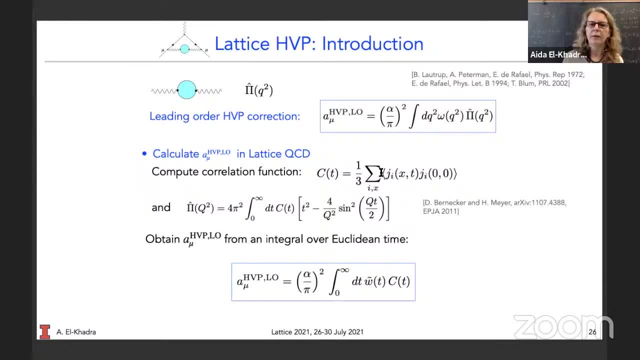 a correlation function like this, where this is the electromagnetic current over here as a function of space and time, some over space to compute this as a function of Euclidean time. So basically, here and here at rest, this is the basic quantity that we compute on the lattice. 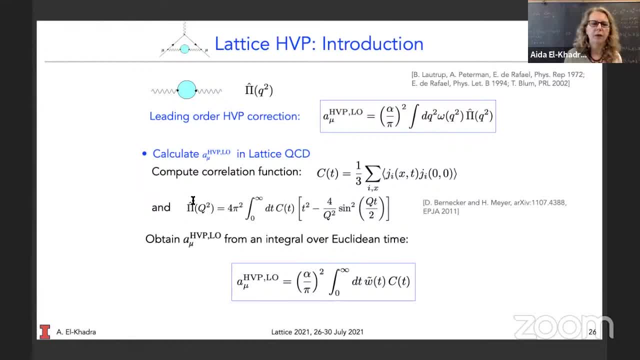 which we we can then use via Fourier transform to obtain the vacuum polarization function or plug in directly and rearrange the integration boundaries to plug it into the integral to obtain the hydronic vacuum polarization. So the currents here of course include all of the flavors. 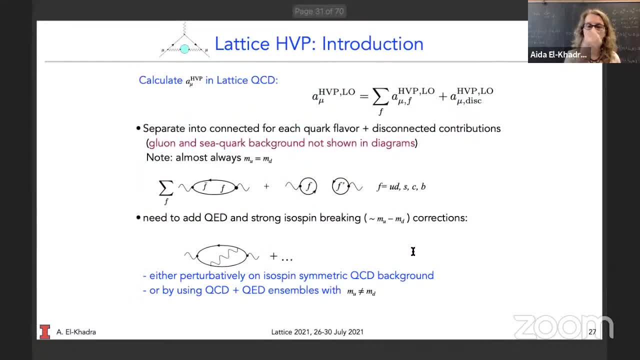 the quark flavors that are needed. So a lattice computation proceeds along a different breakdown from data-driven dispersive methods. Well we're, we're summing over all of the different hydronic channels Here. we are summing over the different. 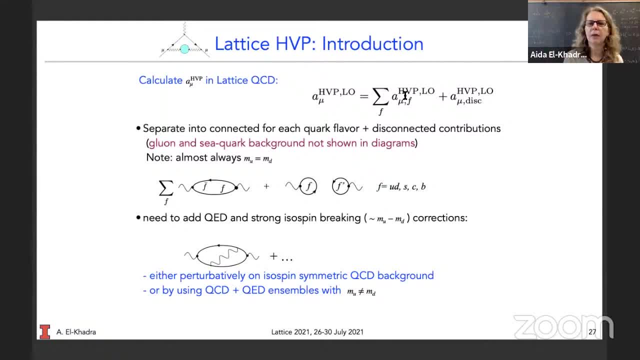 flavors. and it also makes sense to separate disconnected, disconnected contributions, disconnected weak contractions from the connected ones. So I'm showing here these diagrams where, implicitly, there's a gluon and seq quark background that's not shown. These diagrams are then computed. 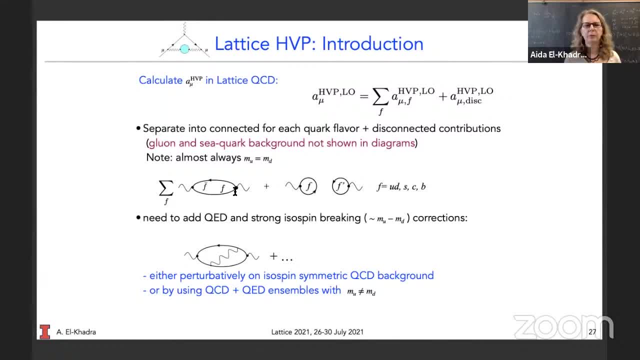 on the, the quark-luon vacuum that is produced by the Monte Carlo simulation. So here's the connected and the disconnected diagrams. Since these simulations are obtained in the isospin limit and often without QED in them, those corrections must also be computed and are often computed separately. 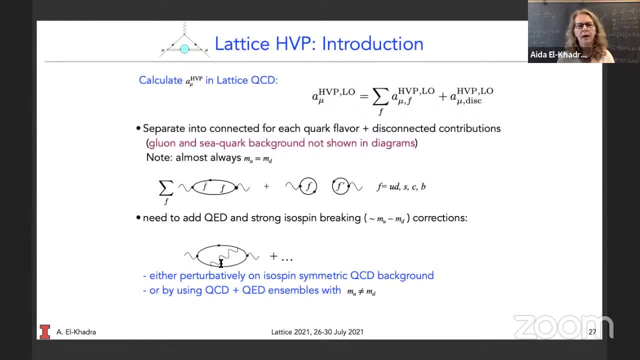 So because each of these different contributions have their own systematic error, the analysis and the way that systematic and statistical errors enter, it makes sense to compute the different flavor contributions, disconnected QED and strong isospin contributions separately and then add them all up to obtain the total AMU. 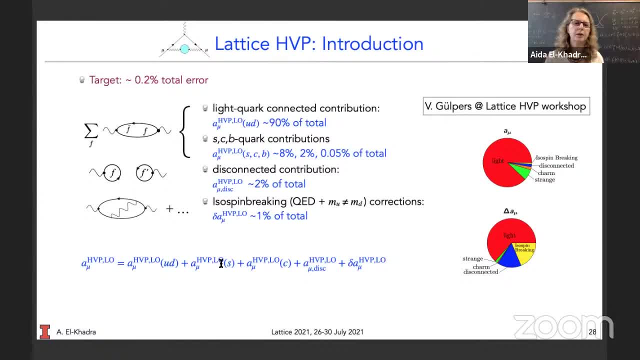 So that's the general strategy, how these things proceed on the lattice, And here I'm just giving you a rough breakdown. The light quark connected contribution. not surprisingly given that in the data-driven approach it is dominated by two pion contributions. 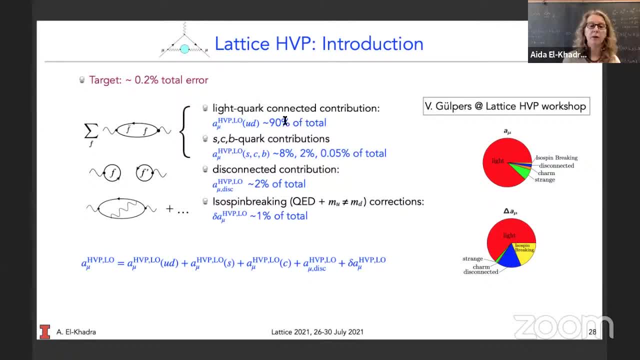 provides us with 90% of the total hydronic vacuum polarization contributions, followed by about 10%, for strange charm. and then the b-quark contributions are really really small. Disconnected is about 2%, and the isospin breaking and QED contributions make up about 1%. 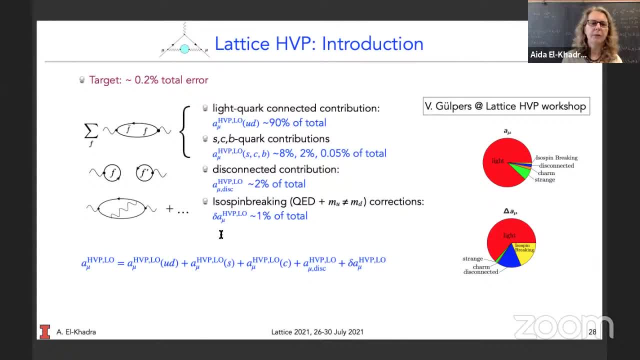 So the precision demands, then, of these different contributions are different. For the 90% of the total, we really must compute it with the precision, the ultimate precision that we need, but we can compute 1% of the total with a precision of 10%, and that's good enough. 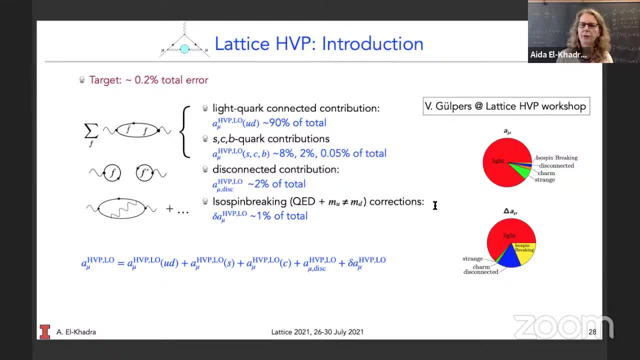 And here's a pie chart breakdown of the different contributions and the error contributions, of the status of the white paper And you can see the contributions to AMU, the light core contribution at 90%, et cetera. And what you also see is that some of the subleading, like isospin. 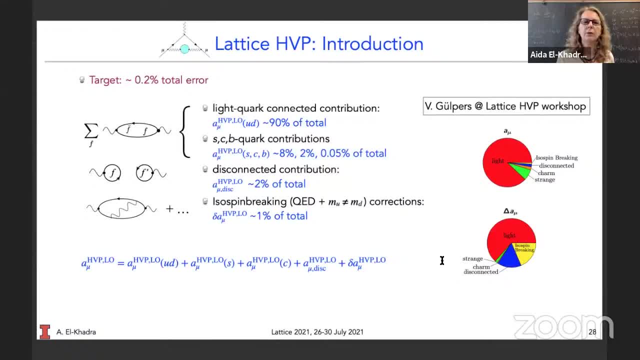 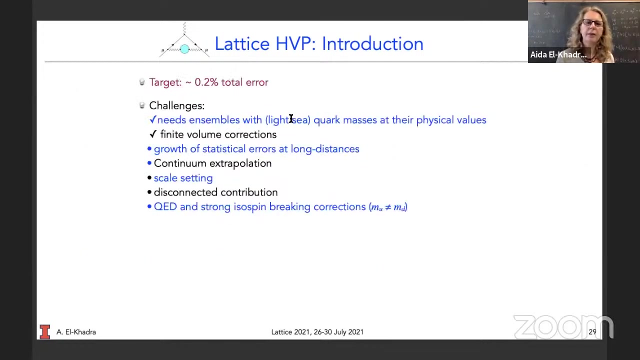 and disconnected contributions. we're still not known with quite the accuracy with which we need them to be, So improving those will be important in improving the overall accuracy to the precision goal, And the dominant uncertainty still comes from the light quark contributions. None of this is particularly surprising, So the challenges are then: we really need ensembles. 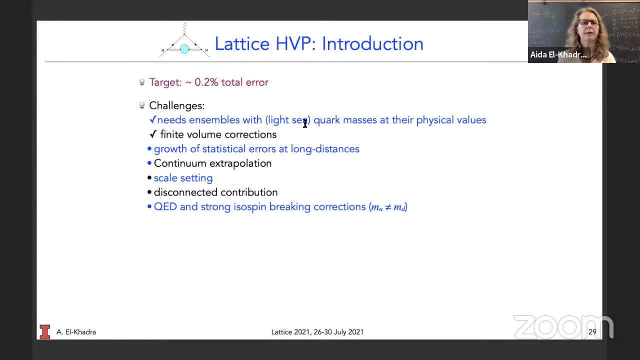 where the light C quark masses are at their physical values, And that's something that I have with a check mark, because there are several groups that have large ensemble sets. where that is the case, We need to carefully understand finite volume corrections. There is 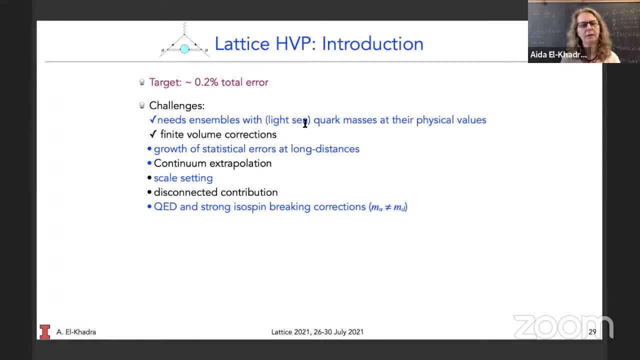 an issue with the growth of the light quark And we need to carefully understand finite volume corrections. There is an issue with the growth of statistical errors at long distances. The continuum extrapolation must be understood, of course, at the commensurate precision And that 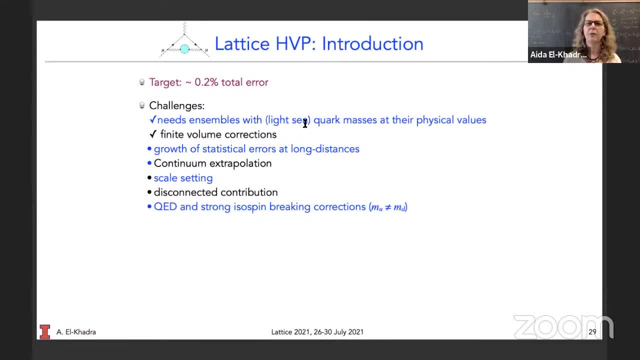 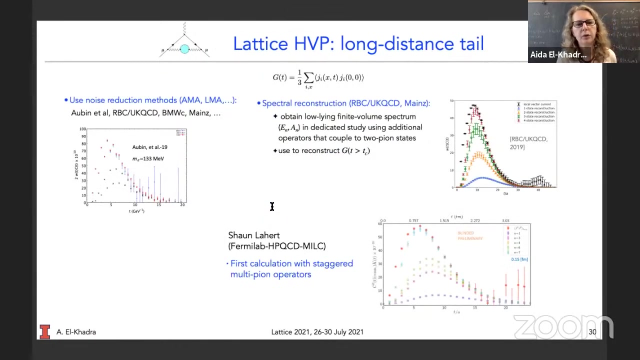 is rather demanding for a quantity like the hydronic vacuum polarization that receives contributions from all these different distance scales. And then understanding subleading uncertainty contributions and including the disconnected and QED I've already explained. So those are the challenges of the lattice computation. I'm going to skip over this. 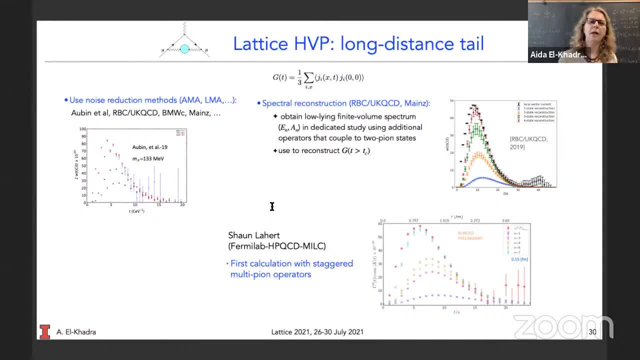 This is just an illustration of the amount of effort that has gone into to address all of the different challenges Here. the challenge that is posed by the growth of the statistical errors of the Euclidean correlation function for light quarks at large times, which then dominates. 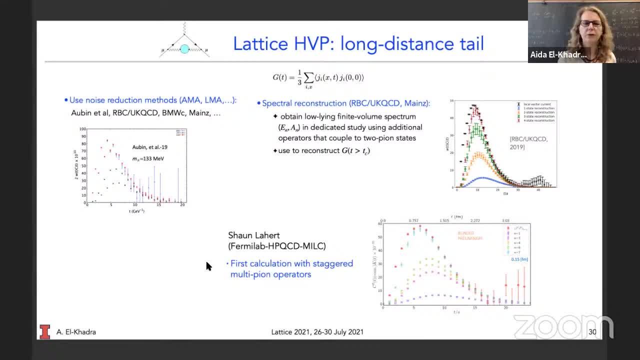 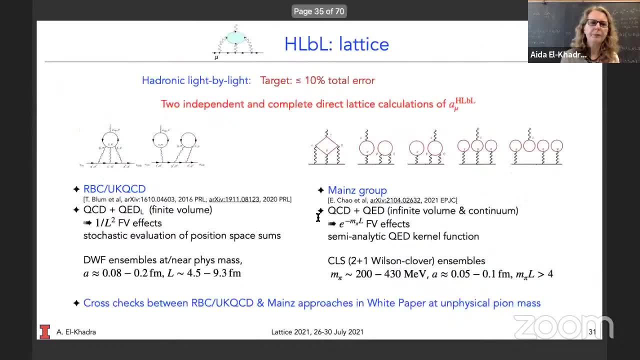 the statistical errors, And there are quite a few differences, So I'm going to skip over this, And then I'm going to go through a few different solution strategies that will lead to exquisitely precise results in the very near future. I would now like to come to the hydronic. 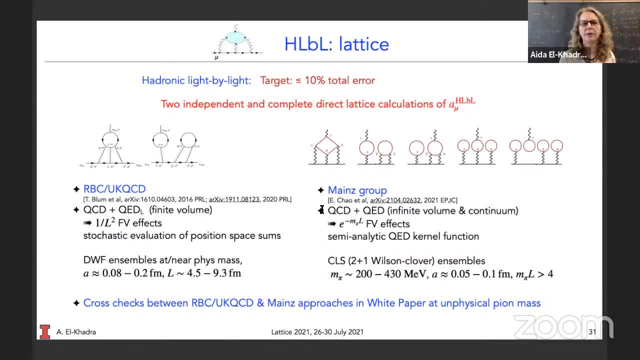 light by light, computed directly in lattice QCD, So computing these diagrams and their disconnected cousins directly. There are two groups who have done so, who have completed their lattice calculations of this quantum quark, And they are the two groups that have been willing to help to produce this very correctwork with the help of a RIBC-UK-QCD. 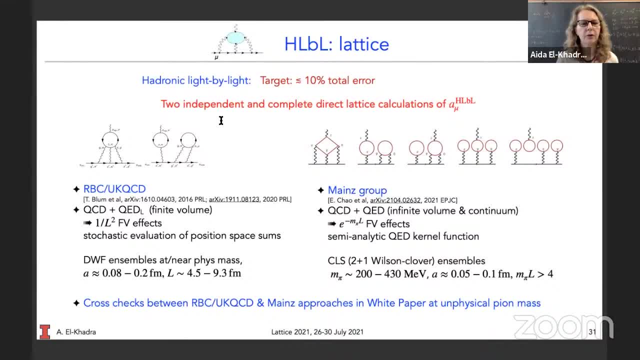 collaboration And the mines group. the RBC-UK-QCD collaboration published their results in 2020, and it was included in the white paper. the mines group posted their result within a day of the Fermilab announcement- Interestingly on archive- And this result is now published. The two groups 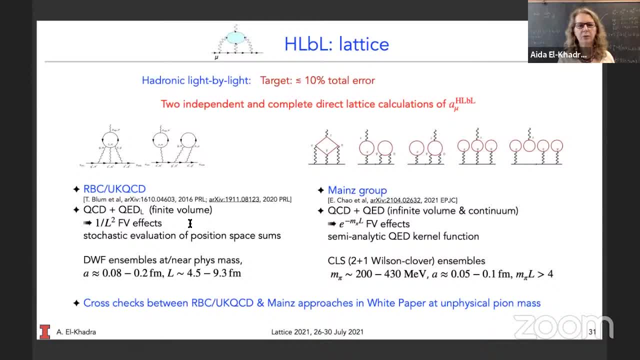 use different methods for dealing with the QED contributions. MIRIAM SAFIR- I will stop there and then we will move on. MIRIAM SAFIR- Thank you very much. MIRIAM SAFIR- Thank you very much. 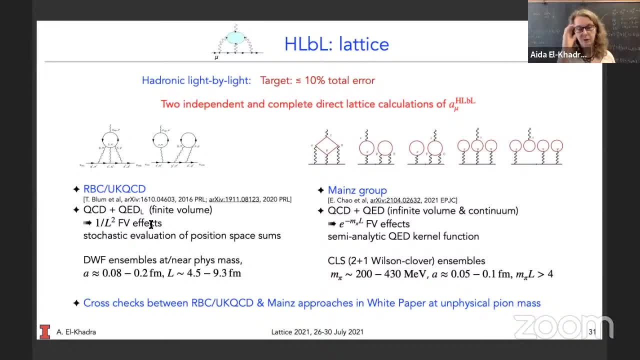 MIRIAM SAFIR- Thank you very much. RBC-UK QCD includes QED effects in a finite volume, which has of course an effect on finite volume effects. Those are much more serious. The Binds group has provided a semi-analytic QED kernel function in infinite volume. 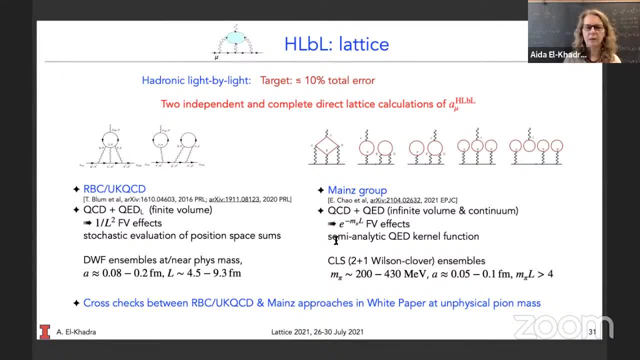 so their finite volume effects are the same as you have in QCD. They use different ensembles that they generated independently. In one case the ensembles are at or near physical mass. In the other case the ensembles have pions, C pions, in them. 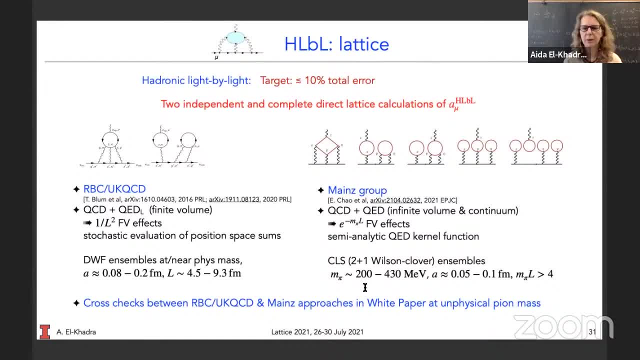 that are larger than the physical pions and you need to obtain a chiral extrapolation to the physical point still, And there have also been cross-checks between the two groups that are part of QCD. So we have the white paper to check the methods against each other. 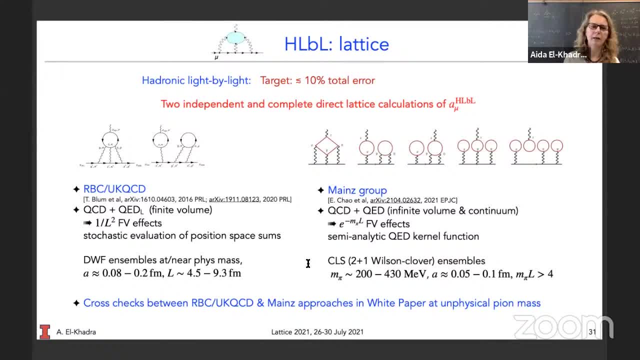 at unphysical pion masses And lead us to say that both groups have also made sure, have also debugged their methods by just computing the pure QED loops to see that they agree with the exactly computed perturbative results. So all of these checks have been done. 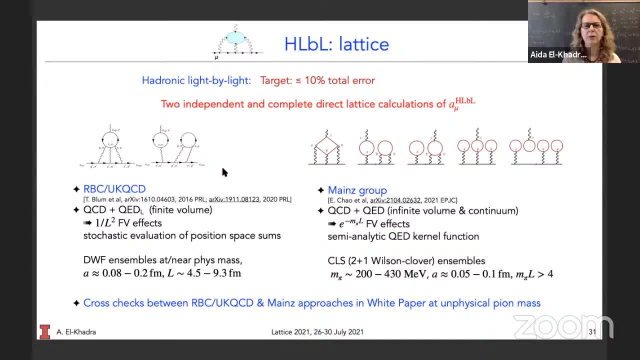 and we are now in the fortunate position to have to complete independent calculations of the hydronic light-by-light. I note that, even though this is a four-point function which is very, very challenging to compute in lattice QCD, the overall precision goals are much less demanding. 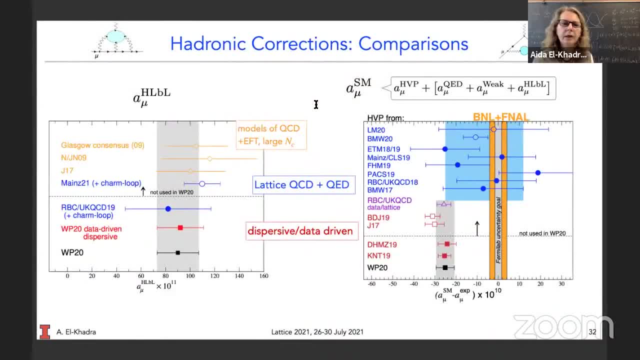 than for the hydronic vacuum polarization. So here now is a summary of the situation for the hydronic light-by-light and the hydronic vacuum polarization. Let me start with the hydronic light-by-light. In orange we have the hydronic light-by-light. 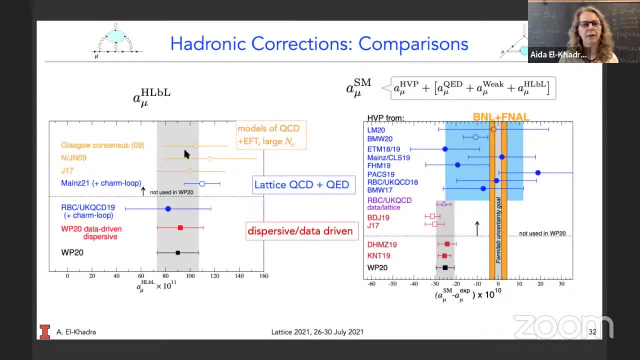 and in yellow we have the hydronic light-by-light And in yellow we have the hydronic light-by-light. In orange you see the old results that are based on models of QCD and some insights from effective field theory and chiral perturbation theory. 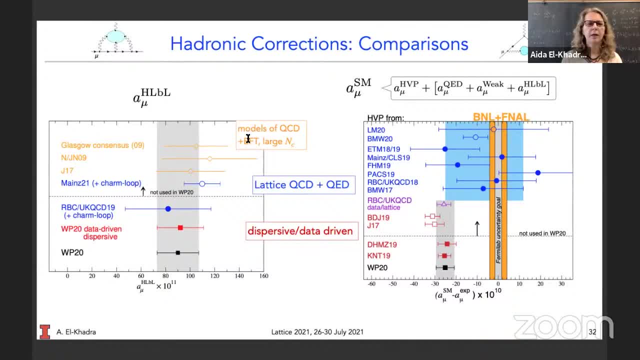 and using large NC arguments. And then there are the two points that are coming from lattice QCD. The red point here is the data-driven dispersive evaluation. in the white paper and in black you see the. the result, that is the, is the white paper. 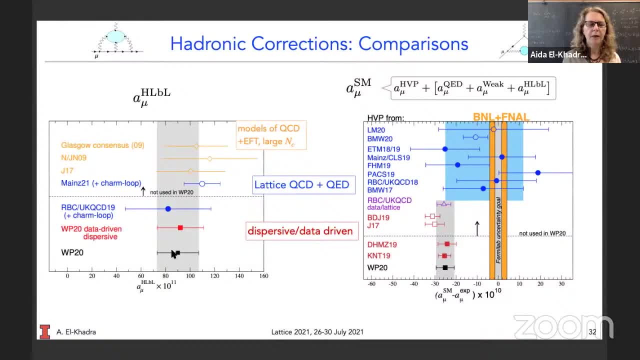 final result: the white paper average. The white paper average was obtained from combining this lattice QCD result with the data-driven result And you can see that the new result of course came out after the white paper is is completely consistent with this, with this white paper average. 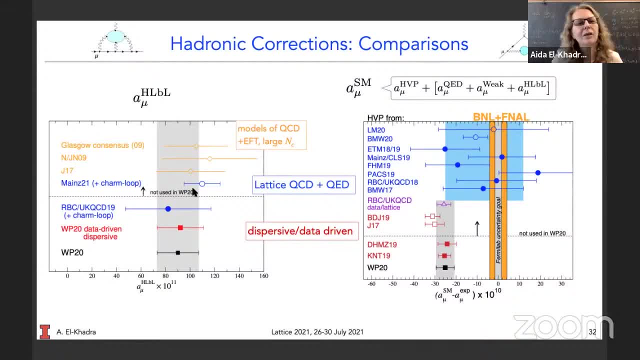 So we're now in a situation where, first of all, we can confirm that the old model-dependent results. actually they got the physics right. These are, you know, smart phenomenologists and the light-by-light contribution, the true light-by-light contribution. 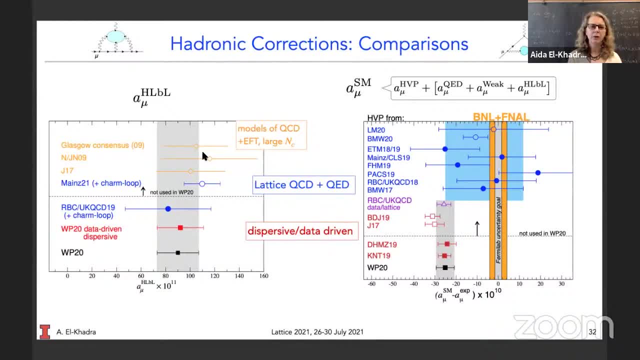 is right about where they said it would be, But now the errors are quantified and with a little bit more work, the errors will become more reliable and will be reduced. We now have two independent ways of obtaining this important quantity, and they all- they both- are in overall good agreement. 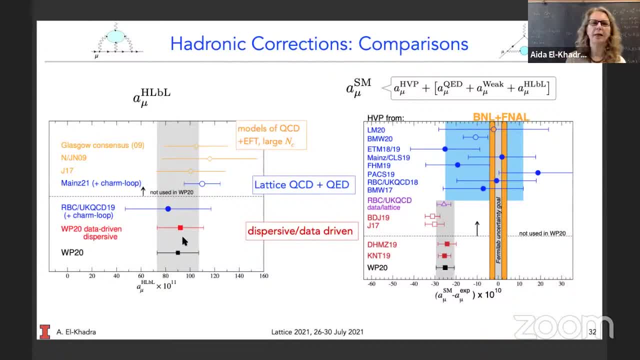 So can the hydronic light-by-light contribution rescue the standard model? The answer is no, it cannot. It is. its value is, you know, close to a hundred times 10 to the minus 11 in in in these units you know will stay there. 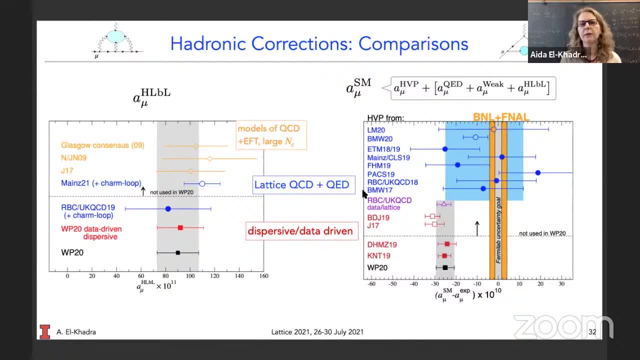 With an error that will become better and better. Now for the hydronic vacuums. for the hydronic vacuum polarization, the situation is a little bit different. In red you see the data-driven evaluations that form the basis of the white paper. 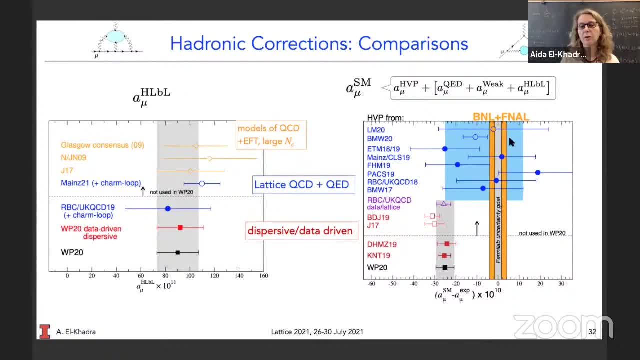 And in blue you see the lattice computations, which have errors that are too large to actually quantitatively weigh in by the time of the white paper came out, And so the white paper evaluation is then based on these data-driven evaluations, with the conservative merging procedure that I showed you. 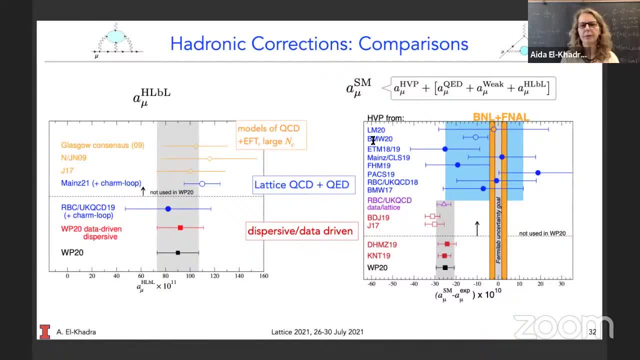 By the time the white paper was finalized, the BMW collaboration posted on archive a new computation, which has subsequently changed a little bit. What I'm showing here is the version three that was published in the in Nature a day after the Fermilab experiments. announcement. 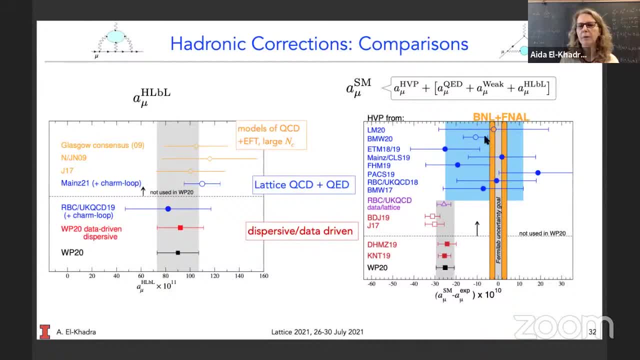 And you can see that this result is compatible with a new experimental average. compatible-ish- It's about one and a half sigma tension and also compatible-ish, if you want, overall with the data-driven results, but in larger tension of about 2.2 sigma. 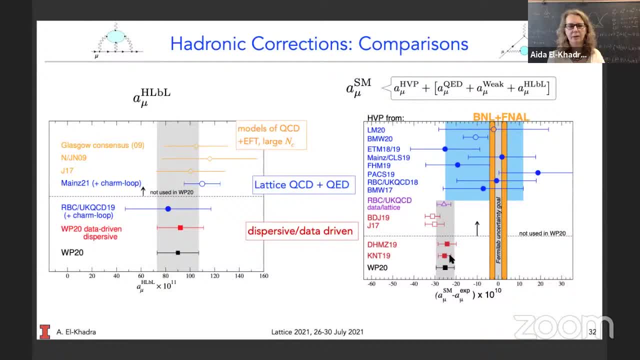 And so this is a situation that you know has been the subject of a lot of discussion and, and will be, will continue to be scrutinized. What I would like to say here is that the BMW collaborations result, impressive as it is, needs to be scrutinized. 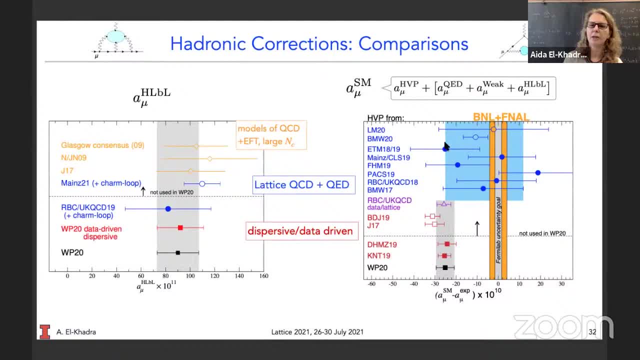 and we need to have other lattice calculations with commensurate precision to really make sure that all of the methods that are basically driven to the edge of the of the you know allowed precision, that all of that we have good agreement between different lattice results for this. 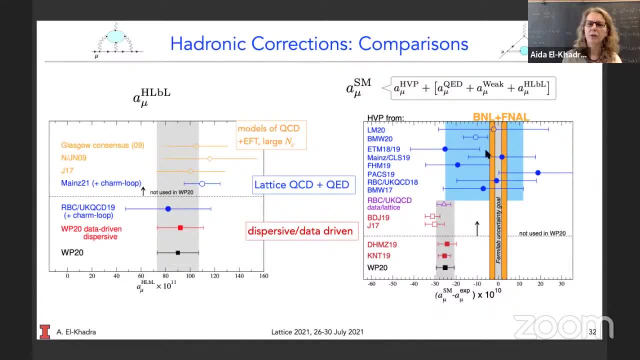 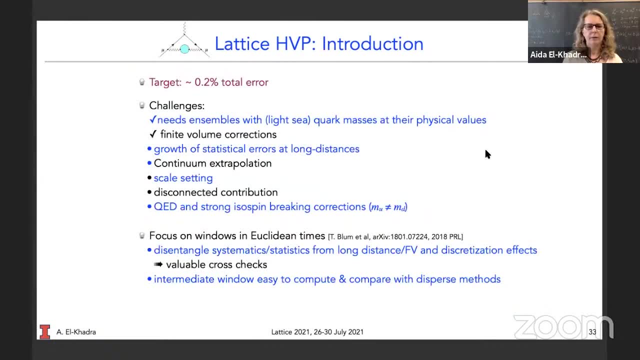 before we can actually draw firm quantitative conclusions from this result. So one of the ways in which we're scrutinizing the, the results and the tensions between data-driven and lattice results, and also between different lattice results, is by focusing on on Euclidean windows in time. 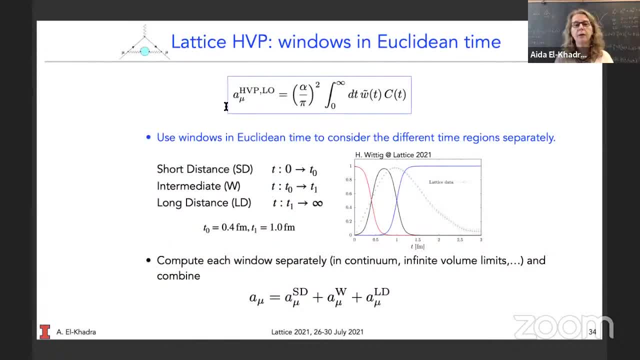 Recall that we compute on the lattice, the hydronic vacuum polarization from, from this integral over Euclidean time, And we can look at windows of Euclidean time to isolate different distance scales and scrutinize them in more detail and also understand how the different systematic errors contribute. 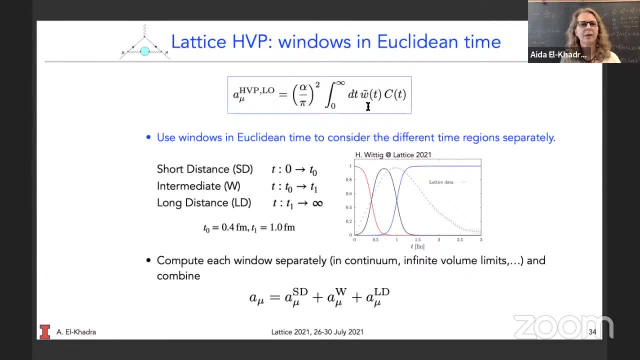 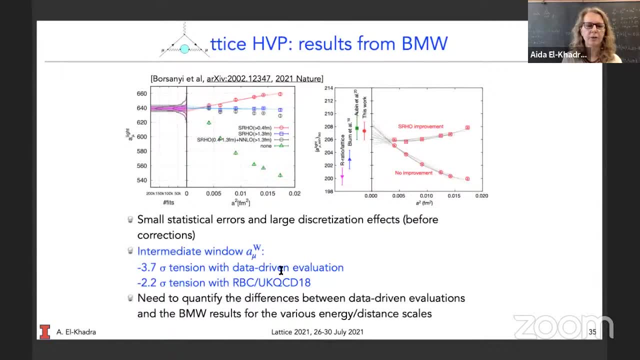 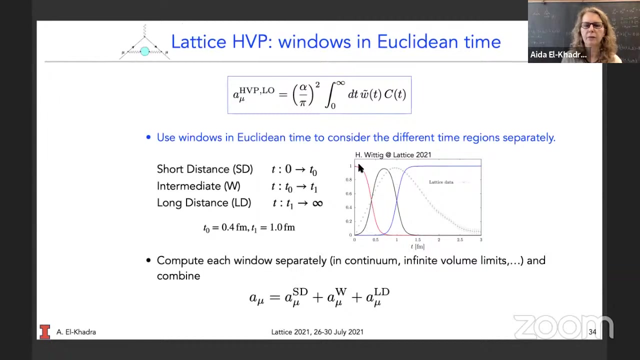 differently. So that is still something that is actively being investigated And in particular, this reveals a large discrepancy with data-driven methods and with the BMW collaborations. result for the intermediate window. The intermediate window is basically this one here, So it is not sensitive to short distance discretization effects. 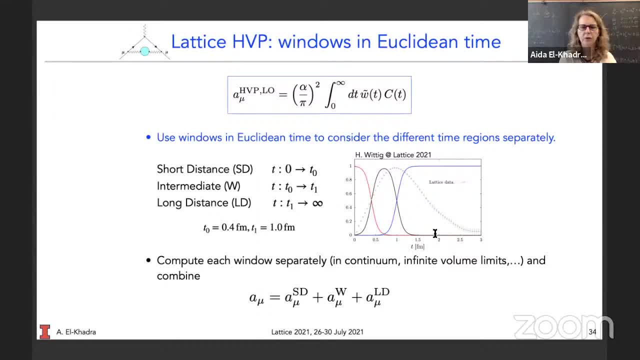 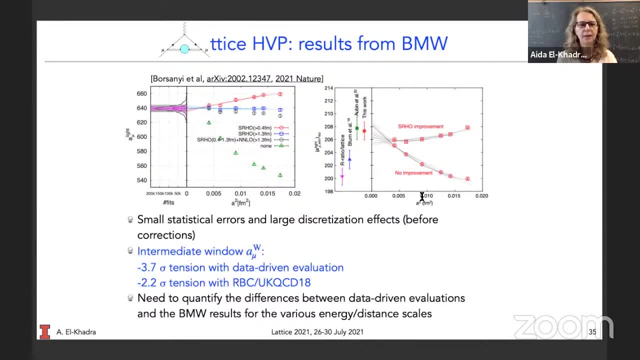 and less sensitive to finite volume and statistical effects at large distances, So it can be computed using lattice QCD methods more precisely than the overall, And so there are some tensions here that need to be understood. So that is the current situation for the hydronic vacuum polarization. 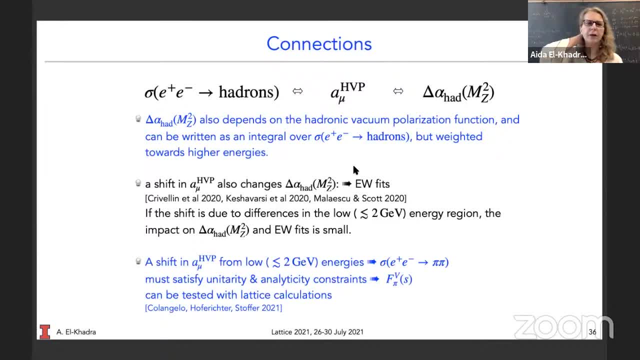 I would also like to point out very quickly that changing the hydronic vacuum polarization has an effect also on electroweak fits And there is an important interplay via the dispersion relations between the hydronic cross sections. the hydronic vacuum polarization contribution to A mu. 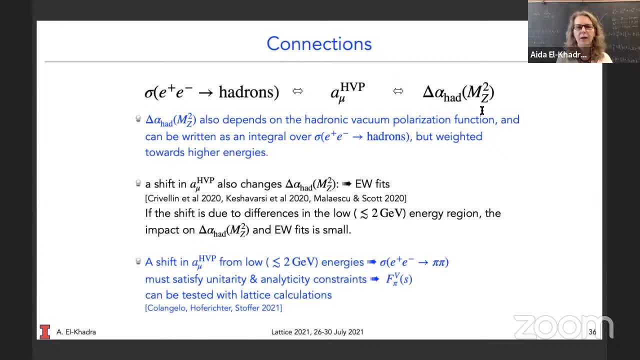 and the hydronic contributions to the running of alpha. All of these are interconnected And having a puzzle in one, you know, having a change in one then- also implies changes in the other, And those changes would need to be understood if these tensions persist. 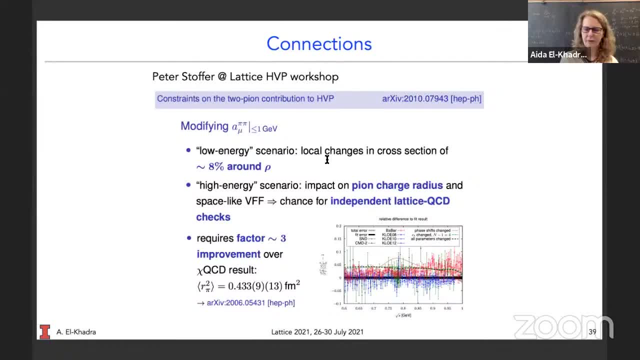 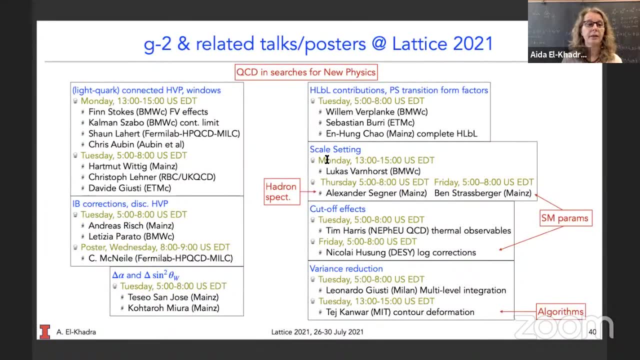 I am going to skip this for now, given that I am running a little bit late. This slide is just to show you that there is a large effort by the Lattice community. Here you can see all of the talks that were given at the Lattice conference. 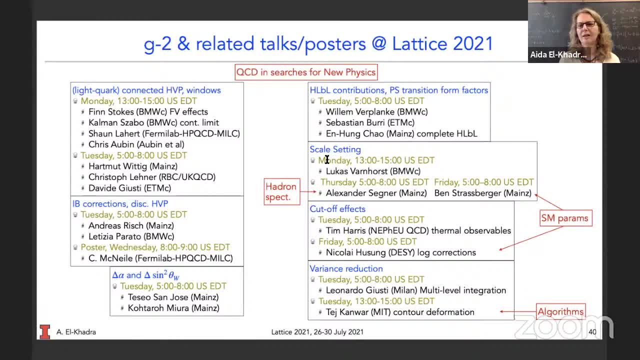 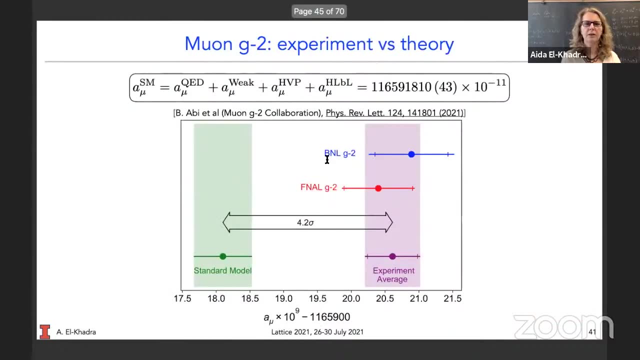 at the end of July, And these are just the parallel talks and posters. There were also two plenary talks on this topic. So this is a priority for the Lattice community: to refine the hydronic corrections To aim you further from direct Lattice computations. 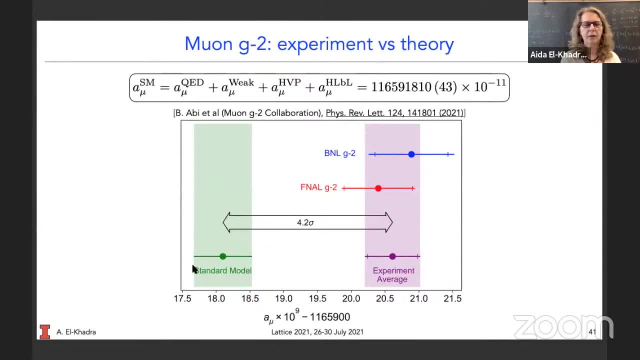 So for now, the standard model, the best standard model, evaluation, still is the white paper, And now we can, and so one should take this tension at face value for now- And there is a lot of work by people to explore the possible new physics scenarios that might give rise to this tension- 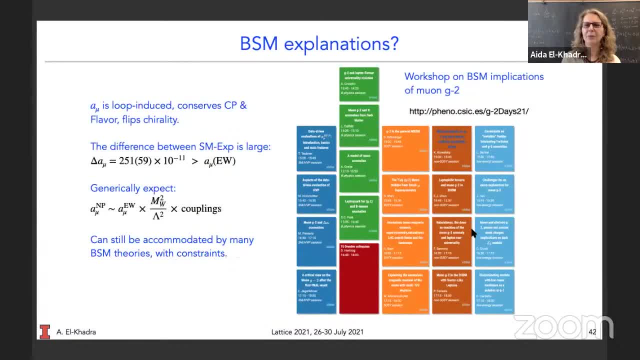 So there's a. there's been workshops on this with many different talks There are basically almost all of the different BSM scenarios can still be accommodated, but they are constrained. As a reminder, a mu- the anomalous magnetic moment of the muon is different. 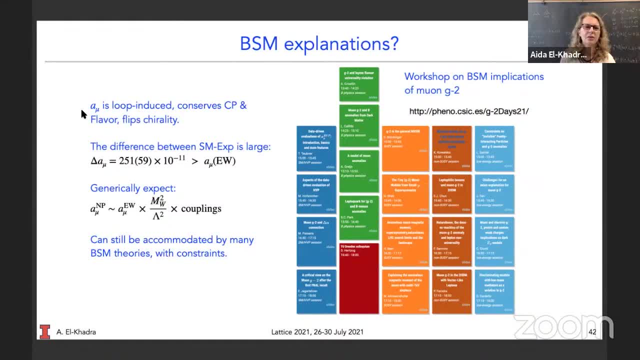 you know, has provides complimentary constraints. But the tension, this 4.2 Sigma tension, if you look at the numbers, this is: this is larger than the entire electroweak contribution. So it is large. It could become smaller and still be a good sign of new physics. 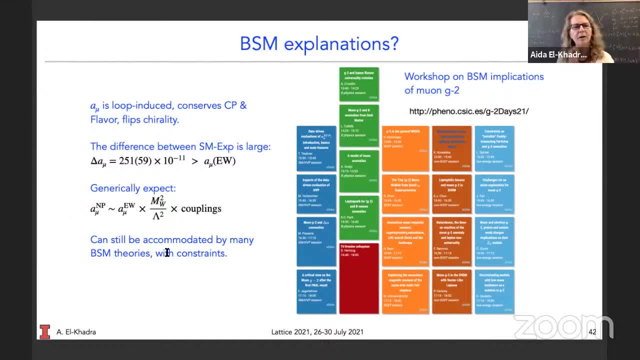 And accommodating this tension in beyond the standard model theories. is is a active area. There's a large community of phenomenologists working on this, with dozens of papers coming out almost every week. hundreds, hundreds of papers already haven't come out since the announcement of the 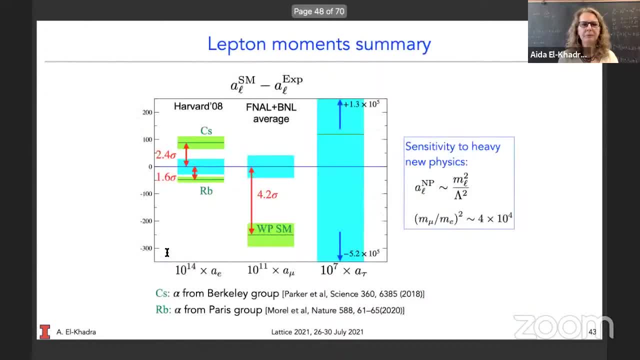 Fermilab experiment. I would also like to point out that there is an interesting development in recent years also for the anomalous magnetic moment of the electron. The precision here is much, much larger than for the muon, of course, but there are some interesting tensions that need to be resolved. 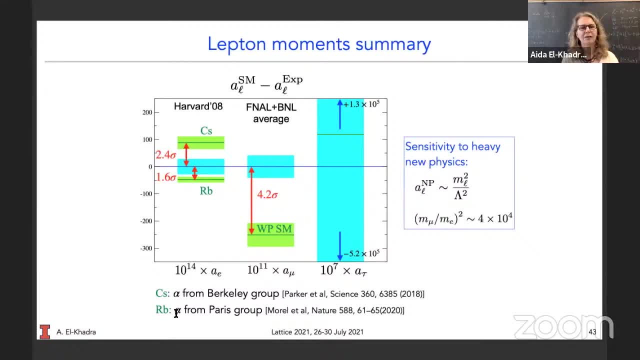 There are two different measurements of alpha that affect the standard model prediction for the electron. In the electrons case, the QED corrections are even more dominant than for the muon, The hydronic and electroweak corrections to the anomalous magnetic moment. 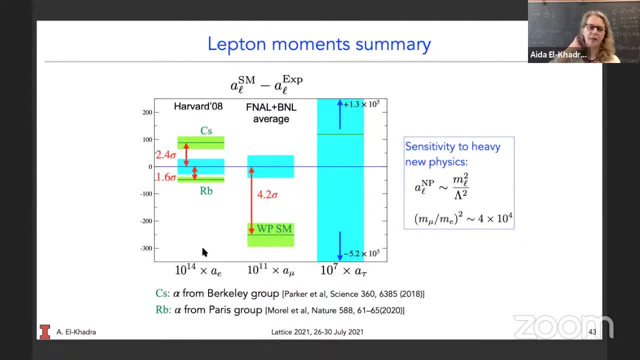 of the electron are suppressed because the electrons mass is so much smaller, But there's a five Sigma discrepancy between two measurements of alpha, leading to this situation here. So this is another space to watch these tensions. These differences are much larger from what you would expect by naive. 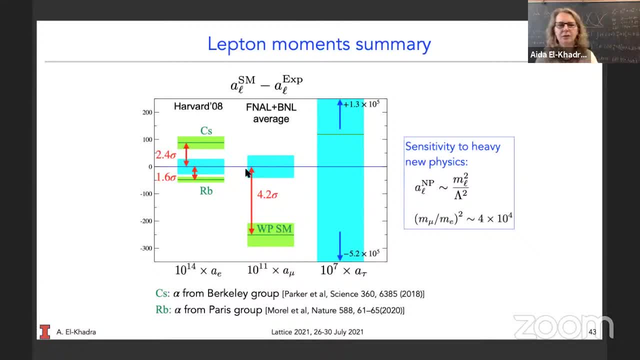 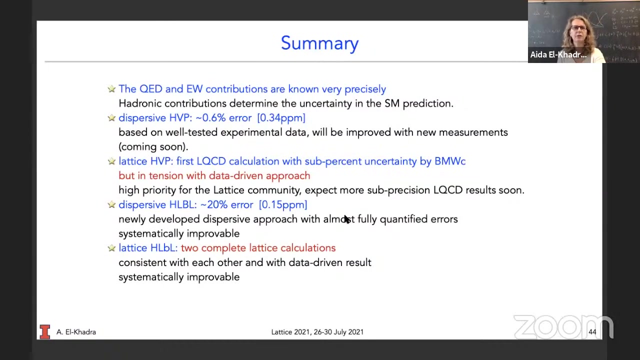 scaling of sensitivity to new physics And the Tau leptons. anomalous magnetic moment unfortunately is not measured, even with a precision that is close enough to be relevant because the Tau lepton decays so quickly. So let me summarize the situation: QED and electroweak contributions are known very precisely. 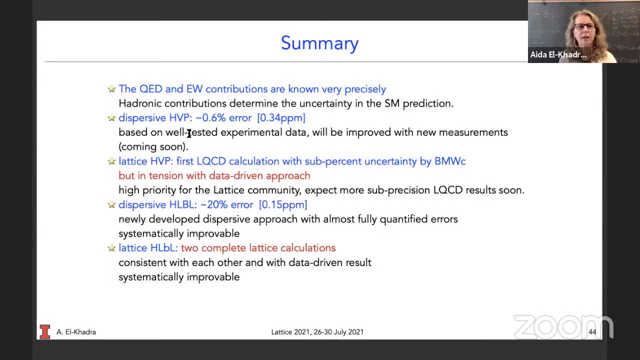 The best determination of the hydronic vacuum polarization comes from dispersive methods which are based on well-tested experimental data. There are some really annoying tensions between the data, but there will be new improved measurements coming out from Babar from bell two. 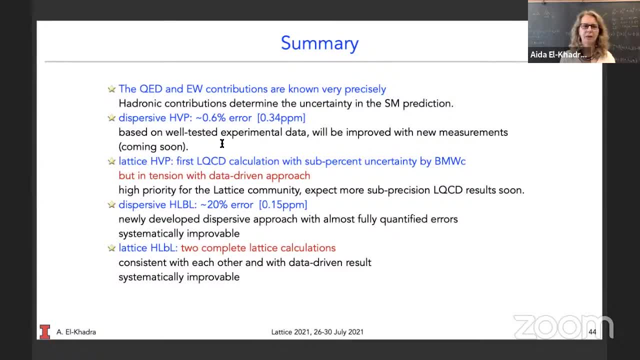 from best three from the Novosibirsk experiments. So hopefully the situation of the tensions between the data will be resolved and we will have even more precise data driven evaluations. I showed you the first lattice QCD computation of the HVP with sub. 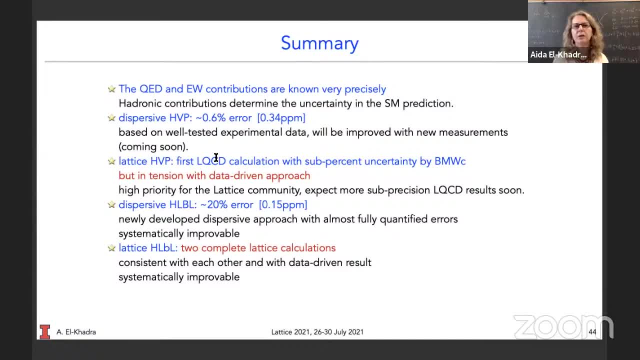 percent, just about sub percent uncertainty- 0.6%- which is, however, intention, with a data driven approach and, you know, wait for the lattice computation. In the HVP community, there are quite a few different groups that are in hot pursuit of these. 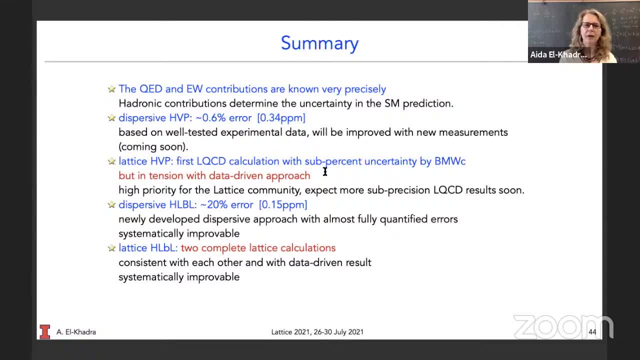 computations, including our group, And so we will have more information soon, And all of this information will go into a new, updated white paper. I also described the status of the dispersive light by light and the lattice light by light, which is basically now solved. 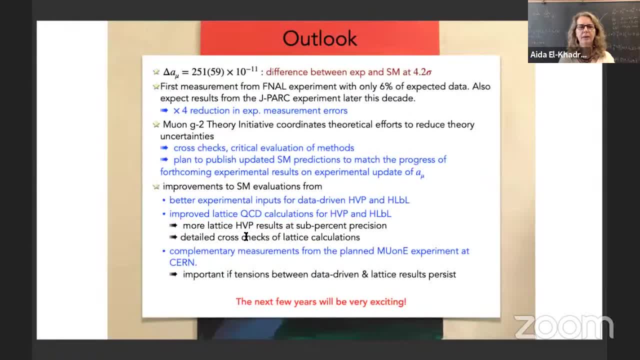 which is wonderful. And here is the overall- uh, overall- outlook. without repeating everything I already said, I wanted to just point out that, if there is if, which we don't know yet- but if subsequent lattice computations reveal a tension between data, 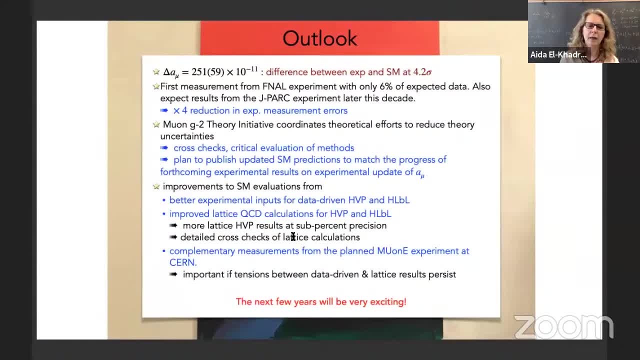 driven and lattice calculations. this is something we must understand. This affects, of course, the conclusions about where new physics is, and there will be further. There's a. there's a. there's a complimentary measurement planned by the muon experiment. 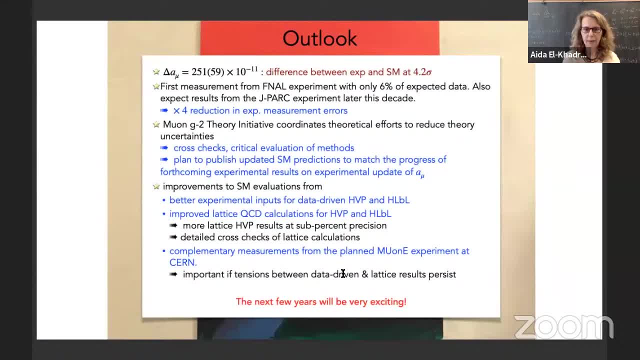 which will give us more information about the um, a different view about uh uh in the space, like region of um, of the hydronic vacuum polarization that doesn't use hydronic cross sections, So that will be very important as well. 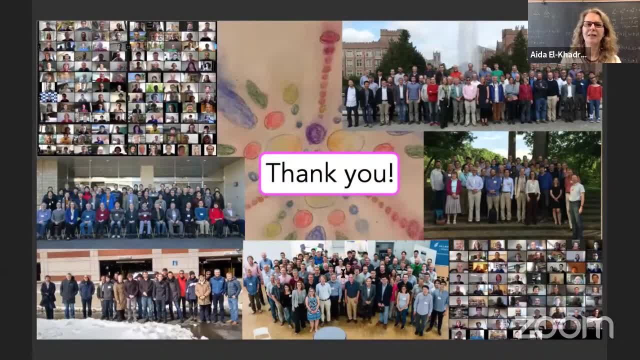 Um, I've mentioned the theory initiative There's been. this is a large, well large ish, you know, um, um, very robust, all of the, uh, the, um, the data of the universe, um, 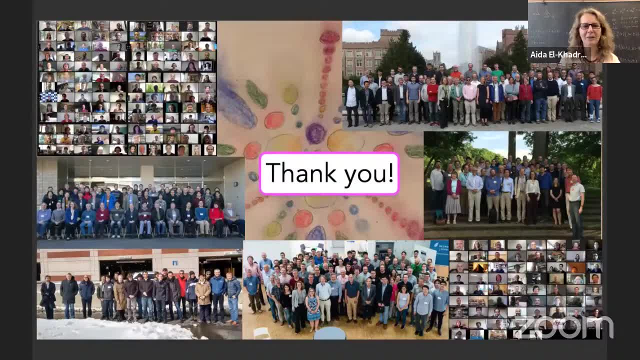 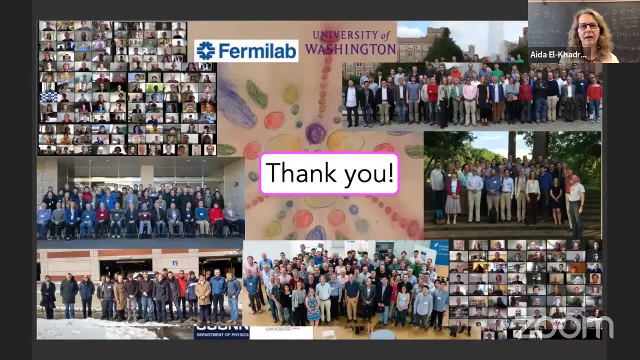 of thewed human uh of the universe, and and and the um of the, the of the time, the, you know, of the time of the time, um of the time of the time. 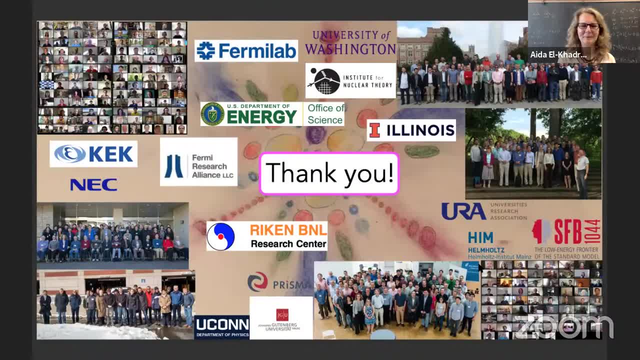 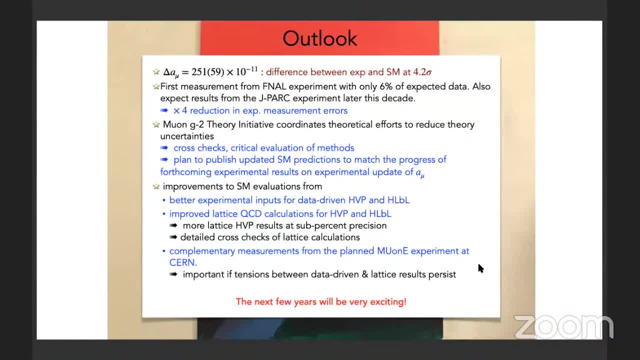 um, it will be much more helpful. uh, I'm going to go back to this. Thank you very much. Thank you very much. Nice, I don't know From the audience. now I have a question. Is there any question here? 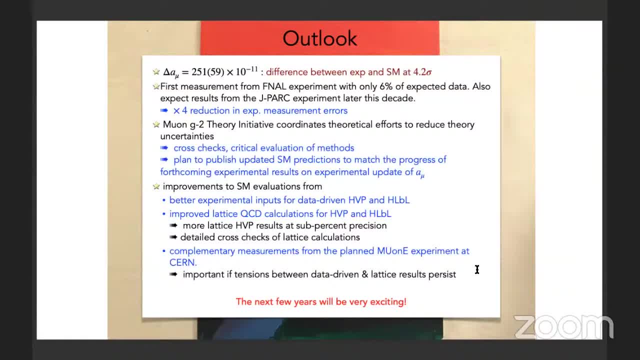 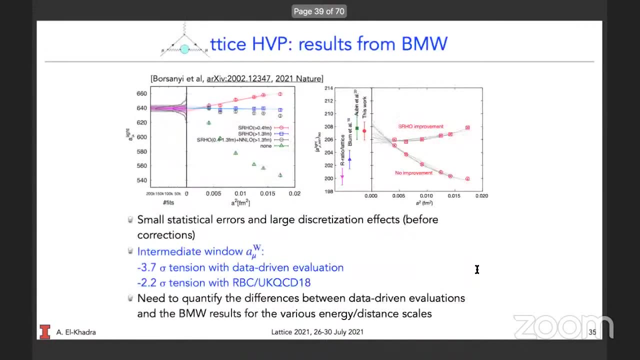 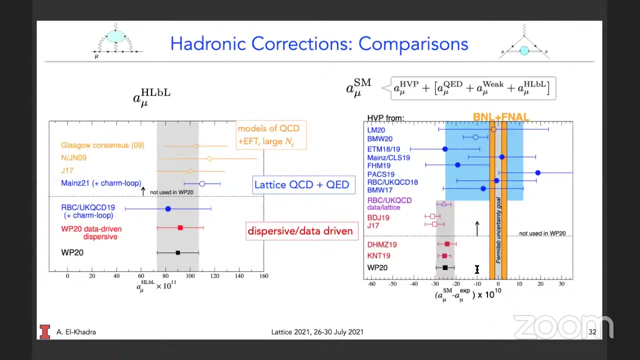 Go ahead please. Thank you for this nice talk, Aida. I have a question in your slide 32.. Okay, It seems there is a trend in lattice calculations to be higher than linear. And then the dispersive approach And, in agreement with the experiment, 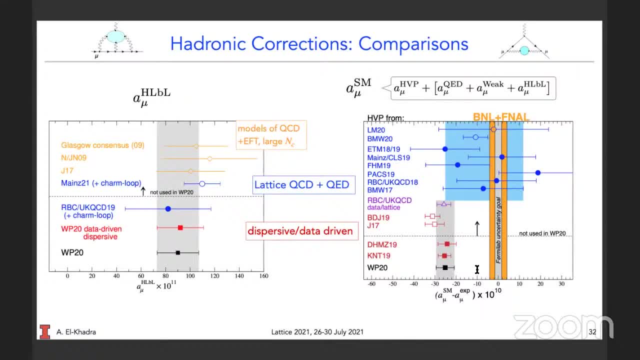 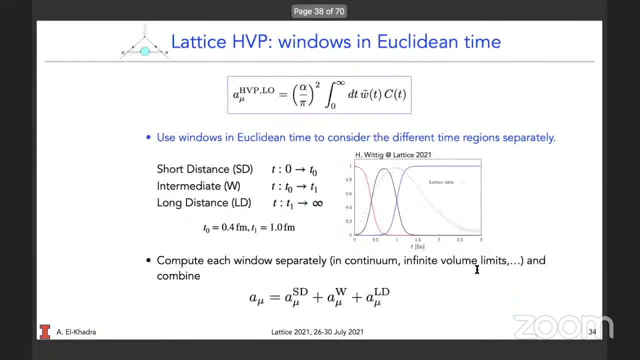 Assume that in the future this trend is confirmed by refined lattice calculations, Is there a way to establish where the difference between dispersive and lattice calculations could come, For instance by cutting the momentum transfer? Okay, In integration, So that you can compare different regions and discover? 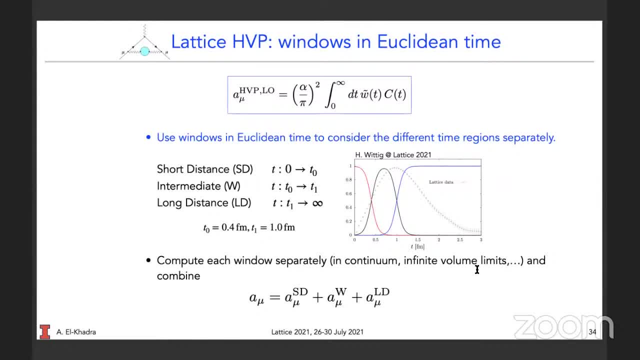 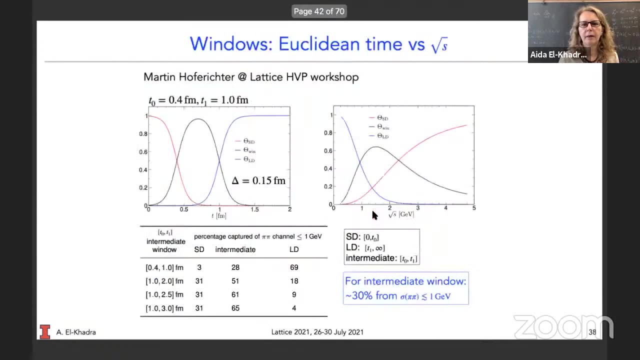 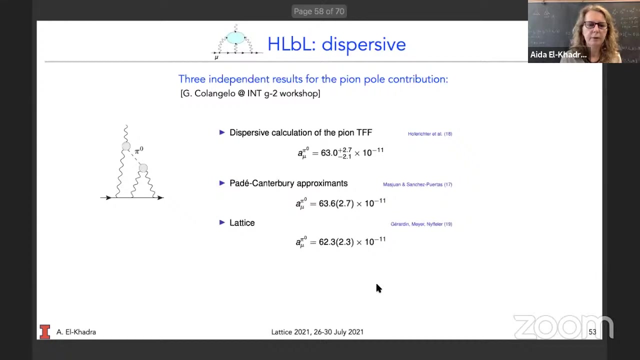 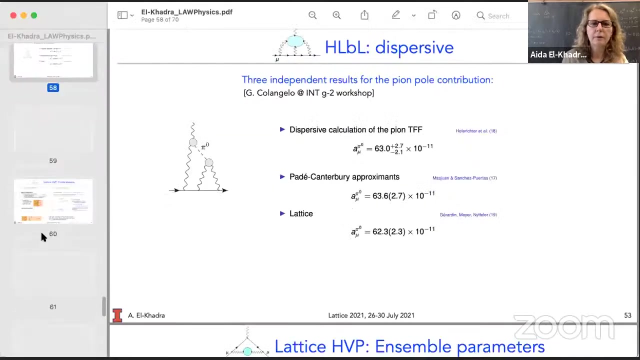 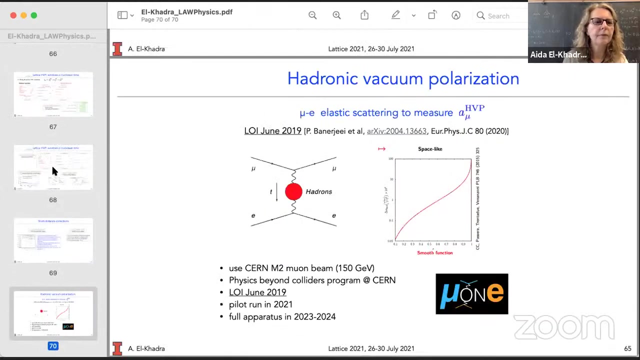 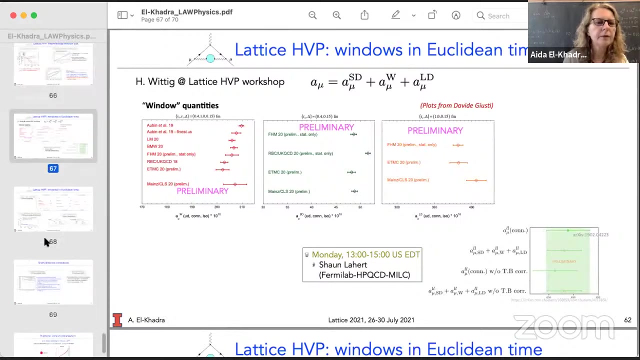 if there is a missing exclusive channel that is not included in the dispersive calculation. So let me answer that in several parts. I pointed out to you already these windows in Euclidean time And you can Let me see if I can. Actually, what I want is: 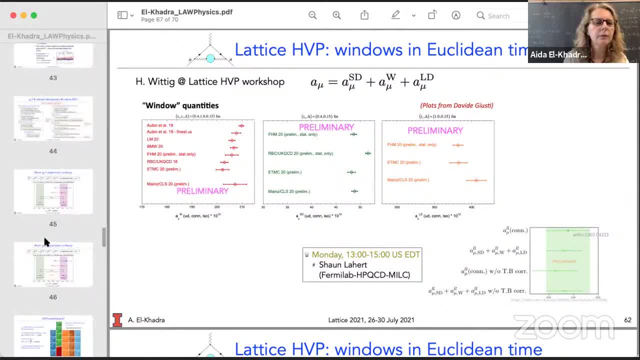 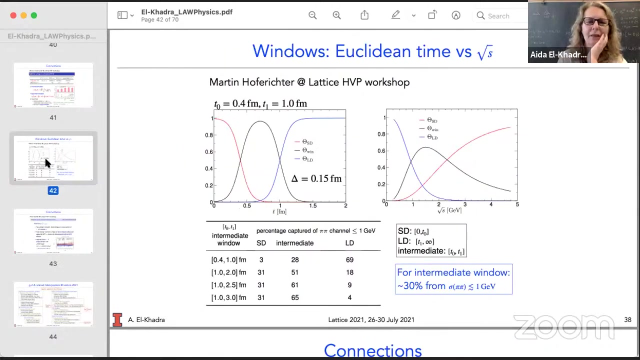 Okay, Okay, So I thought I had a. Okay, Then I need to just Describe it. Oh, here it is. Sorry, I thought it was in the appendix, but it was in the main talk. I skipped over this. 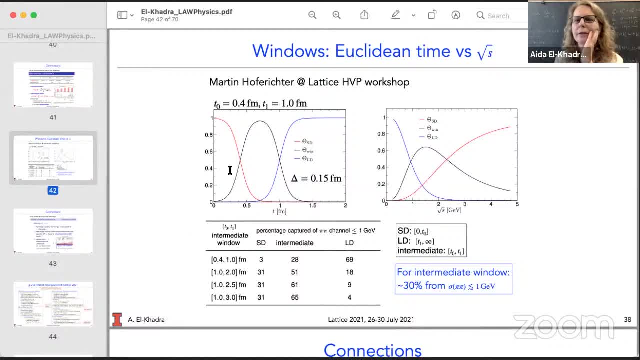 So here you see the windows in Euclidean time again, And You can now take a look at These windows in Euclidean time And bring them back. to Bring them back to root S Okay, Which is, you know, the, the data driven approach. 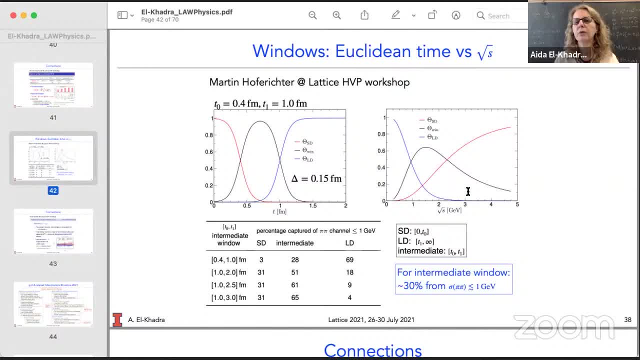 You see that of course there's not a one way, Of course there's not a one-to-one correspondence with exclusive channels Directly. But you know, there's some intermingling between, You know, between Euclidean time and and and S. 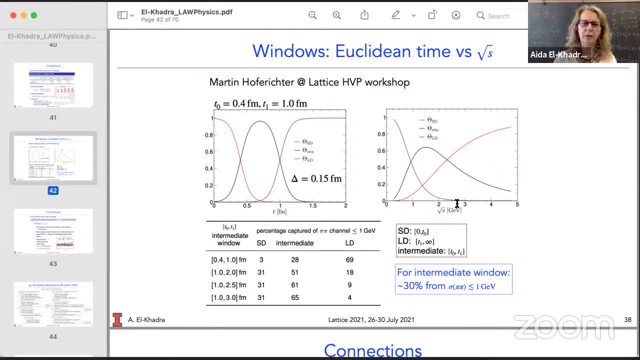 What you also know, probably what, what all of you probably realize, is that going Going from Euclidean space Into Minkowski space, you know, in this case would require a A Laplace transform, Which is difficult to do, but the other way around is fine. 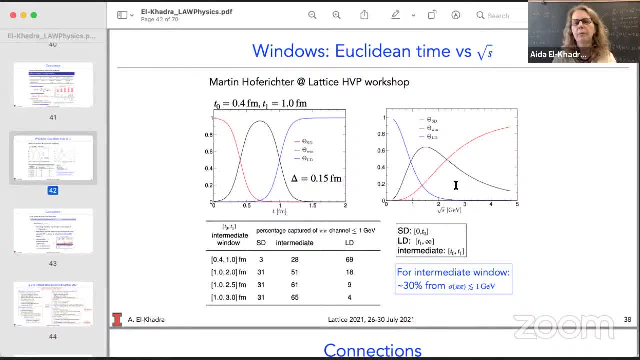 So we can take experimental data, Measured, the cross-section data, and we can very easily Turn them into Measurements of the individual windows, So measurements of windows that are constrained, You know, with these weight functions, And then you can look at. 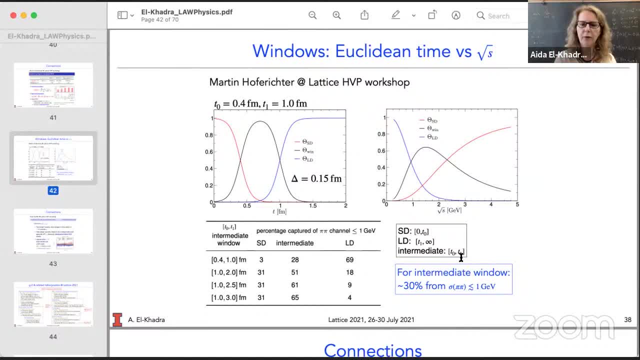 What the different windows that people had defined, What the what Channels contribute. And for the intermediate window, for example, the pipe high channel at less than a GV Contributes only about 30%. The long distance Window- here the blue window- would receive 70% of the contribution. 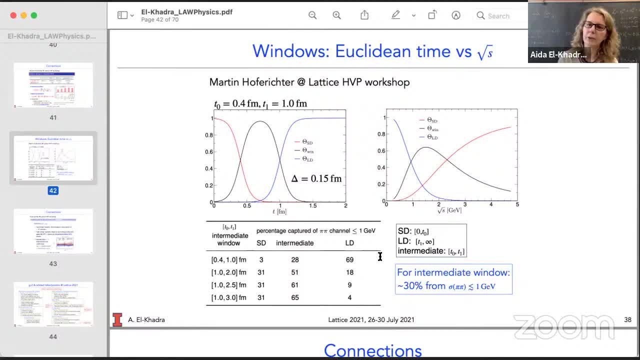 From the pipe high channel at low energies. So in this indirect way you can, by looking at Windows, and you can even look at, you know, smaller windows. If you want, you can Isolate the, The tensions in more detail. 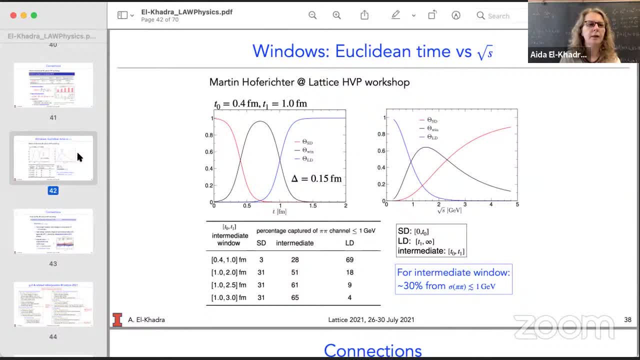 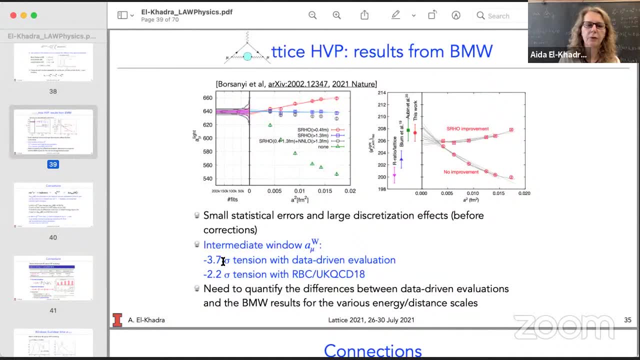 This has not really been done yet. You know, I showed you. I showed you this: This is the intermediate window and there's a four Sigma tension In the intermediate window between The BMW collaboration And what you would obtain from our ratios. 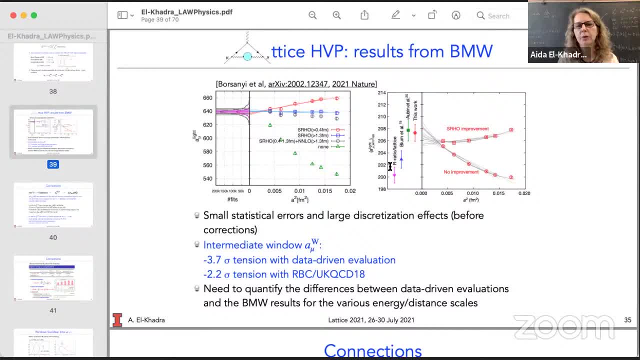 But there is another lattice computation That's perfectly compatible With the R ratio And intention with the BMW collaboration. So the in these windows Will allow us to perform more detailed crosschecks And actually seeing whether the different lattice computations agree with. 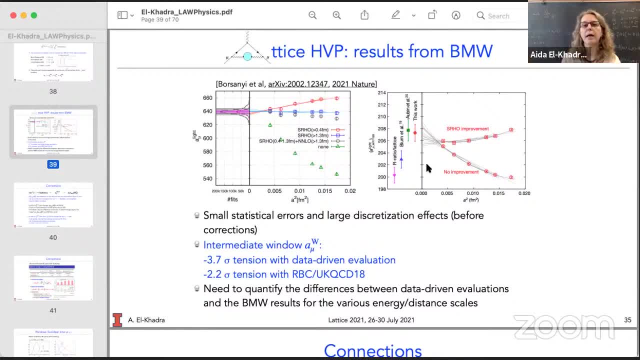 each other and each of the different windows And How the, which have Different systematic Errors And, if You know, the long distance window, say, the way it is treated by the BMW collaboration Gives rise to a bias, For example, 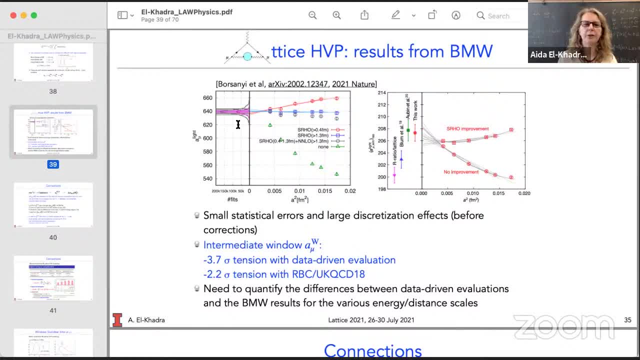 The reason why I say that is because The BMW collaborations result Requires A treatment where they first have to Correct The data for the dominant discretization effects That are not describable by a linear semantic EFT description. You know, extrapolating linear and a squared: 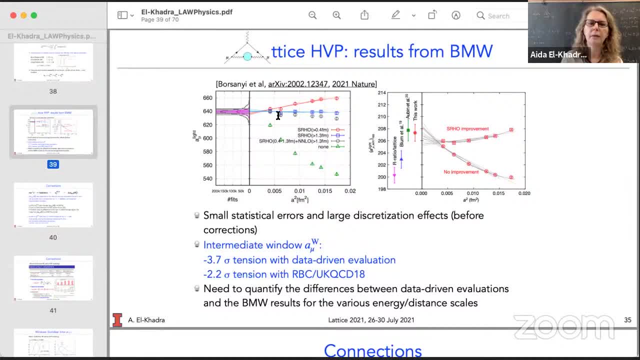 So they first correct the green points to obtain the Gray, blue and red points, And they really have to trust the correction procedure. They don't just extrapolate these results To the continuum limit because they believe that They have That. there are corrections here that are nonlinear and the lattice spacing. 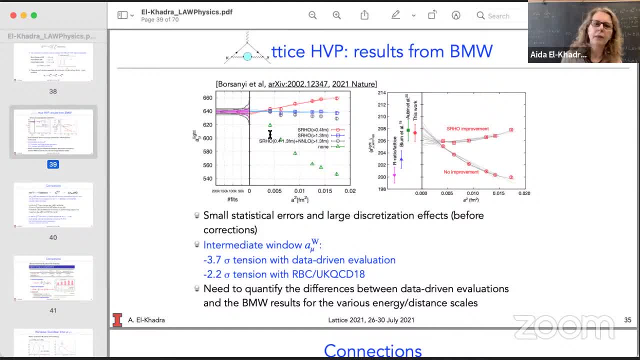 That are important, that are large. Okay, So the continuum limits Procedure by the BMW collaboration. You know they've tested this procedure. They believe that they are. you know what they're seeing is correct, But it is something that needs to be scrutinized with other. 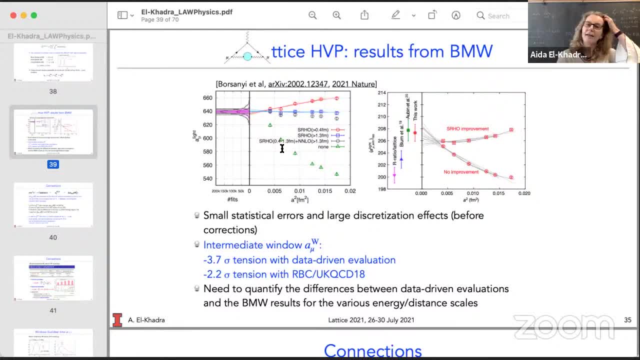 discretizations. Recall that different lattice actions Have different discretization effects. So at finite lattice spacing You know different results will be very different, but they all have to have the same continuum limit, So that continuum limit should be universal. So that's one question that we need to scrutinize. 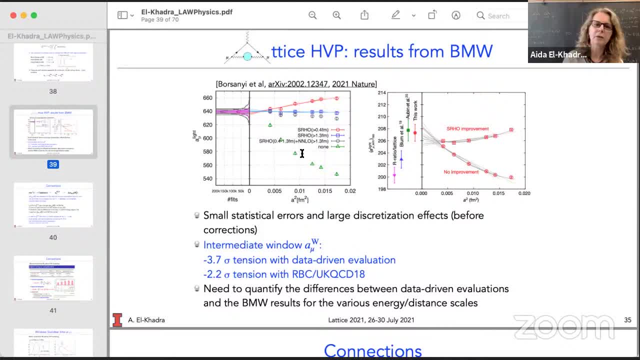 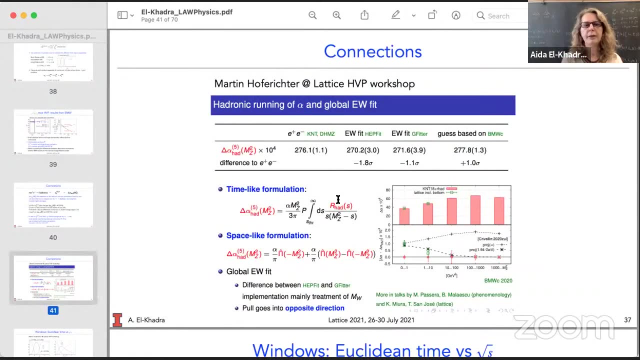 In very much in detail. in particular, this correction procedure would affect the long distance More than the short distance onto immediate distances. The reason- Another reason why I'm talking about this is because The interplay between Between electroweak fits and the adrenic vacuum polarization. 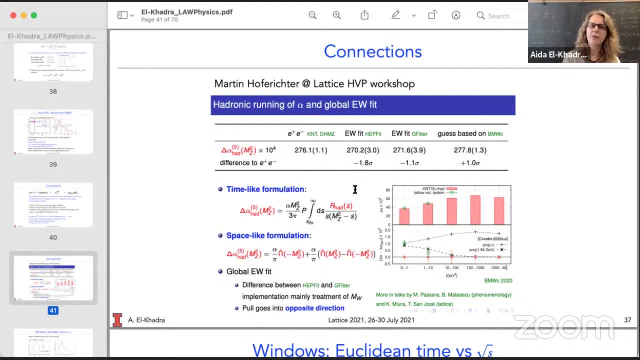 If you take the BMW collaborations result of HVP And just say that Their result is larger than data driven And that difference is evenly distributed over the energy, Overall energies- Then that gives you A large difference with electroweak fits. 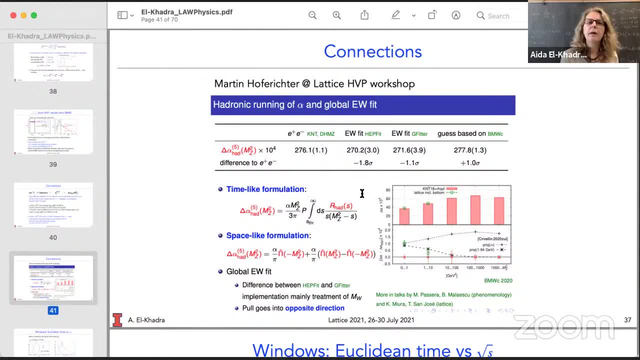 You get something close to four Sigma Electroweak fits, of course, have. The running of alpha has a different weight in it than HVP. The HVP, as I explained Is, Is weighted towards low energies, Whereas the running of alpha is weighted towards higher energies. 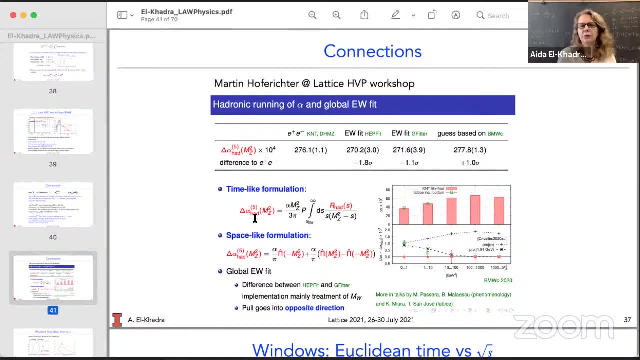 So if the HVP Difference comes from low energies Right Then, Then It can be hidden in the electroweak fits, but that's something that needs to be understood. Finally, what I also wanted to Show you is: 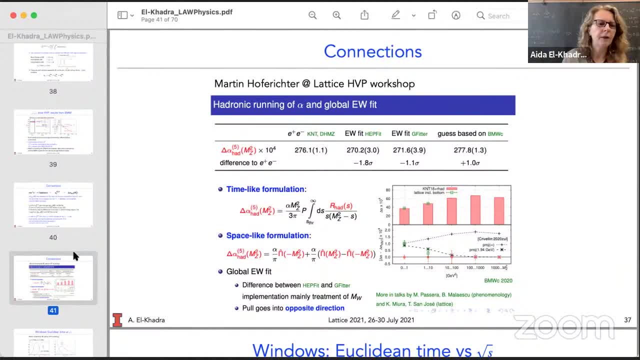 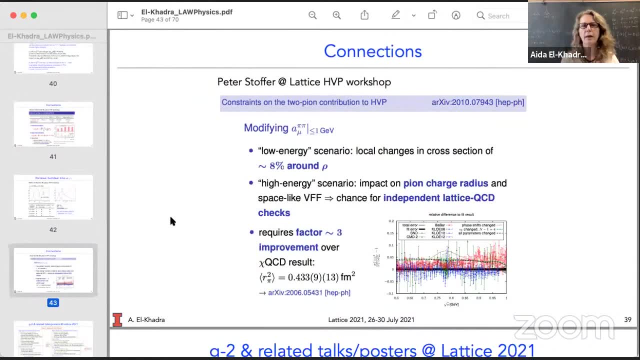 That One can take a look at. You know what changes do you need in the cross section In order to get Something larger in this One GV energy range. So So, So, So, So, So So. 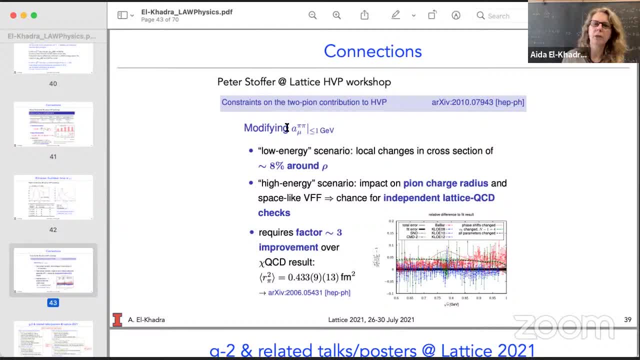 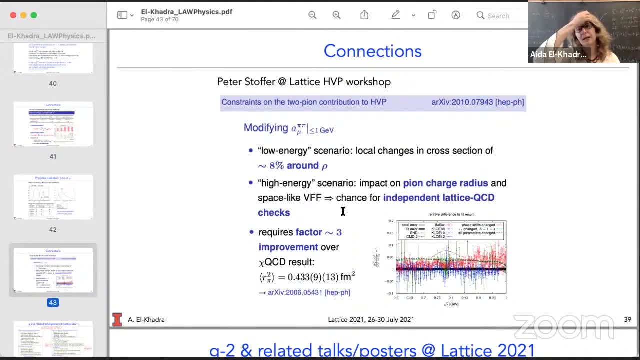 Atymentally measured class section In conflict with the implications from the lattice calculations. But there are further tests that one can do this for the lattice computations If needed. that one can do. It's too early for that because first we need to do those other están. 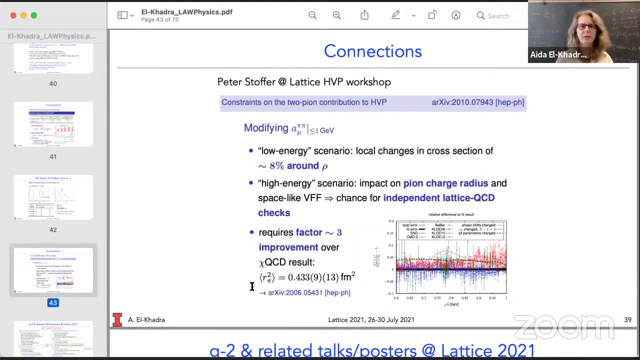 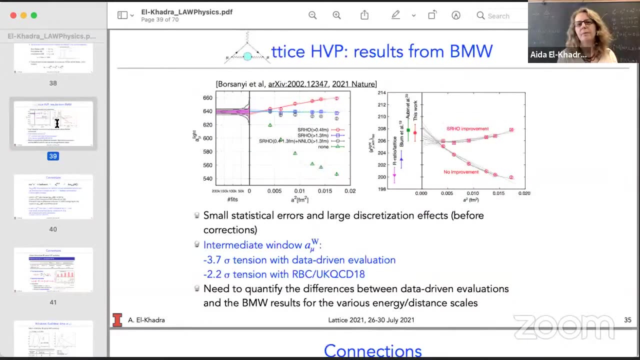 w представля la base de las etiquetas. Cross checks of the different windows, distances at long distances, at intermediate distances in Euclidean space, and also understand whether or not this tension that I showed you here for the intermediate window, you know, if the excess is in low energies, but the intermediate window only 30% of it. 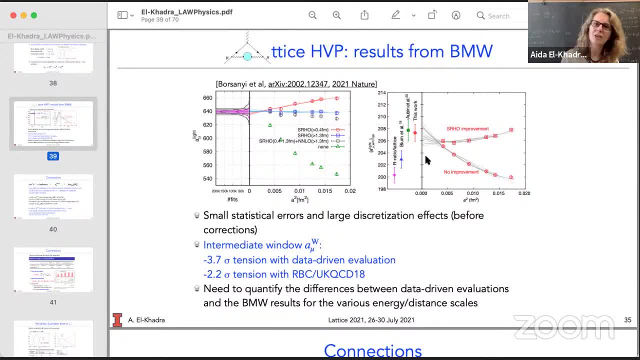 comes from low energies and there's a four sigma tension, then you know you would get a much larger tension at for the long distance window. So so there are ways in which we can understand these tensions better. Some of them are a little bit less direct, but they're certainly important. 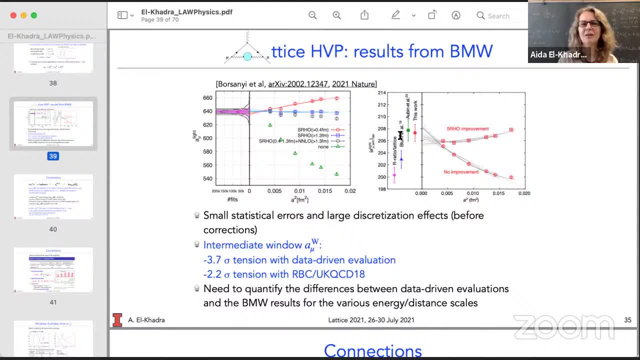 But first we need to resolve the tensions between the different lattice results. You know this is significant, this two sigma tension here. So I would say that, to answer the start of your question here, these errors for these, these groups, lattice calculations- these errors are real. 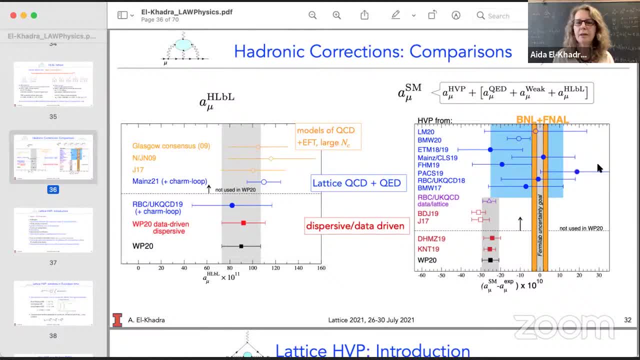 There are some that are large, with large errors. there are some that are low, that are actually the central values are much more compatible, But the overall errors are large. These errors are real right now Where a new lattice average centers, whether it centers here. 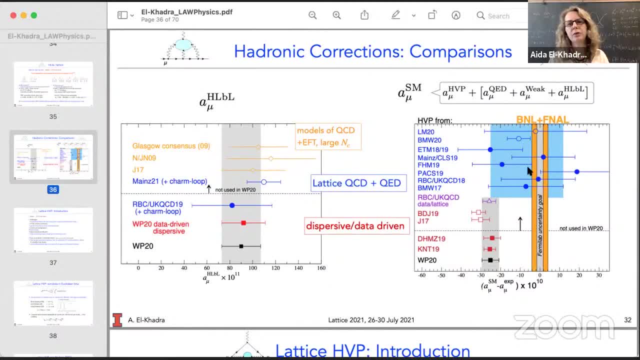 or here we really don't know yet It's really too soon to make a decision. So I would say that, through some understanding, that connection is really necessary for this flow To make two. I mean, that was a big if the statement that you gave. 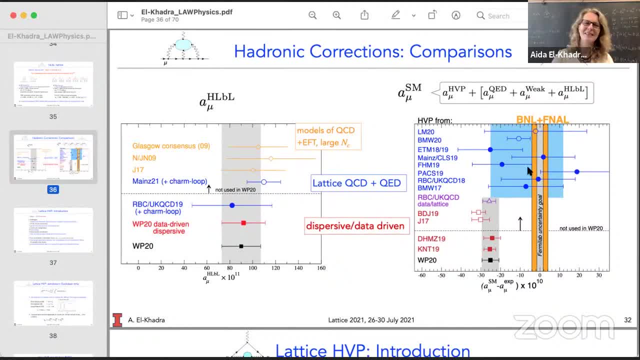 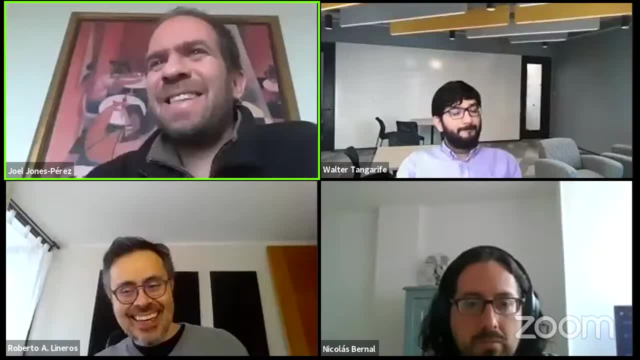 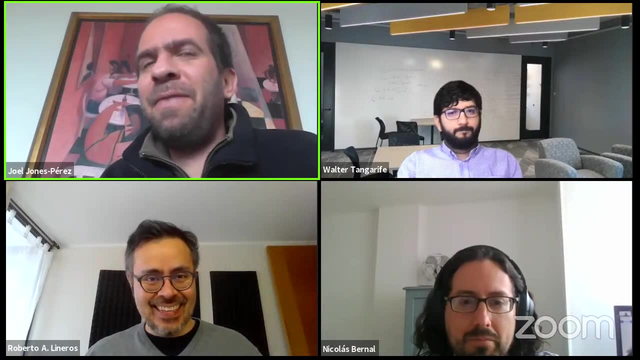 You know, if lattice results go there, in my mind that's a big, it's a thank you. Sorry, that's a long answer. No, not buzz very detailed, Thank you. Okay, Thank you very much. I have been told I have some audio issues, So I apologize in. 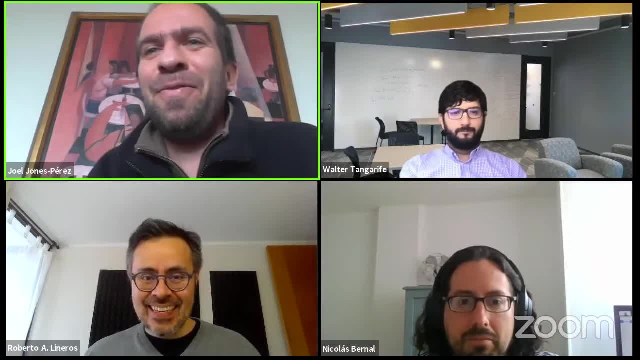 advance, in case we want to stop talking about audio. but while we're writing the battle to start, I'd like a few words from you, in case we're trying to solve them meanwhile, but hopefully they'll be okay. I think we've lost Aida. 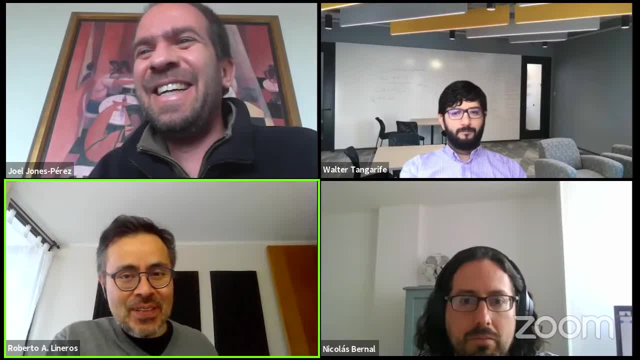 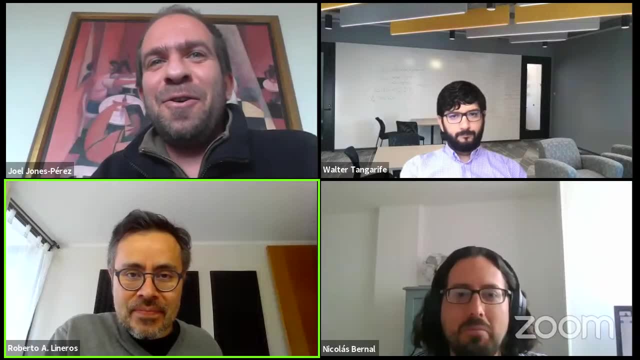 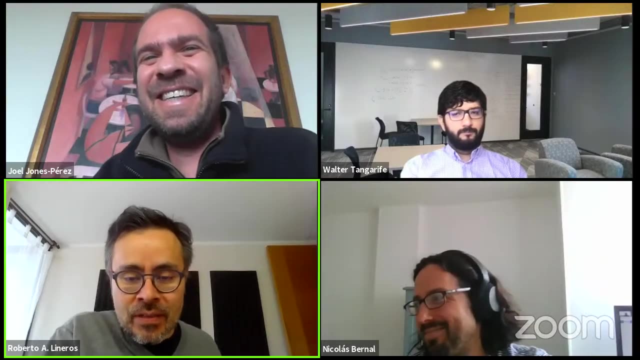 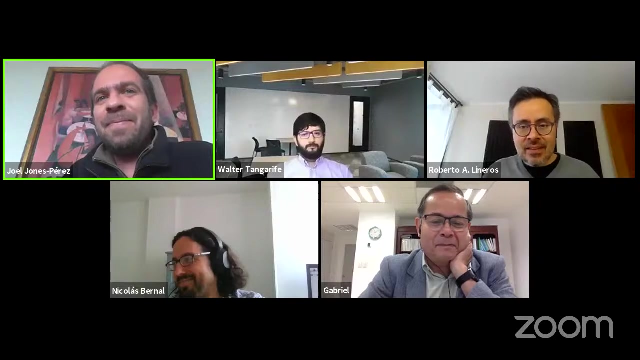 Yes, we've lost her. Let's wait for some minutes to reconnect. You can start your juggling act. Roberto, I don't have anything here, No, no, but maybe when she stopped the screen, share she, without wanting to leave the Hello Gabriel. 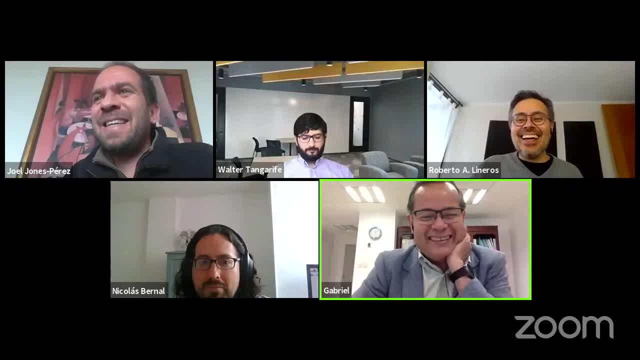 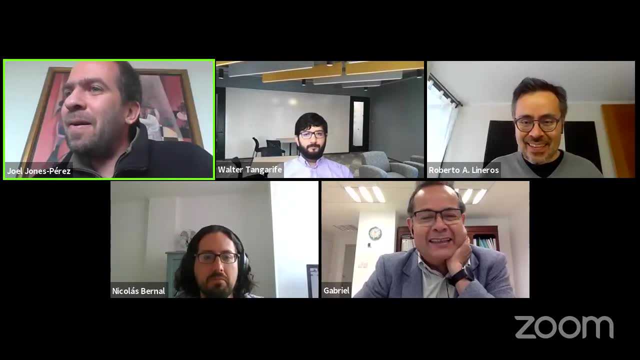 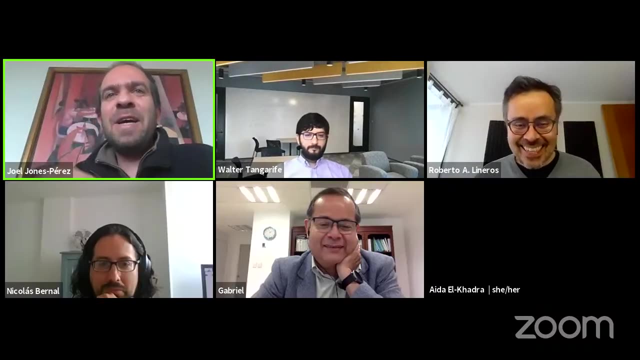 Hola, Roberto, Ah, hello, How are you? I'm fine And you? Yeah, here is Aida. Aida is connected, She's back. Can you guys hear me well now? Yeah, now we can hear you well. 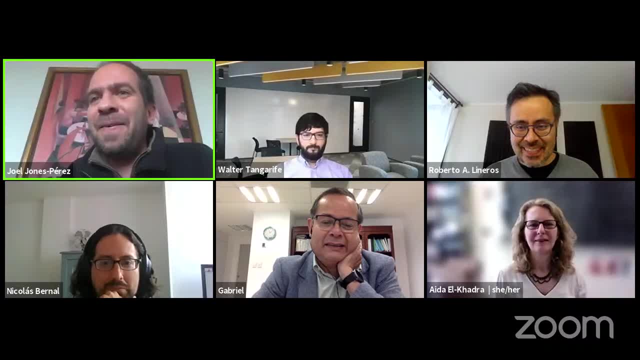 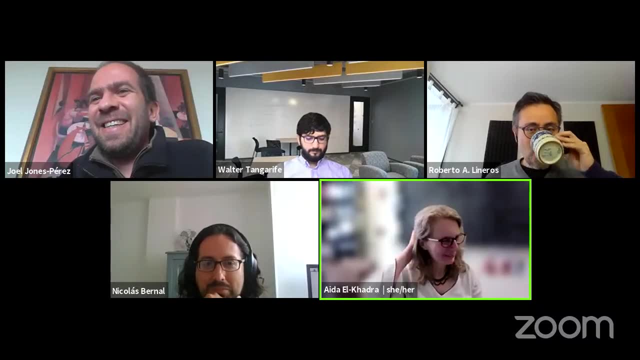 I closed a lot of things, so it should be working. Let's see. I'm very sorry. My laptop died. I wasn't paying attention to it, telling me it was out of juice, so now I'm on the other computer. I'm sorry. 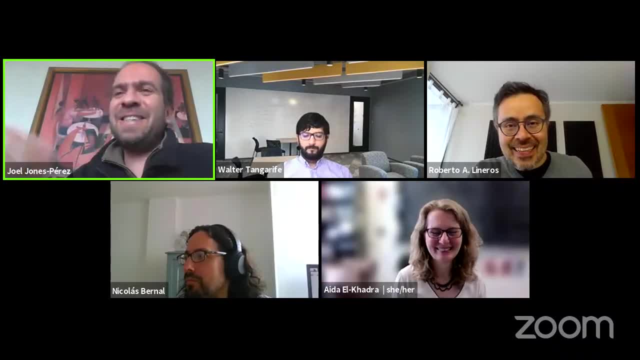 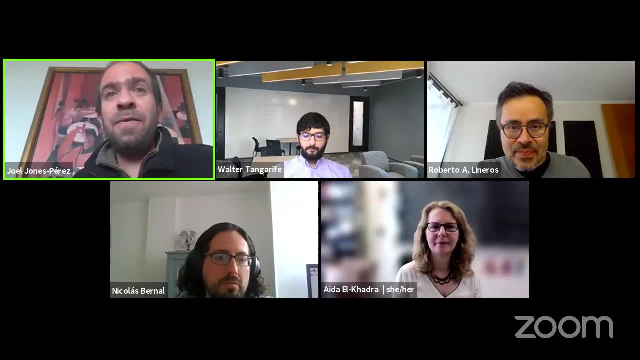 Don't worry. Don't worry, You just missed a thanking for the answer. Okay, Okay, So should we go on? I don't know if there's any more questions. There's a question in the YouTube channel. Do we also have a question, if I may? 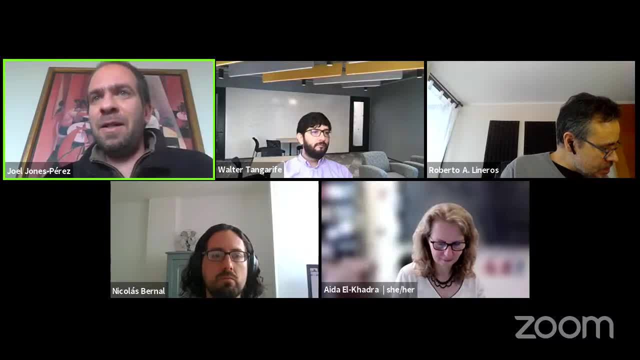 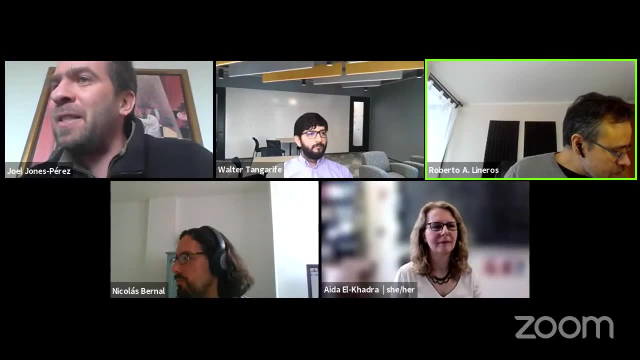 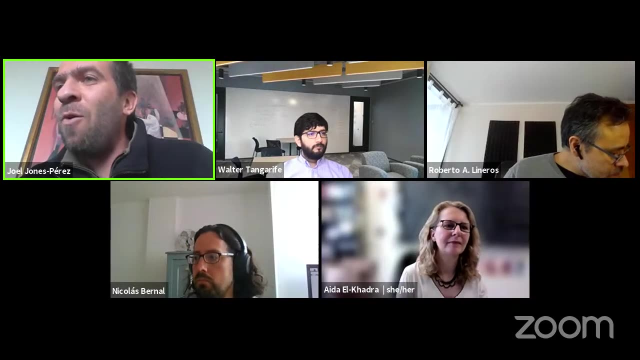 Right. So I noticed a question in YouTube, so okay, I'll pass it on. So the question comes from Carlos Antonio de Sousa Pires. Is it possible that this result comes down to the uncertainty in the hadronic calculation? Actually, how hard is it? 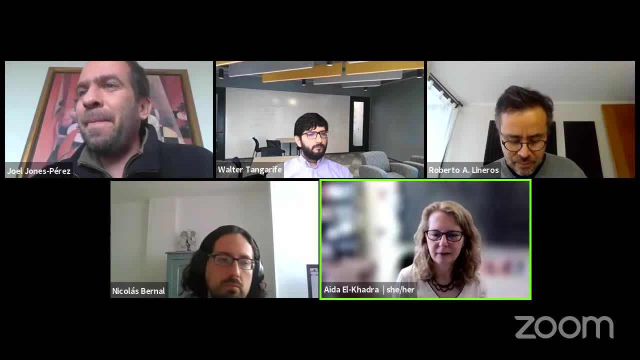 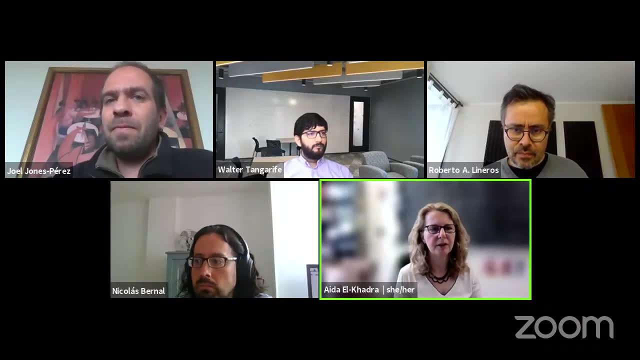 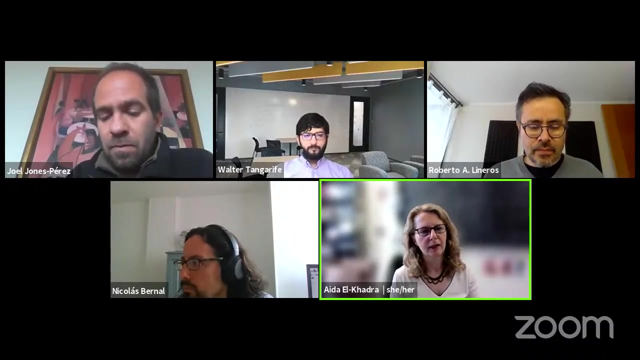 Yes, The uncertainty, the standard model prediction, is completely dominated. the uncertainty is completely dominated by our knowledge of the hadronic corrections. And what we're working towards is to have two independent methods that can address these hadronic uncertainties, hadronic corrections, in two completely 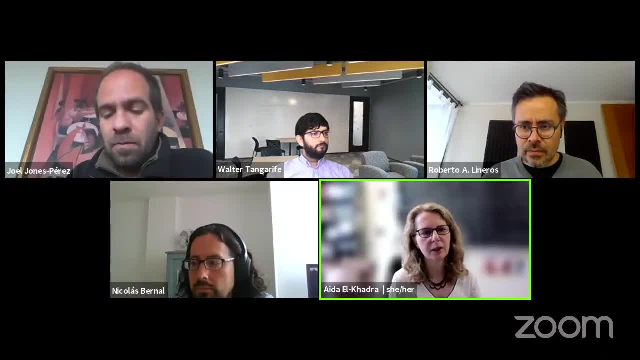 independent ways. Right now, as I showed, there are some puzzles. They don't completely agree. I would say that the data-driven method based on experimental measurements is really well established. The experimental measurements of the cross-sections have been performed Over decades. the method to turn the hadronic cross-sections into a hadronic HVP. 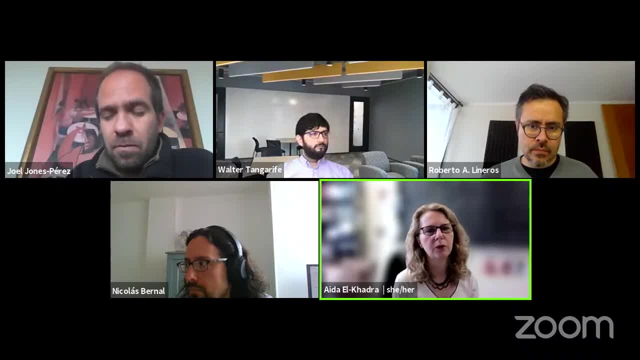 HVP estimate of the muon, some magnetic moment. those methods are pretty solid, They're, you know. there are some details like understanding, radiative corrections and so on, But all of that work has been done and And the methods themselves don't use models. 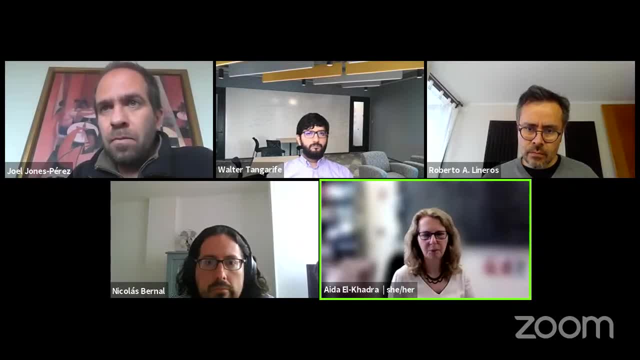 I mean you're just summing over the channels You don't have to describe. you know resonance, shapes and mixing between the rho and the omega, rho and photon. Nothing like that is needed because you're directly summing over all of the hydronic channels. 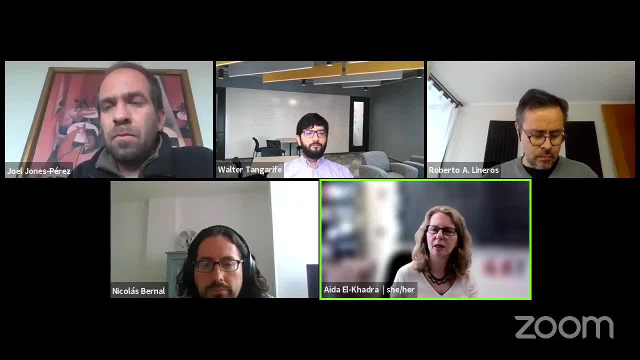 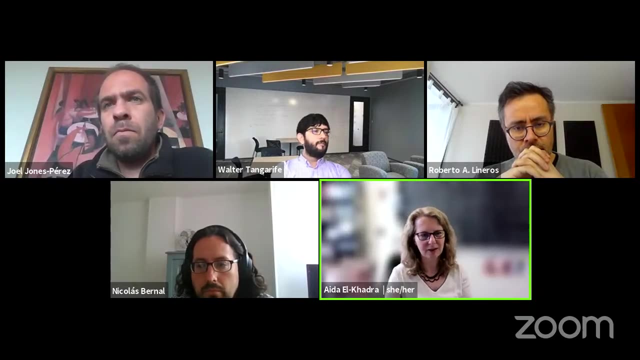 So the amount of theoretical assumptions that goes into the data-driven method is really very small, But it is entirely driven by how well can we measure those cross-sections. And you know, there are those annoying tensions, but those tensions are actually much smaller than the differences that I was talking about. 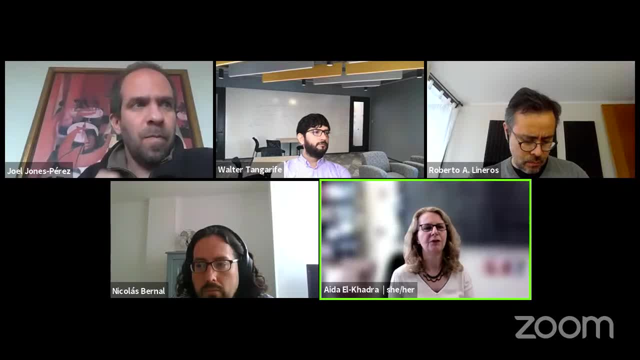 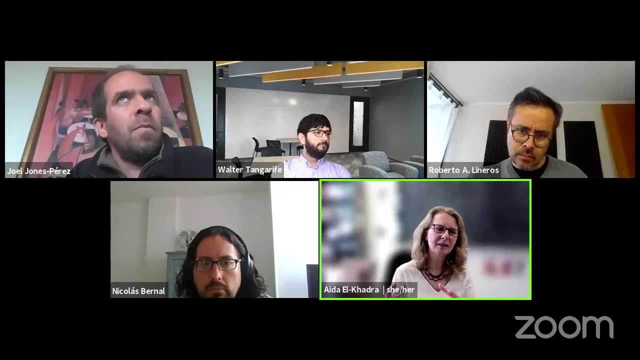 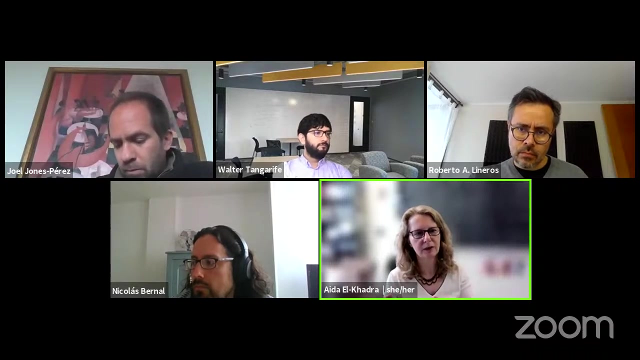 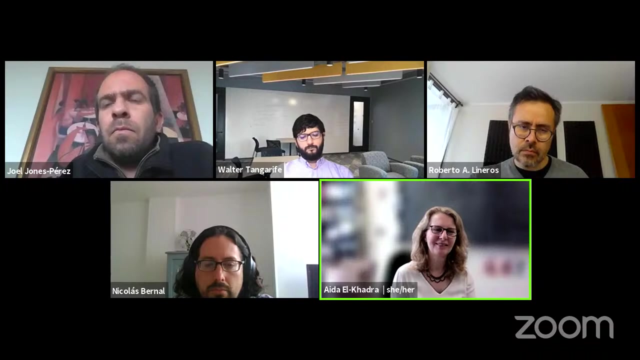 The lattice methods are still being refined. I would say We're still needing to understand, for this really complicated multi-scale object, that the hydronic vacuum polarization is that we need to know at points, And the key to this is that we need to know the 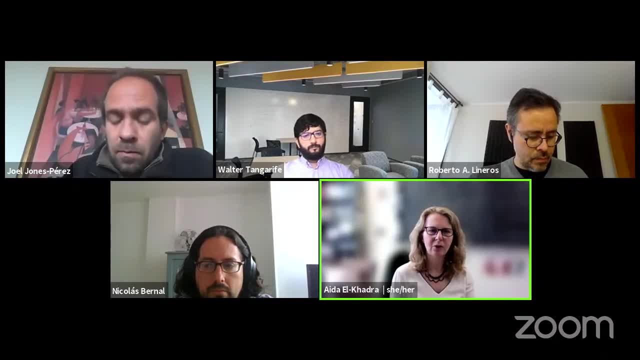 What I tried to show you is that you know our methods are being refined And we are really moving very, very fast towards a time when we can have method averages of the different lattice results and we can quantify how well the different extrapolations work and really get 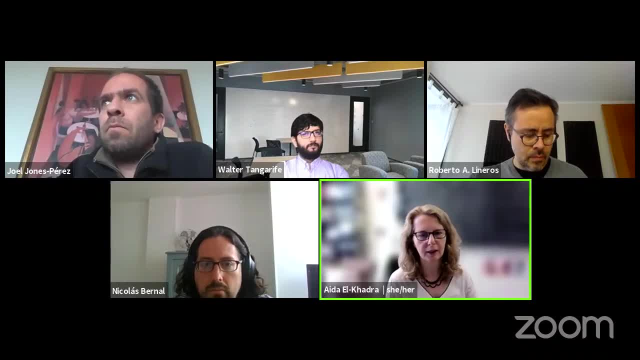 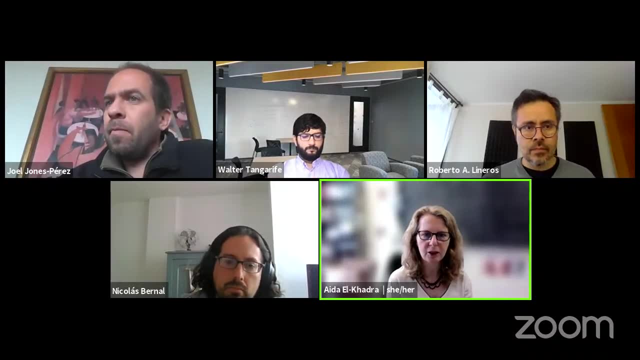 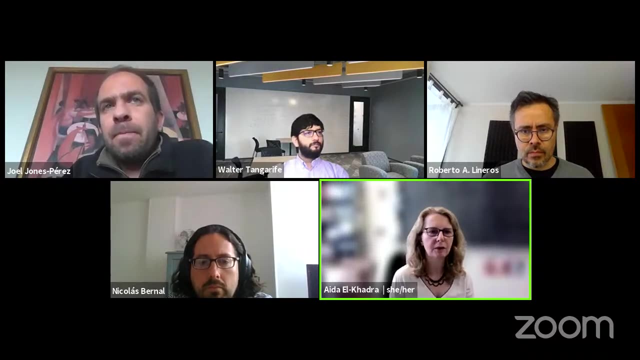 an understanding of the reliability of the underlying methods. So you know the BMW collaborations result. they did a serious computation, They used, they did what I said needed to be done with having many different ensembles, with having many different parameters. 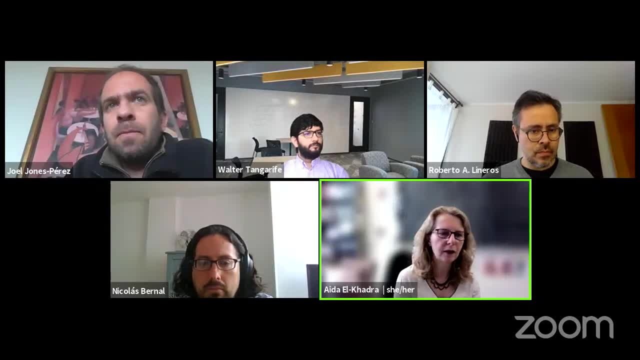 They did a very, very careful, impressive finite volume study. So you know it's a serious calculation, but it's really pushing, pushing the boundaries, And so it needs other other computations, using other discretizations, independent teams, and that is coming along. 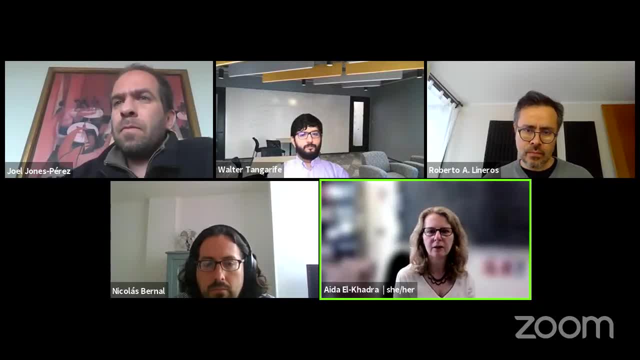 I think in a year, in in two years, we will have clarity and we will see if there's a tension between data-driven results and lattice results. It's too soon to say that. they will be Another long answer. I'm sorry. 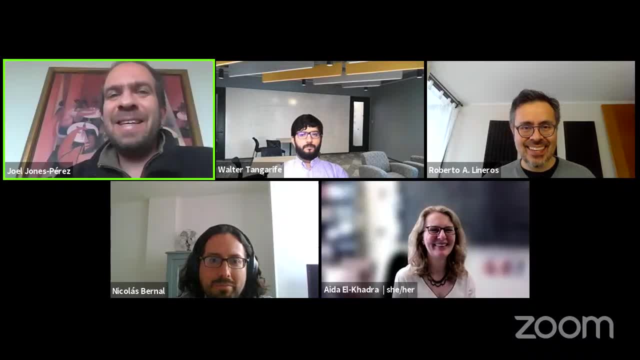 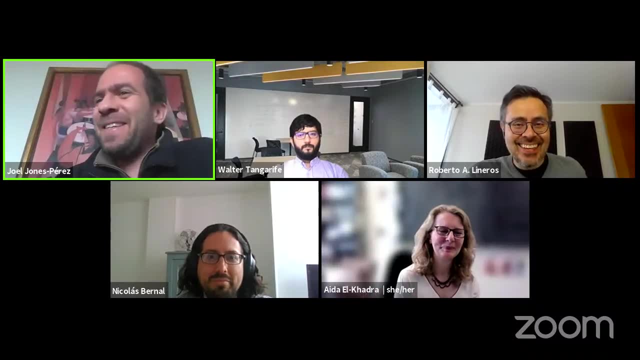 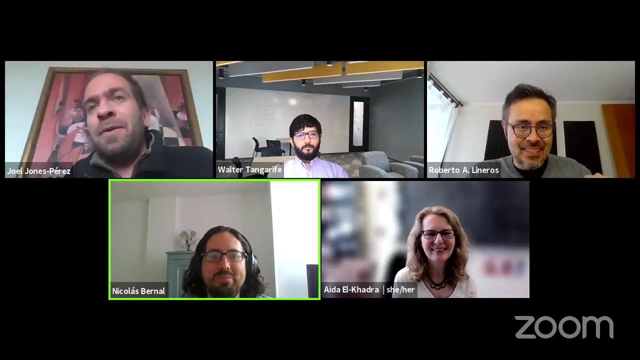 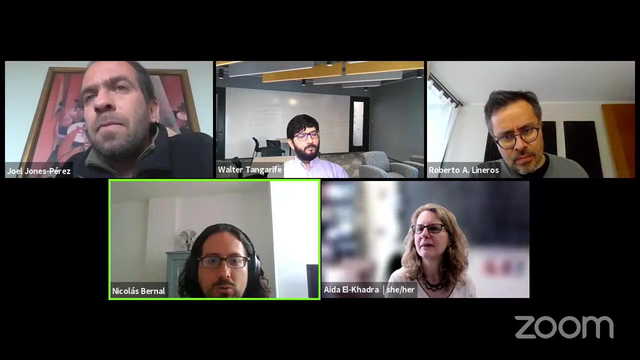 You are muted, Joel. Yes, sorry, Thanks, these mistakes anyway. um, so there's nothing else on youtube, so great. thank you very much, nicolas. please go on. okay. thanks for the nice talk. so just out of curiosity, if you take now this bmw result, what happened to the 4.2 tension? i mean going down to what do you know? 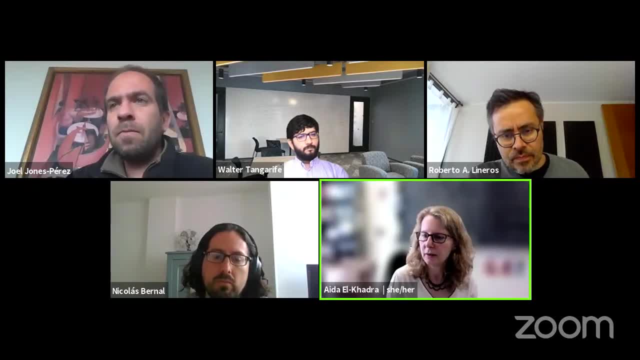 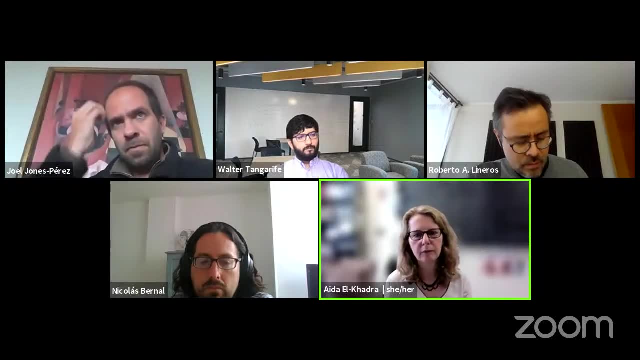 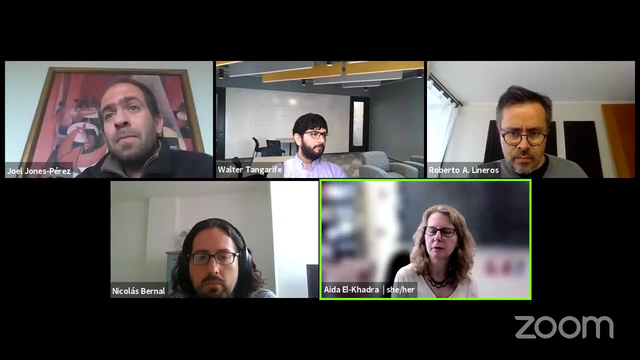 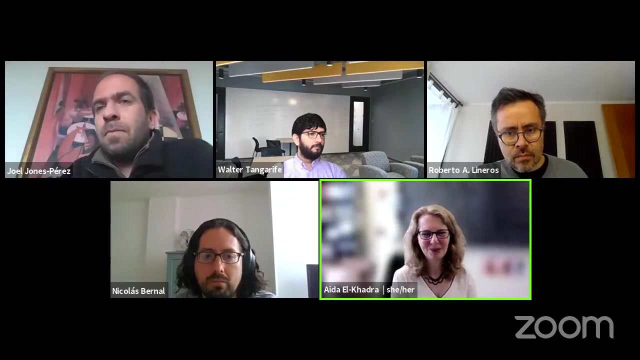 um. so if you take the bmw result as at face value and so replace the white paper um with the bmw result, it's 1.6 sigma tension with the experimental measurement, which is not something which is not really attention right. 1.6 sigma, you say, is. 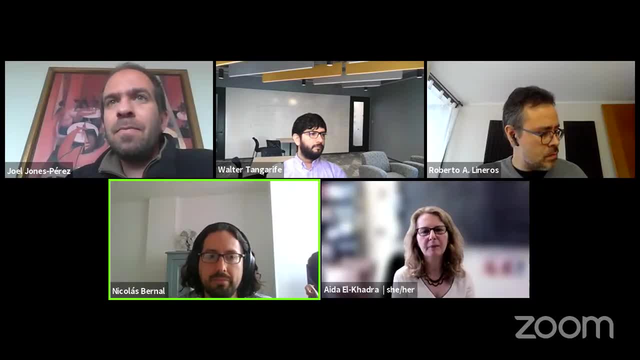 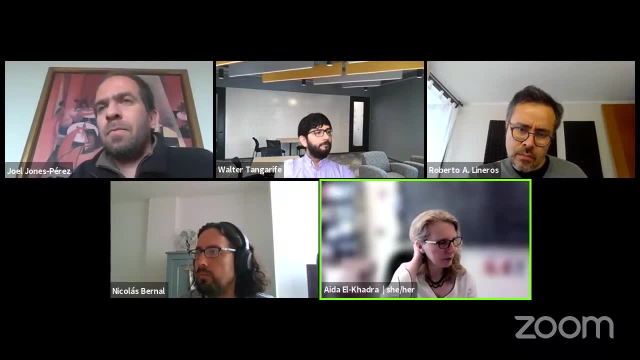 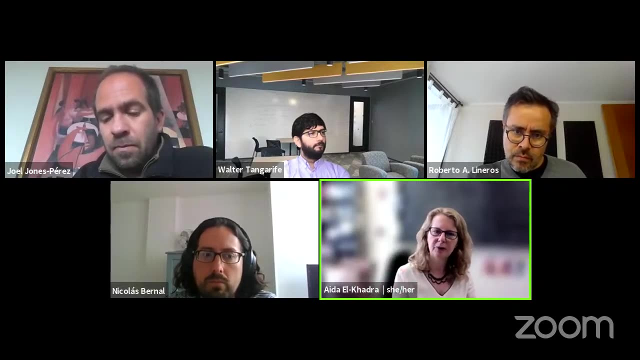 compatible, okay, um, but uh, the um, and and the difference between, because they are right in the middle, the difference between the bmw result and the data driven result is a little bit more than two sigma, which you can also say well compatible, but if you go into the scale, dependent quantities, as i discussed you, 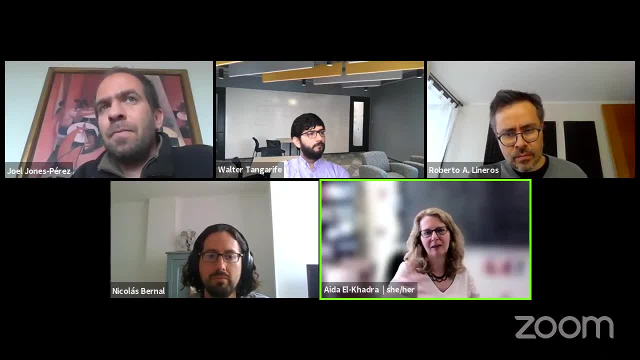 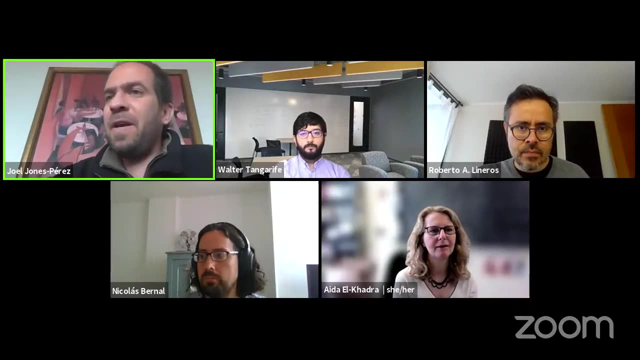 have this four sigma tension. that's now not so different between, you know, between experiment and and theory. i mean, it's an. you know you can play these numbers games. great thanks, um so on, via, via youtube. carlos antonio is also thanking you for your previous. 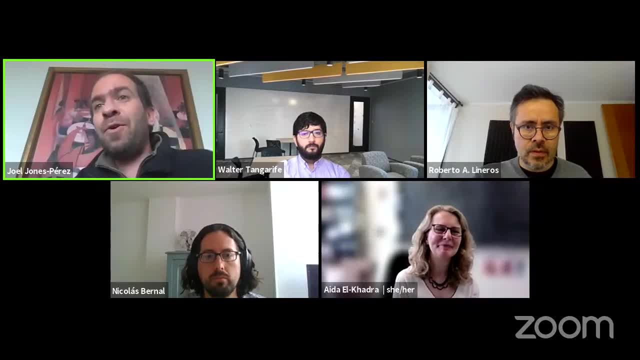 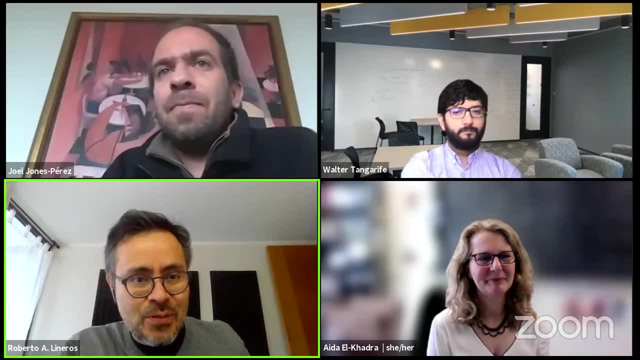 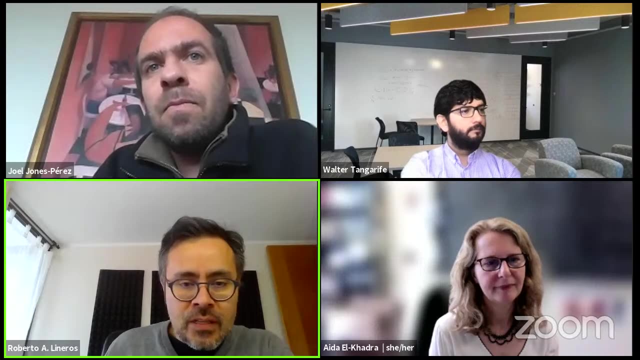 answer um more questions from the from the audience. roberta i, i have a question. first of all, thank you very much for the for the talk. that was super interesting. so one question i was wondering: is the because for people that is looking for bsm- i mean theories or whatever- this uncertainty and 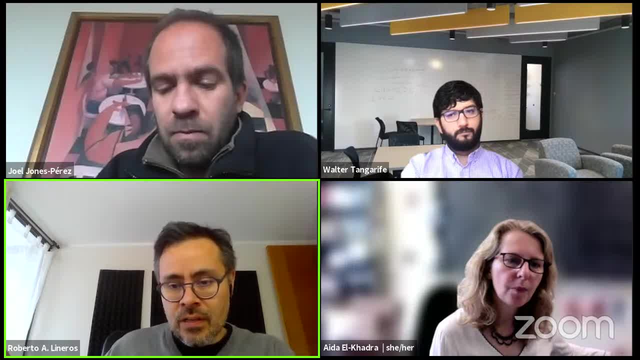 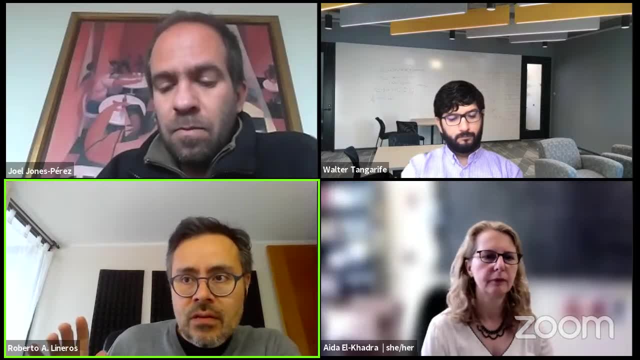 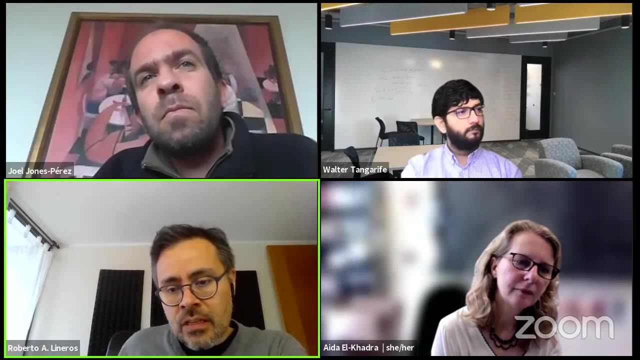 the, the most important to to set up the scale of the new physics, if there is a new physics explaining the, the, the g minus two. so more or less for the point of the experimental side we could wait for for, reduce the uncertainties because one one part is the part of qcd and that 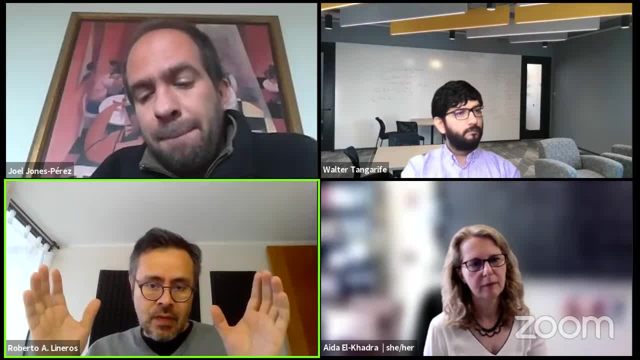 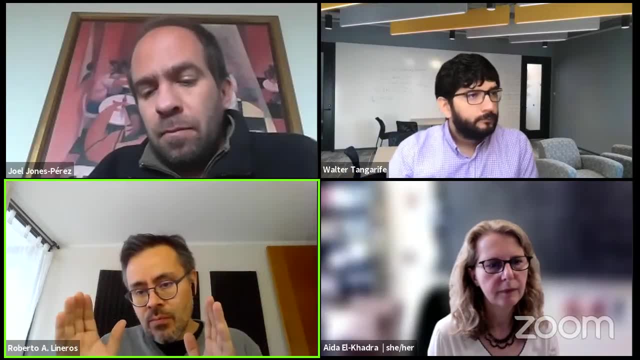 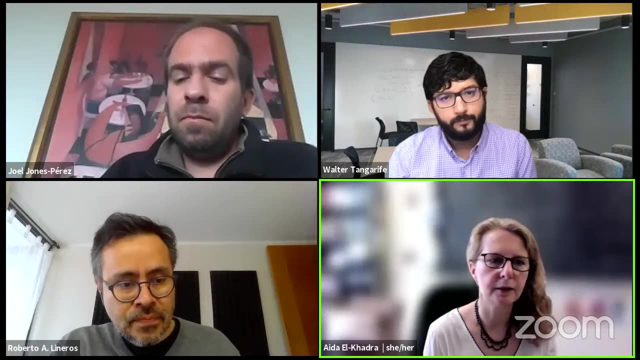 is. that is very important. but, as you said, uh, also with the question of nicolas, if the you have 1.6 sigma in the, in the worst scenario, but you reduce the experimental uncertainties, maybe right. right. so the analysis, the analysis of the family lab experiments, so they already have. 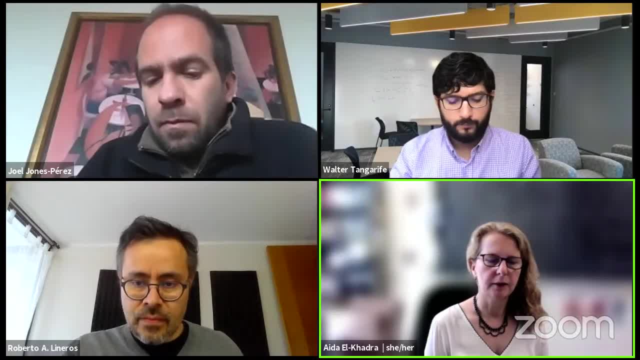 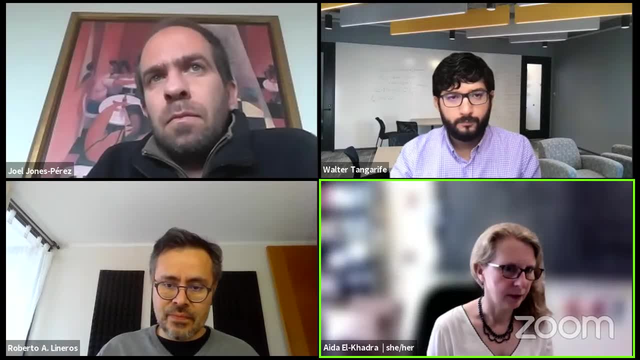 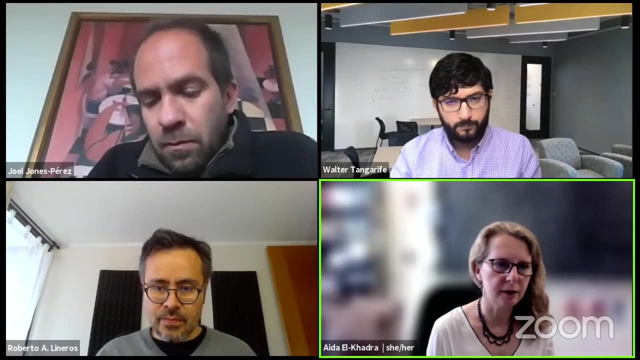 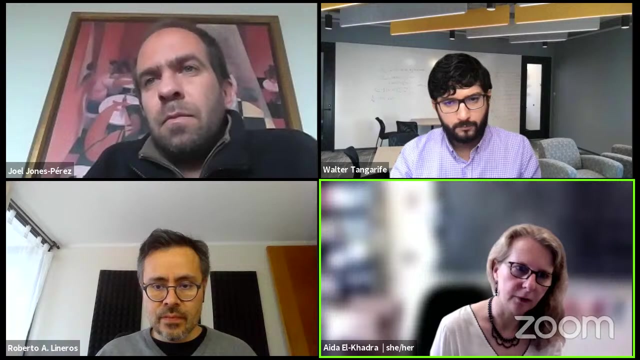 data from run two and run three and um, those data are, i think, like twice in terms of statistics. you know we might expect something like uh uh, twice the statistics, maybe even three times, and so they're analyzing those data right now. so you might expect a reduction by a factor of one and 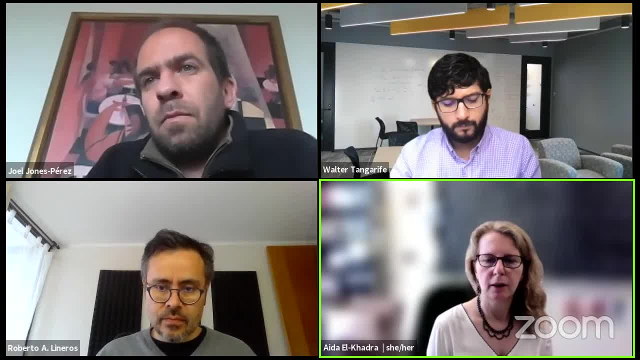 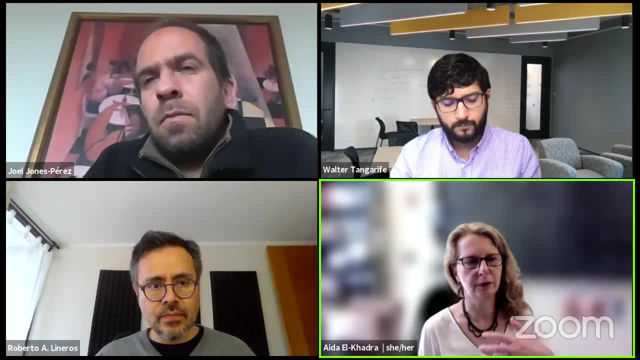 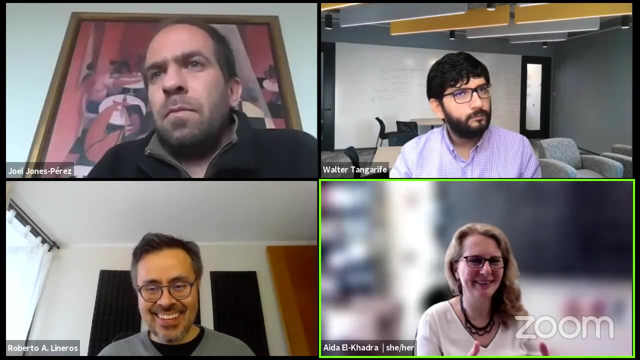 or a little bit more compared to now, uh, in about a year's time, next year, uh, and then you know they will the following year, roughly speaking. i mean you know it could be earlier next year. it could be that, because they've been known to be very careful and they 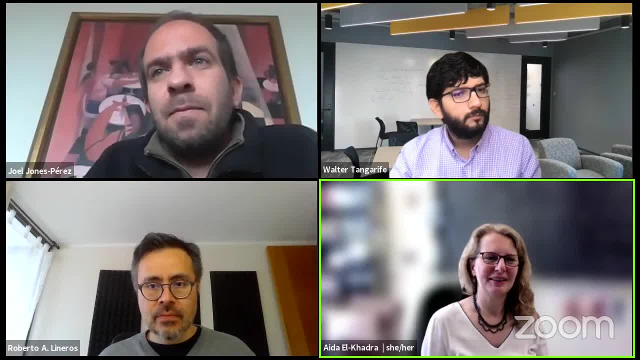 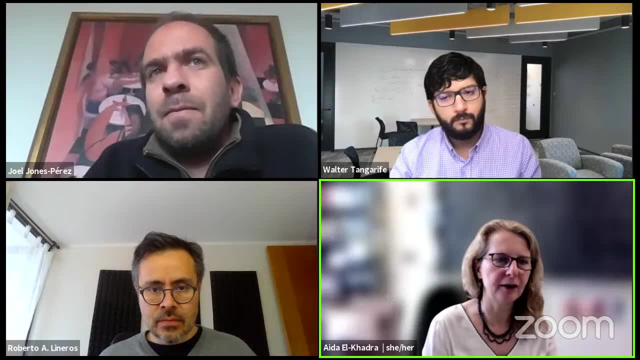 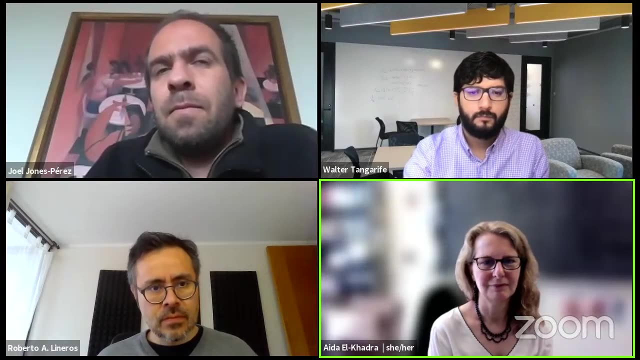 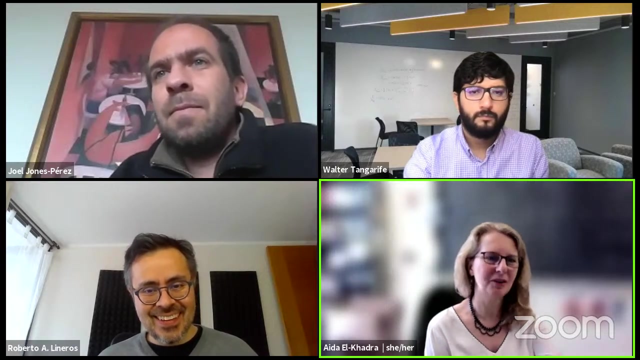 they are done, when they're done, which is what they should do. uh, you know, so it may be a little bit later, but the data already there. so i expect to have something like a factor of four reduction in the overall uncertainty. say 2025 very soon. and you know, in between it'll be, you know, in a year's time, two years time. 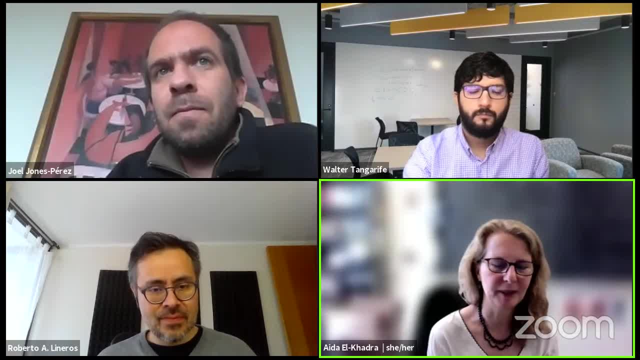 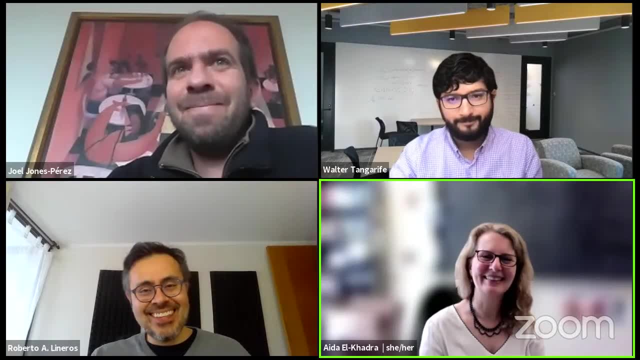 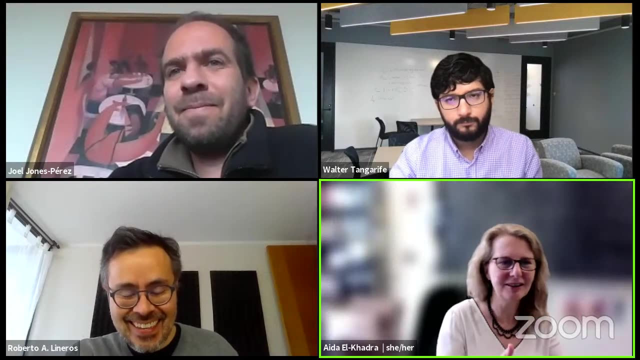 factor of two, factor of three, etc. that's my expectation. so we're gonna have a lot of news from the yeah yeah and of course we'll have to see where the central value goes right. you might have noticed that the central value went down a little bit. you know, we'll see. i mean completely, you know. 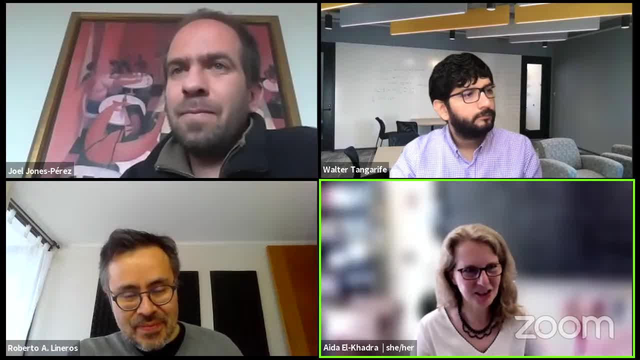 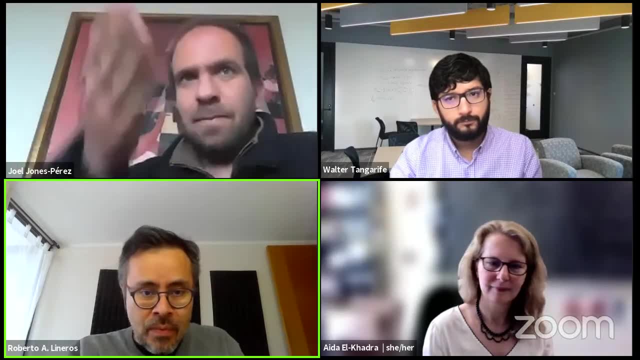 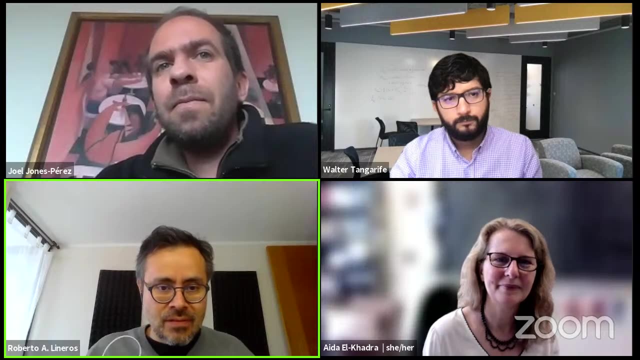 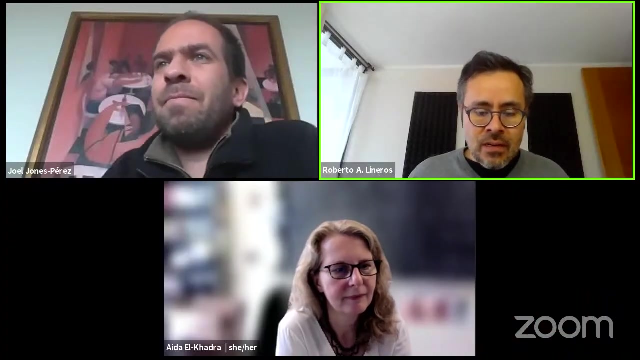 completely compatible, of course, but things can change within errors, yes. so another question, if i may. i'm not, i think i really want to ask something, because he unmute himself or i don't know. anyway, just by curiosity, because this part with lattice qcd, which is the main, 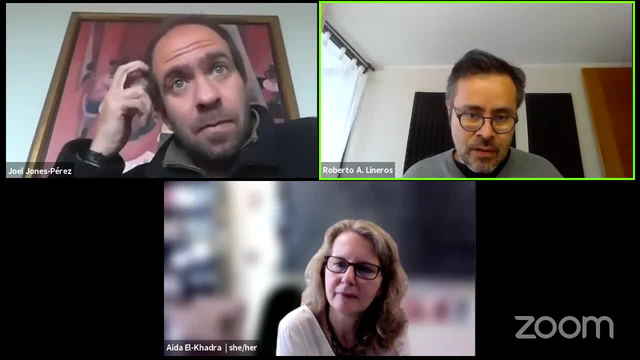 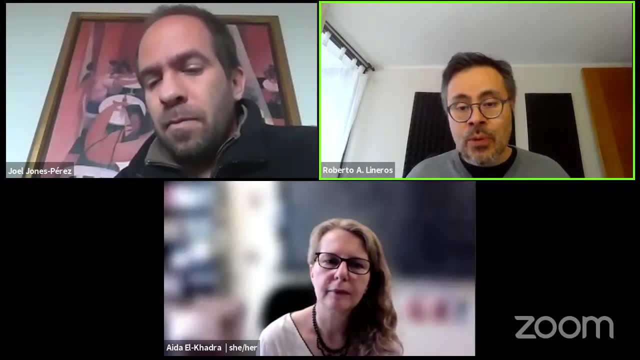 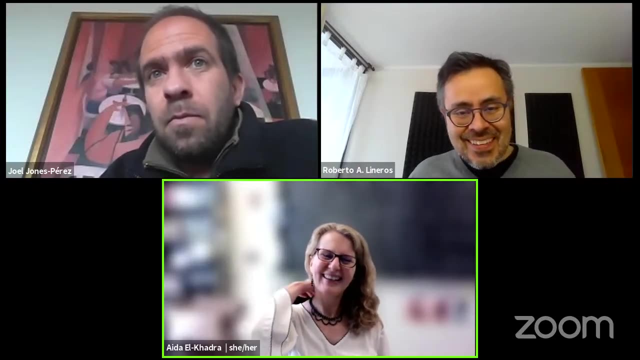 let's say, problem with the, with the lattice qcd is the kind of you need the refinement of the techniques for the qcd or it's just. you know, not just, but is the computational complexity of the to to make the calculation i mean right, or both? i don't know. so, um, for, 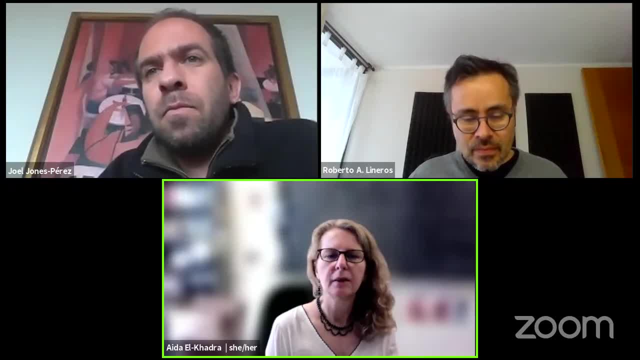 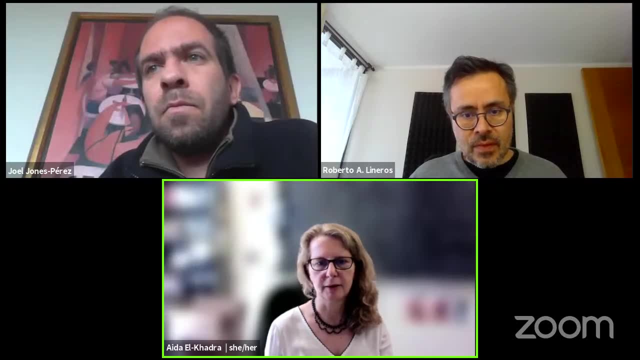 yeah, so i ask two questions, um, and so we'll go over the, the, you know, one more question and then, after downtown, uh, first question. but for me is that: how do you fish? because the 때문에 problem is often mach時候, no matter how advanced it is creating. 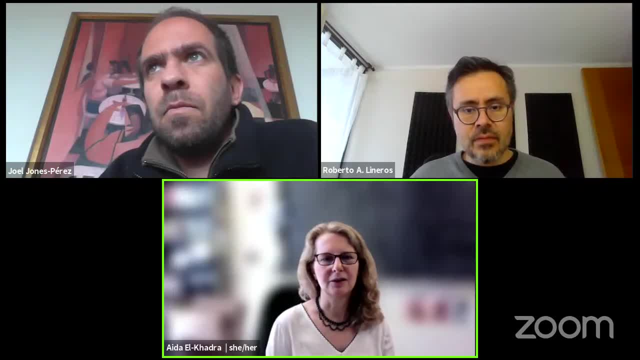 a simple design and of course this бо is a problem in their future. podéis 한국에서 luxury factory op wieder? 1510 men Day 80: 00 a 40% Outagem. the BMW collaboration was able to obtain the precision they did, to put it in technical terms: 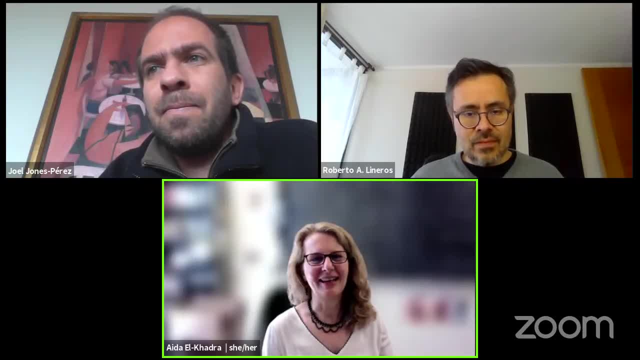 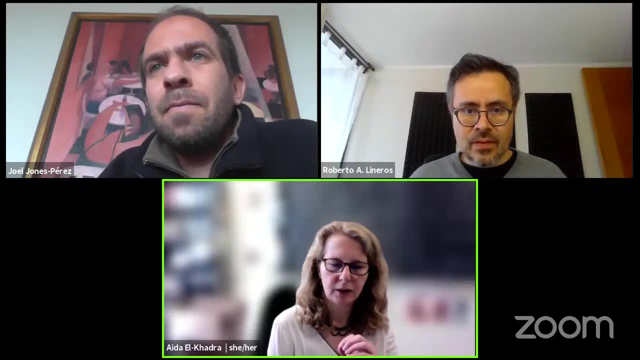 is because they clobbered it. You know they, they had, they used a lot of computational power. I mean they also, you know, did a good job. So you know that's one answer, but the other answer is: 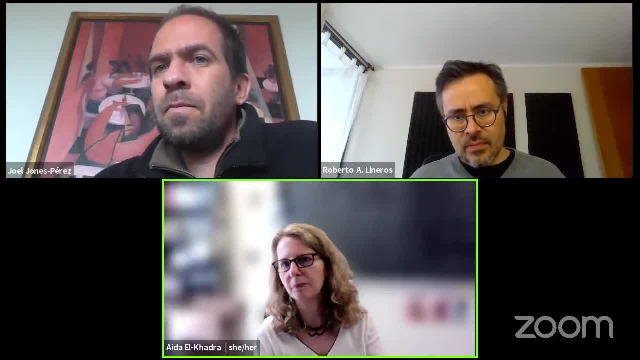 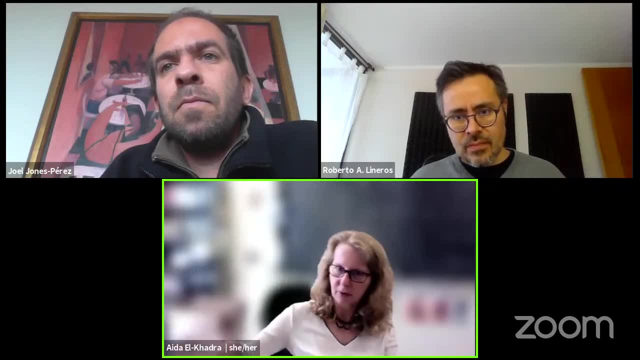 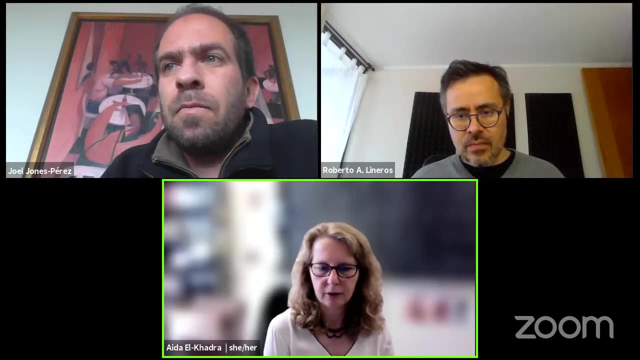 if you look at, say, the intermediate window, the statistic, you know you can actually do that with much less computational power because you know then you don't carry it. care about the large errors in the in the time and large times, And I mean it's pretty remarkable the difference. 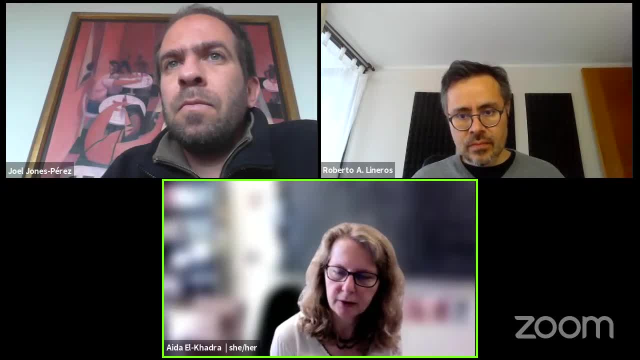 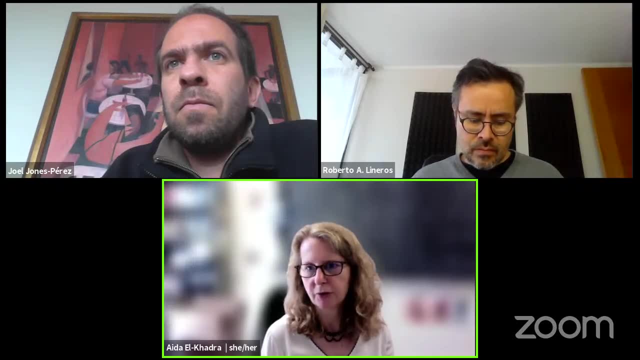 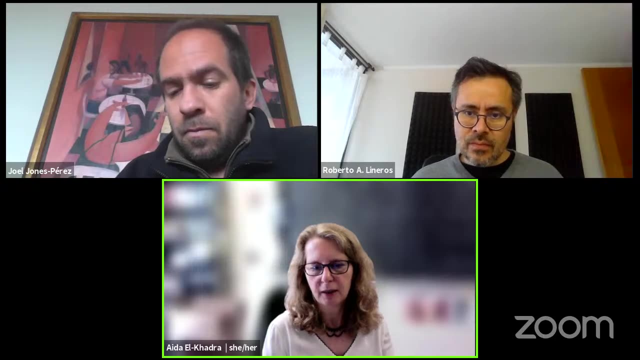 So. but now we, in order to get to the precision we really do need to also understand the continuum limit extrapolation. So this is kind of back to bread and butter. here we're talking about, as I said, a quantity that has, you know, that is sensitive to many. 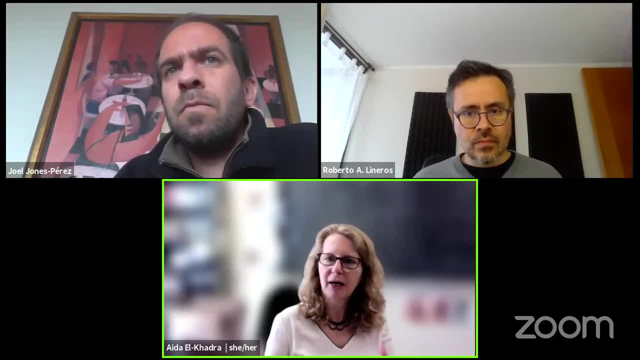 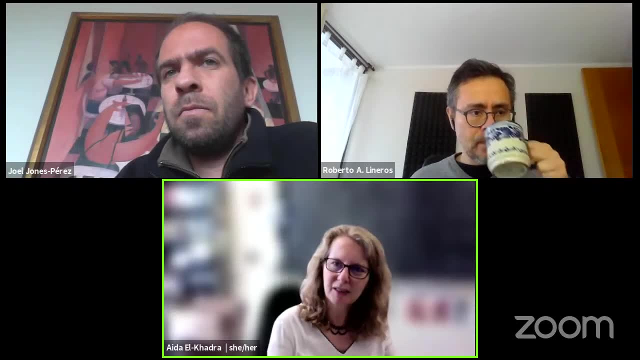 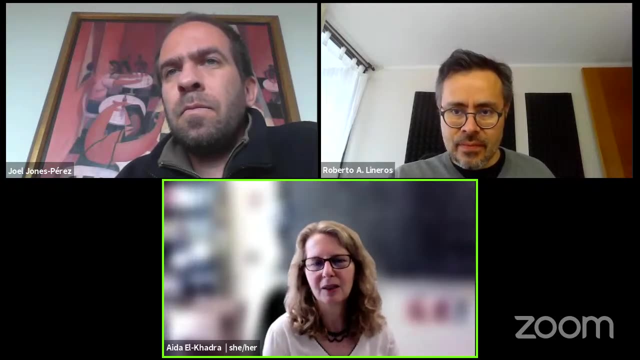 different physics scales. When we talk about a pion, and you know pion, decay, constant the scales, it's much simpler. It's a stable meson and you know it's lambda, QCD, and you know figuring out the. you know I mean the semantic. EFT tells you that discretization errors are. 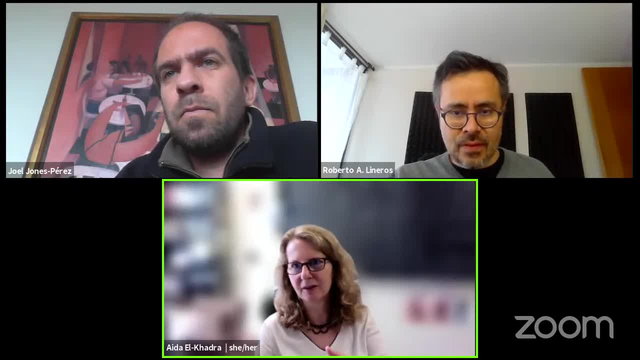 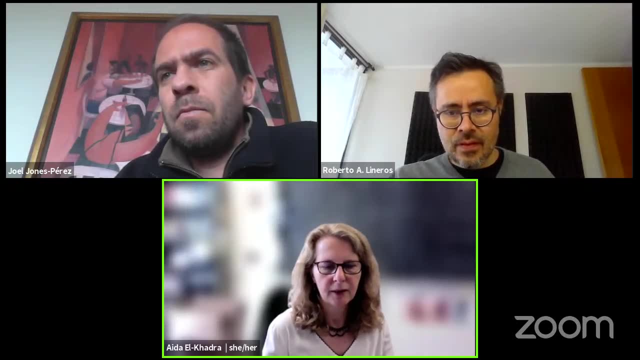 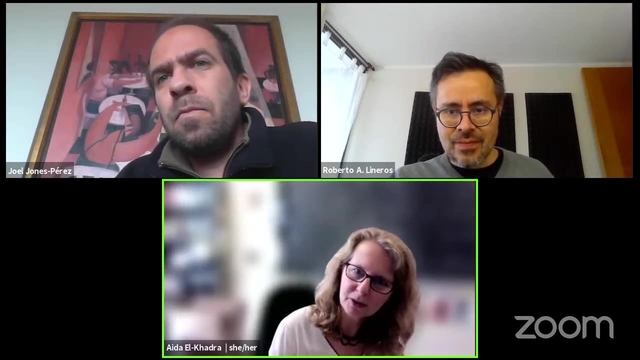 are powers, of lattice spacing times, of element physics scale. So life is simpler there And I think that all of these methods work, certainly work for this case. It's just when you, when you push on the precision, then you also. you know, precision makes things harder. 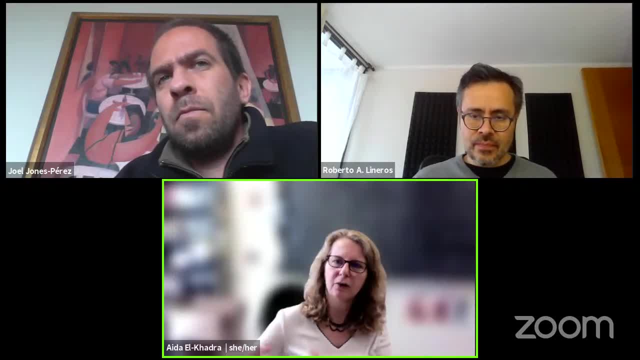 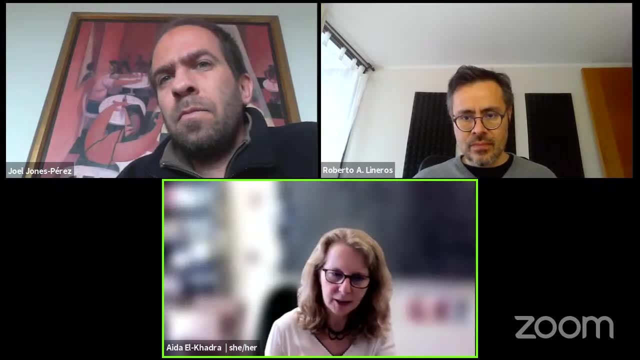 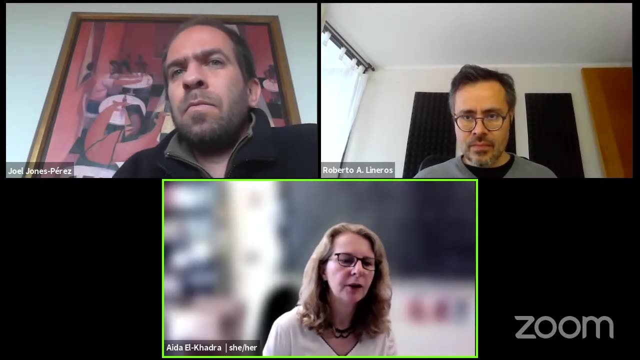 So now you have to understand higher order discretization effects. You know in more detail and really you know, do you have? you might have you know from from off-shell contributions which you have here? you would have not just. 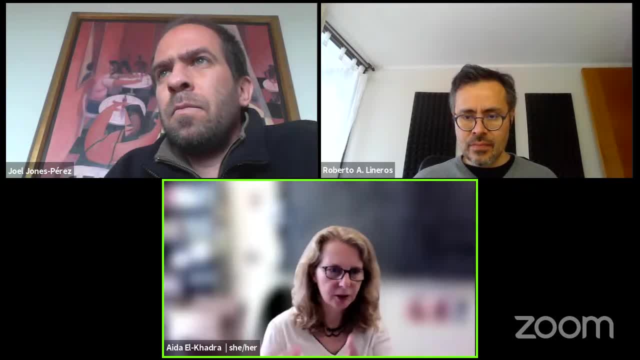 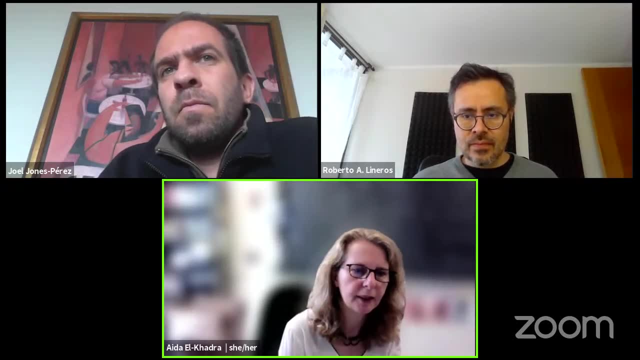 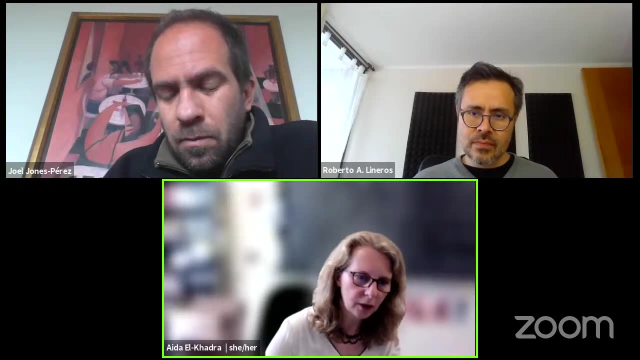 not just a squared and not just the power law, but you would also have terms that you know would be logarithmic and lattice spacing, and can you resolve them. So it's a matter of increasing the the precision to really include all of the different variations at the, at the needed. 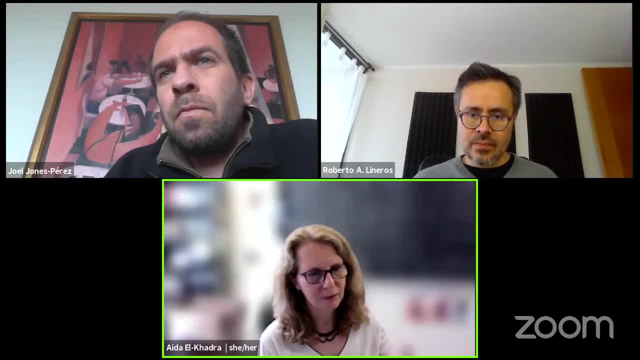 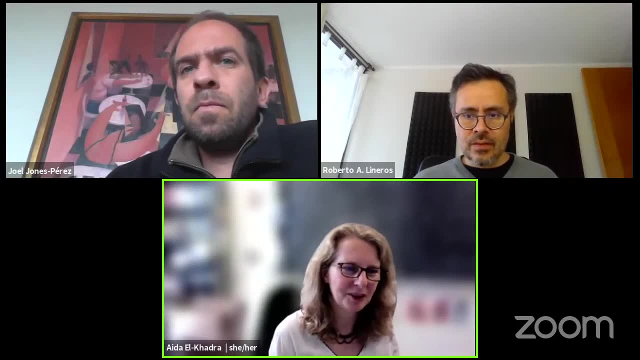 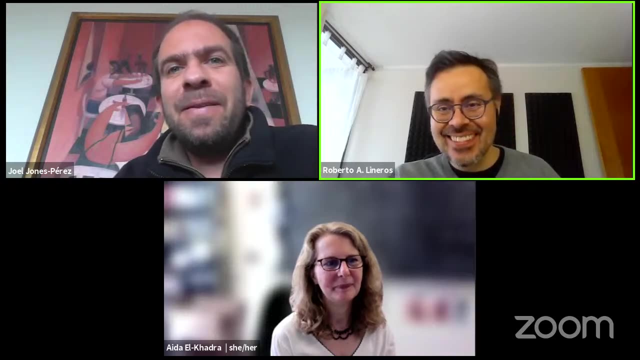 precision. It's not new methods, It's just refining our existing methods to address the precision needs. I would say Again: that becomes computationally also expensive in the end. Thank you, Okay, You okay, Roberto. Yeah, I was just thinking. 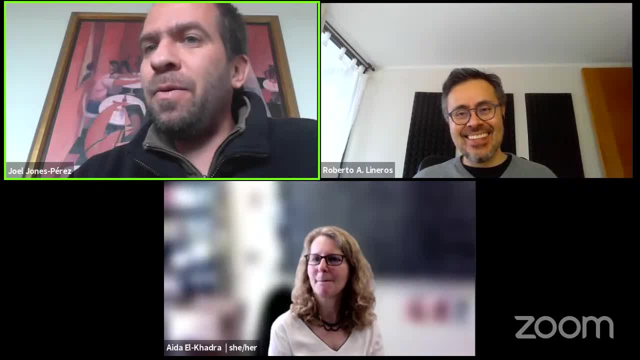 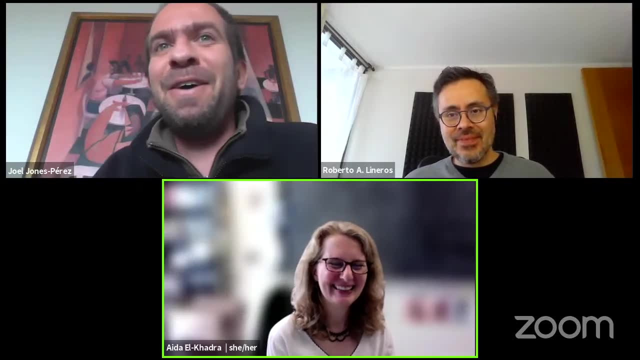 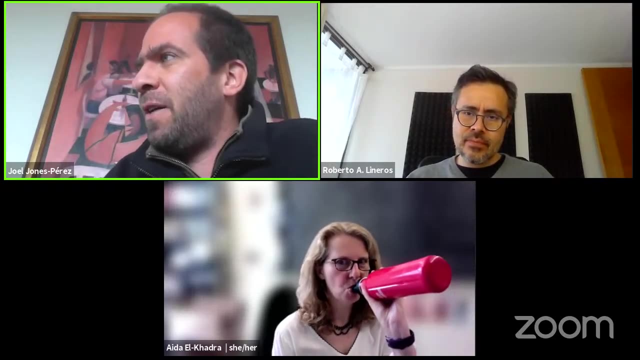 So I don't think there's anything else from YouTube. No, nothing else from YouTube. I'd like to ask one final question. Okay, We're running out of time, But I remember many years ago that when evaluating the, the hydronic vacuum polarization. 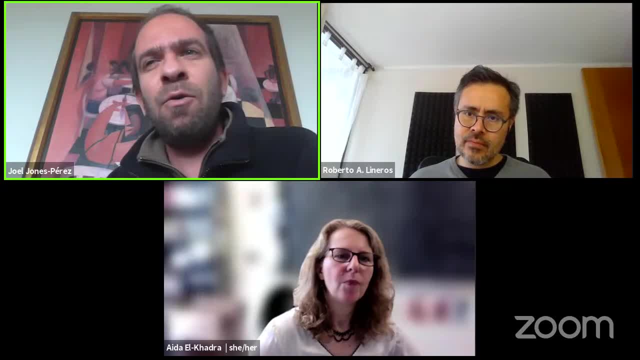 there was this tension between data coming from electrons and taus. Is this why you refer? No, no, Very good, yes, So I've, I've, I'm going back to the question: I, I've, I've, I've, I've, I've, I've, I've, have you know, I, I've, I, I, I, um, I, I, I, I have a question of: is there any kind of reaction to the process of what you average and relative? 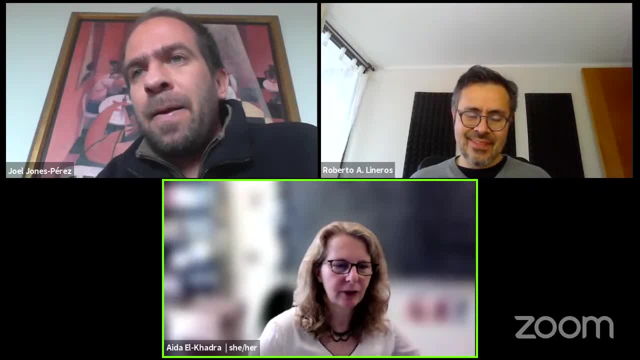 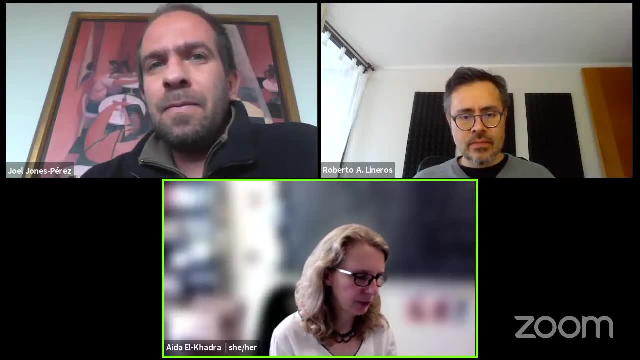 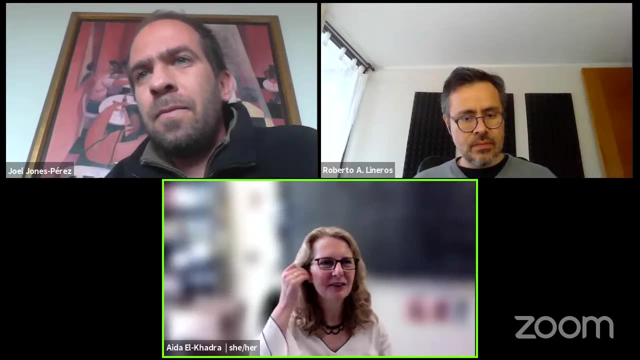 No, no, Very good, Yes, So I've. I've completely glossed over that, And so there was a tension, and some people are pointing out that the- if you take the old tau data that they are, you know, agree with the BMW, collaborations resolved, et cetera. 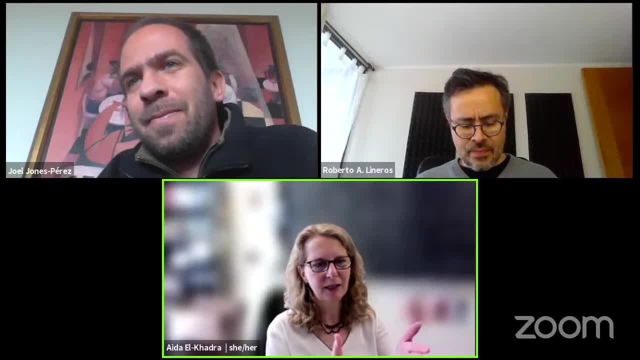 When you use tau decay data right, The tau lepton decays by a virtual W boson, you know. and and then the virtual W boson will will decay into the hadrons, pi, ions, et cetera, You know. 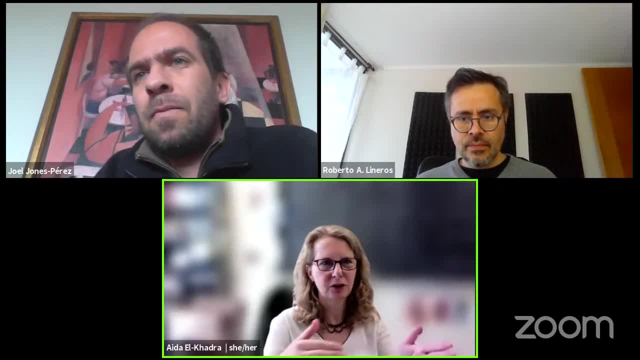 so you might have, you know, tau plus by virtual W boson decays into pi plus pi zero, say, and pi plus pi zero, pi zero, pi plus, pi minus pi plus, et cetera. So the final state of course is charged, because it goes by a charged W. 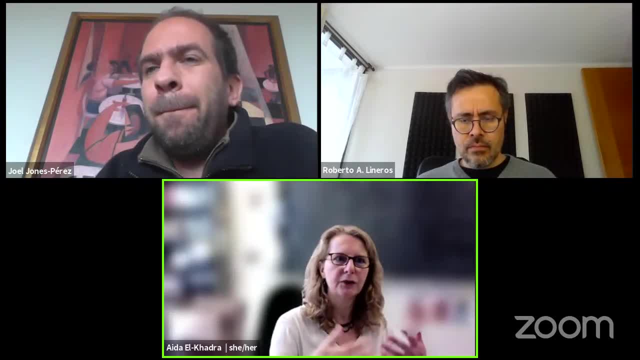 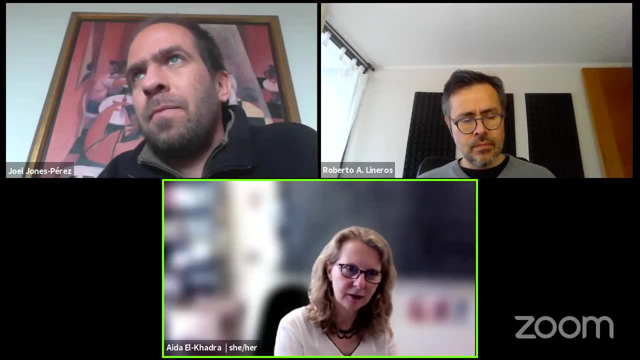 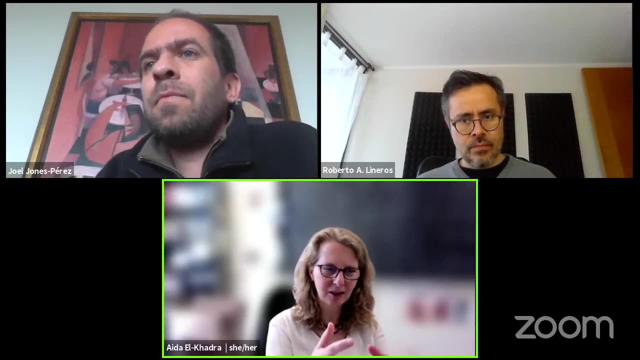 boson, Because you start with a tau lepton, whereas for E plus, E minus data you're directly measuring the photons, vacuum polarization. You have a photon connecting to a dronic vacuum bubble. The cross section is E plus, E minus goes to pi plus, pi minus. 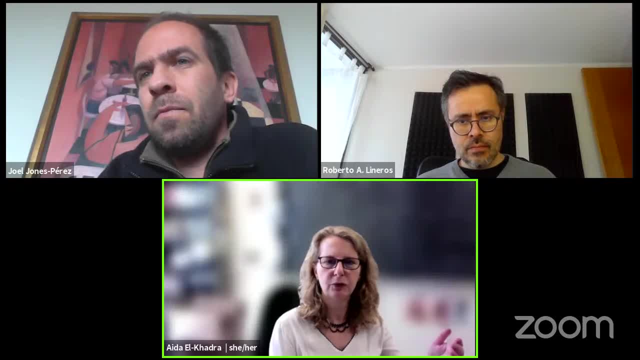 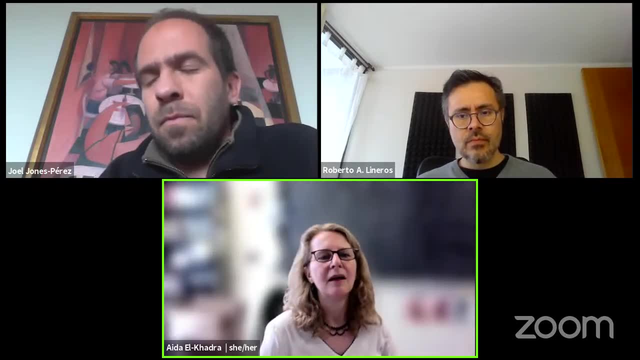 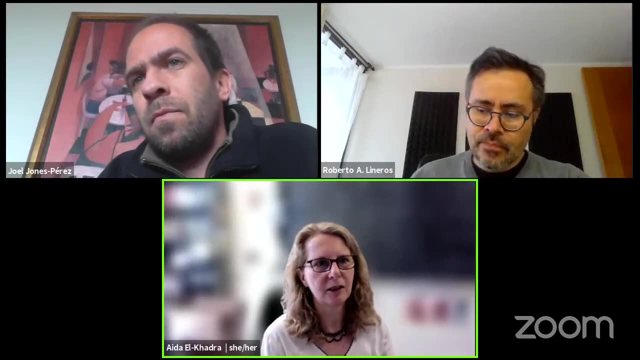 So it's electrically neutral. So you have to account for the isospin rotation going from basically the photon to the W boson. And now, at these scales this is not something I mean you can estimate it phenomenologically. 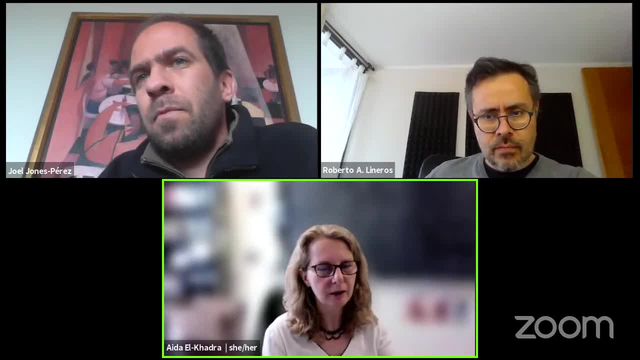 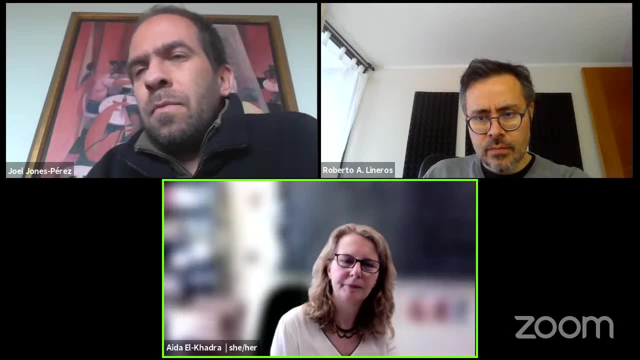 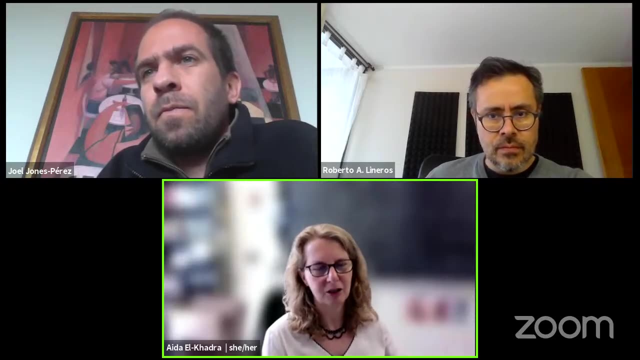 but there are errors associated with that. If you include those errors and if you do this, then basically: first of all, the tau data now are less precise because we have much better E plus, E minus data. You include this correction, they weigh in much less. 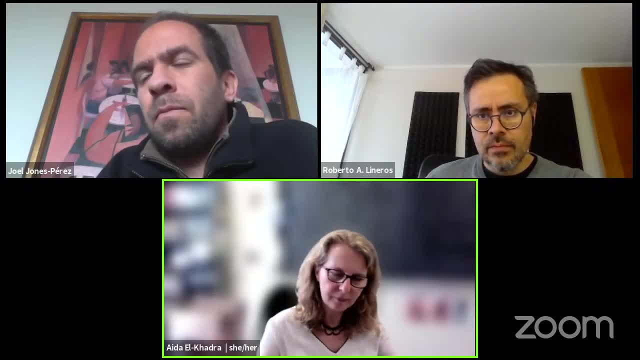 You know, you have, you have an uncertainty, you have an uncertainty from that, And then you know. and then how well do you know, you know, how well have you estimated the uncertainty? Because this is also, again, a non-perturbative problem. 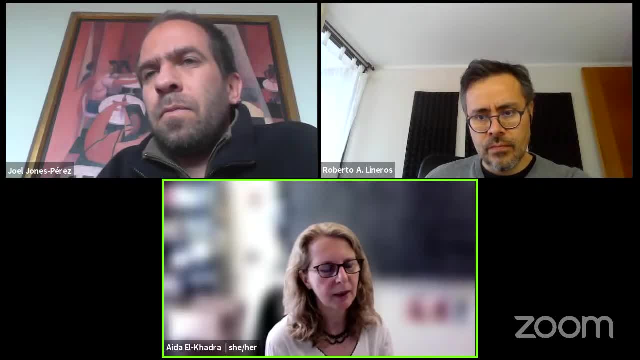 You know people have tried to work on this and the conclusion has been that the tau data are just not that useful. but there are ideas for lattice calculation of this isospin correction Once you have something that you have calculated, that if you can calculate. 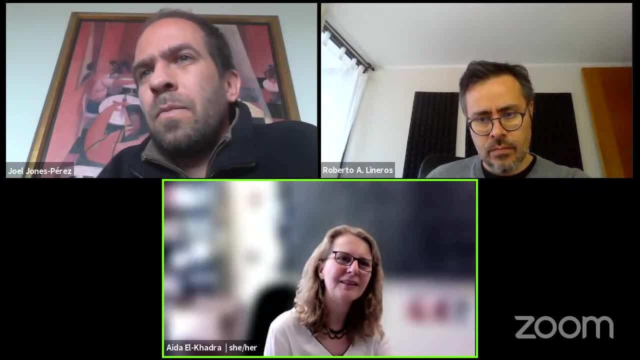 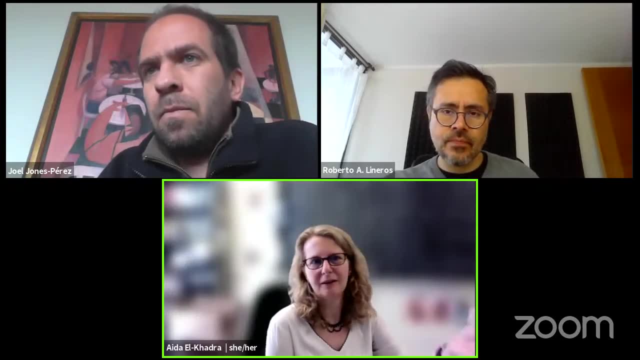 the isospin correction, again non-perturbatively, with quantified errors. then you can use the tau data And if we have, say, a tau charm factory, well, I think we have a tau charm factory also, you know.